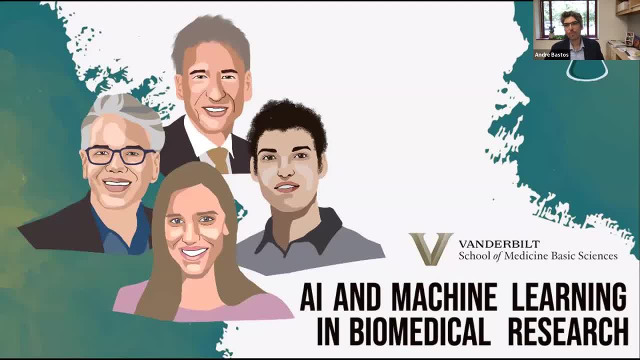 Thank you all. okay, we're at 100 participants, six. the number's still going up, but i i think we should probably begin to get started, which is just a housekeeping um thing. so if you have questions, um, if you would please put them into the q a at the bottom of your screen, uh, on the little icon there, um, and then um, we can. 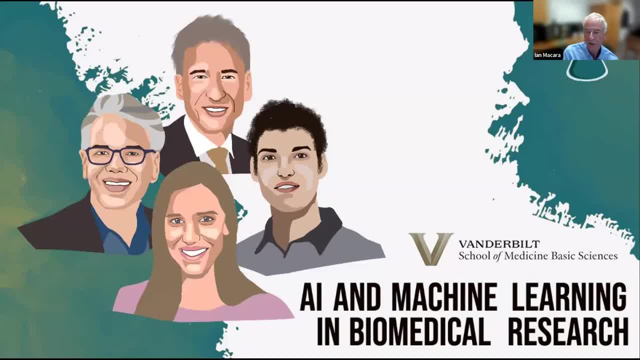 hopefully have time at the end of this panel session to discuss them. we already have a number of questions um that were submitted at risk registration and we'll try and answer as many as we can, but we might not be able to get to all of them. okay, so to begin, my name is ian macara and i'm going to be the moderator of this session. 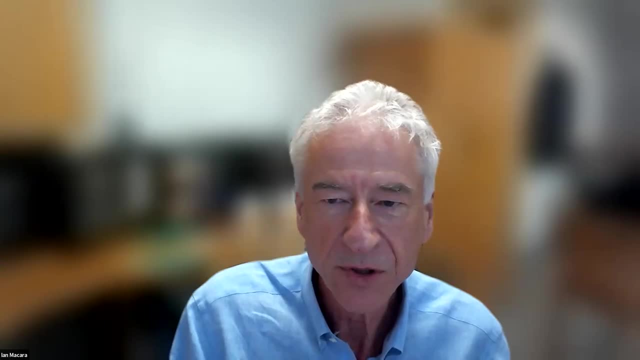 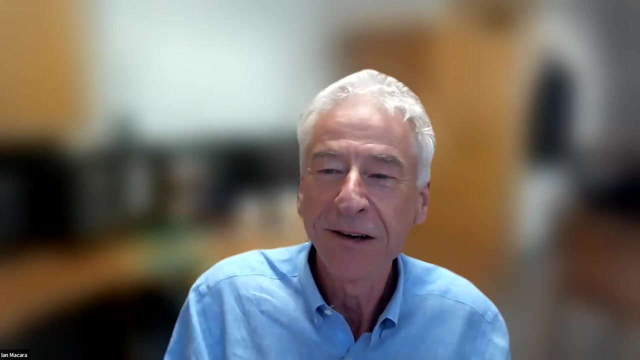 and by way of introduction, i'm the chair of the department of cell and developmental biology in vanderbilt school of medicine. my laboratory studies how cells self-organize into tissues and organs that comprise our bodies and how this organization is disrupted in cancer. so i confess i'm not an expert in ai and deep learning, but these tools now play vital roles. 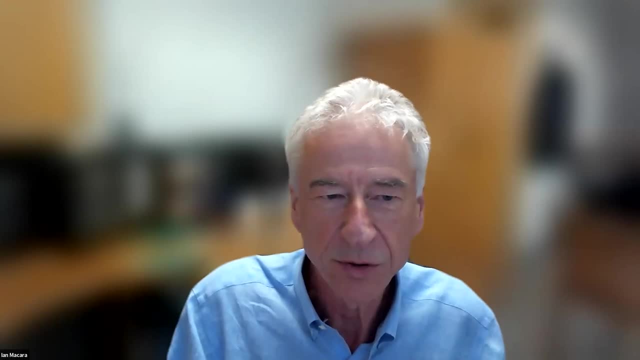 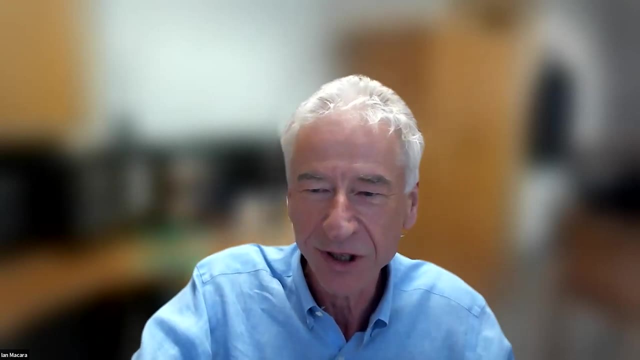 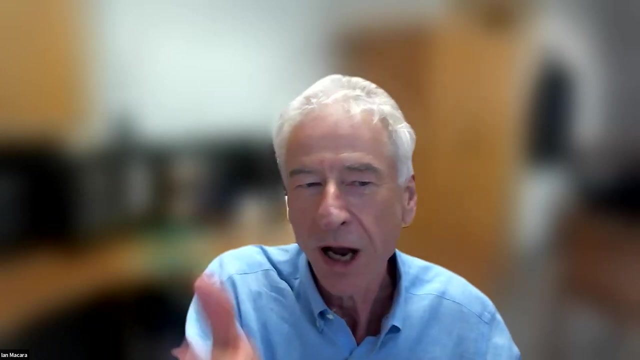 in many aspects of my research, and my laboratory uses them almost daily in one form or another. however, we do have a panel here of experts in artificial intelligence, and i'm going to now ask each of them to briefly introduce themselves, uh, before we begin the discussion. so, andre, why? 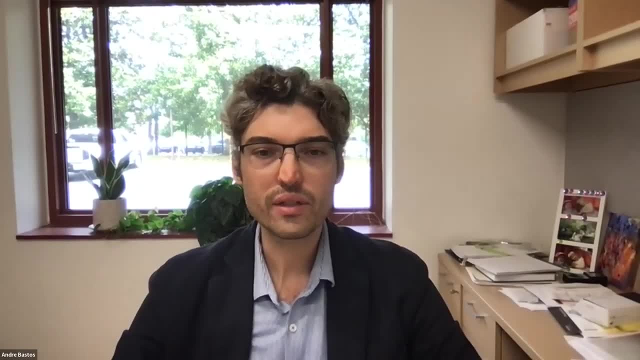 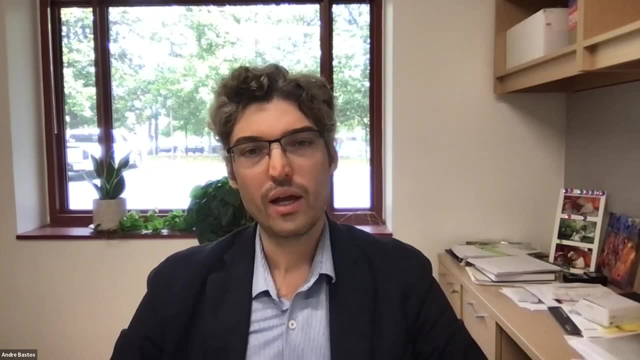 don't we start with you? hi everyone, nice to meet you all. thanks for attending. my name is andre bastos. i'm a assistant professor at the university of england. at the university of england, i'm an assistant professor here at vanderbilt. i've arrived only about a year ago. i'm starting up. 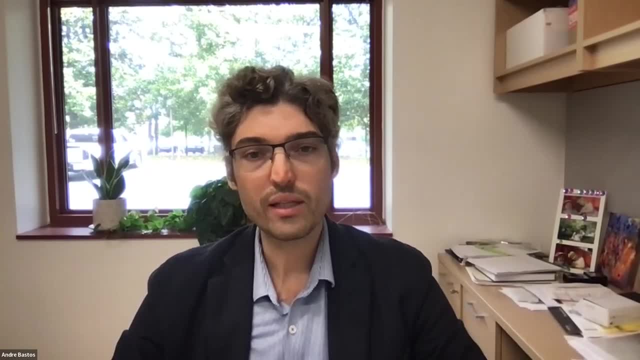 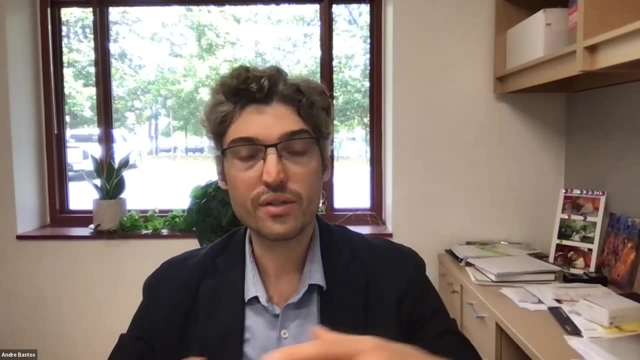 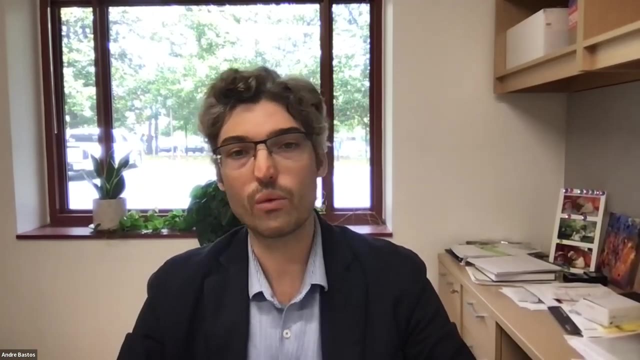 my lab here, and the purpose of my lab, or the goal of my lab, is to understand cognition at a single neuron level and also to understand how networks of neurons interact in the brain as, for example, we are perceiving something, or when we're remembering something, or when we're deciding. 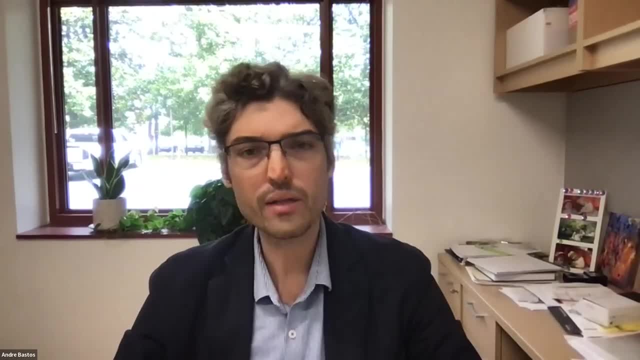 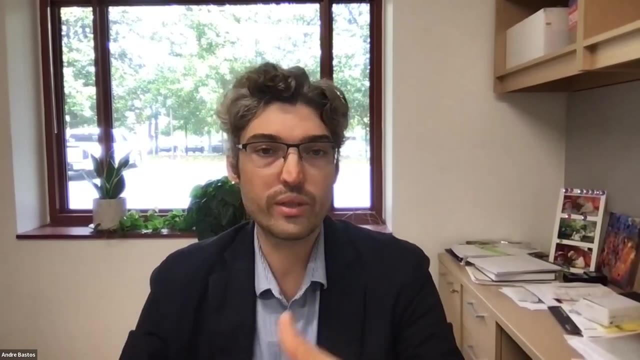 whether or not to pay attention to something. and in order to- in order to answer this research question- we train non-human primates, monkeys, on tasks, and that enables us to then have almost human level- uh, style behaviors that we can study all the way down at the neural level. so we're trying. 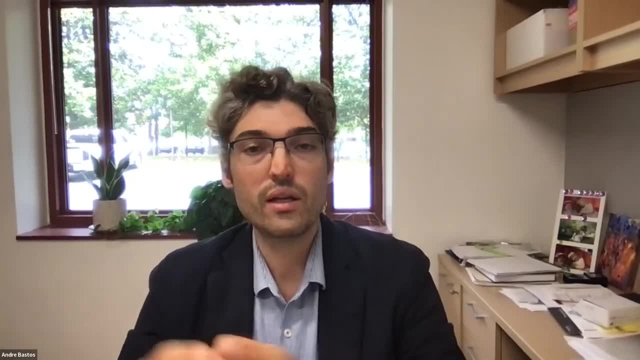 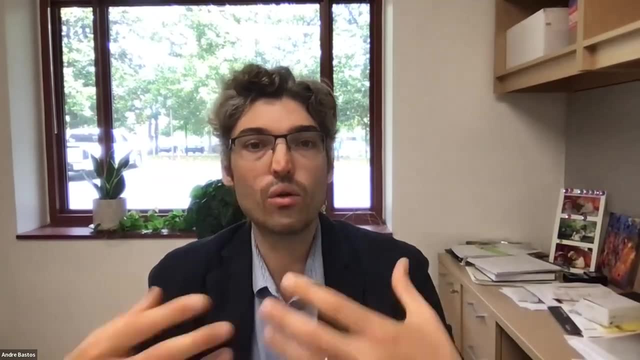 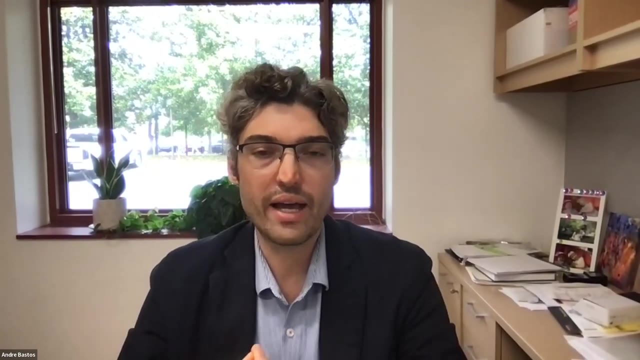 to really span a whole host of different neurobiological organizational levels, from the single neuron to networks of neurons, to brain regions and then ultimately, to behavior, and we're trying to understand that and, needless to say, the data sets that we're collecting on that end are getting more and more complex and as they scale up and get more and more complex, 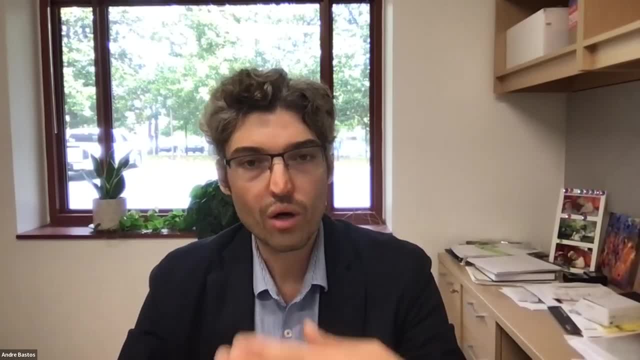 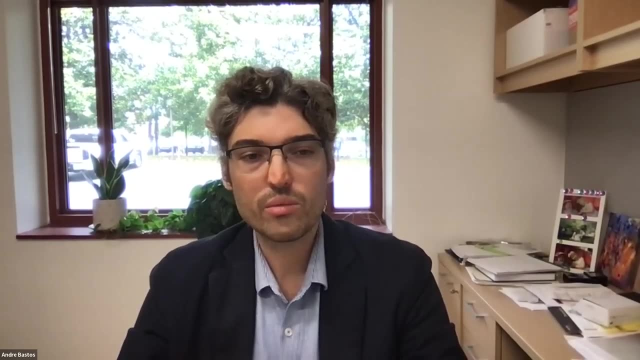 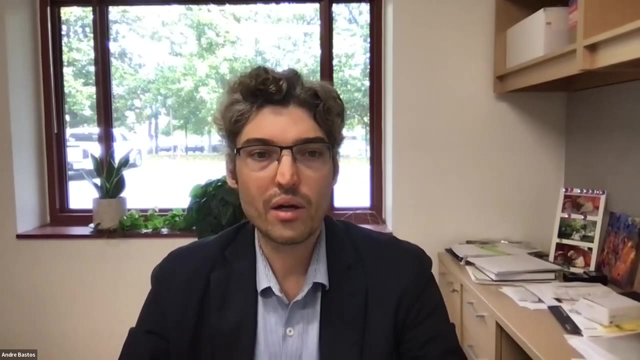 we've been increasingly using and borrowing tools and expanding on tools from machine learning and artificial intelligence to understand that data and ultimately also we want to create better models of the brain. so we're also going to test whether or not some ai models are good models for. 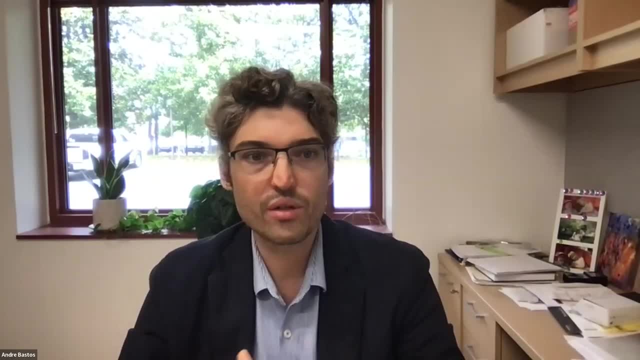 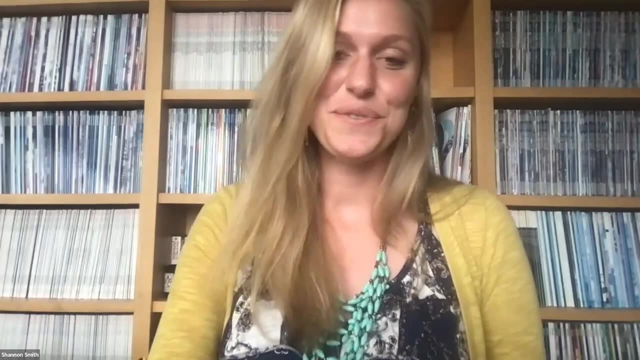 what's happening in the brain itself as these types of computations are performed. super, thank you so much for this very inspiring presentation and i'm going to hand it back over to you, shannon. yeah, well, thanks so much for that and i'm going to hand it back over to shannon. 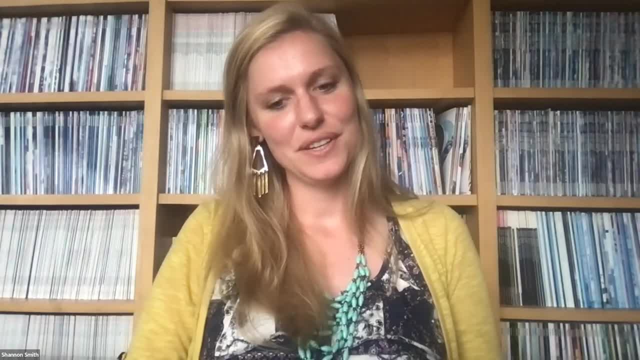 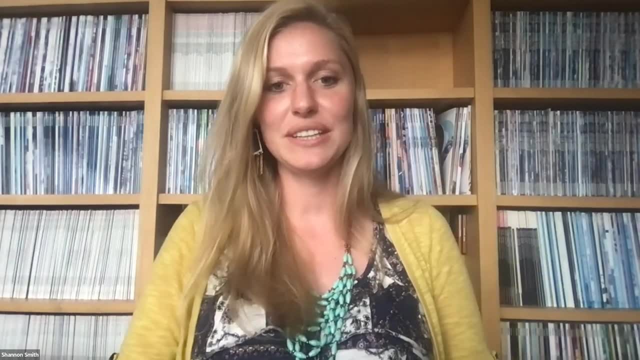 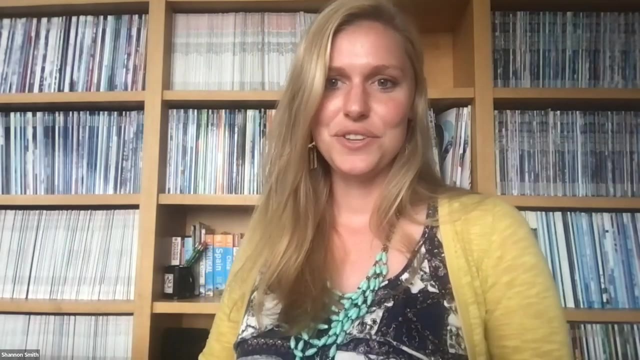 i'm going to hand it back over to you, shannon. so, shannon, you're doing very different type of research. yeah, so my name is shannon smith. i'm a graduate student here at vanderbilt in the lab of dr jones myler doing a lot of- uh, smaller, uh, biochemistry research. think, think, a lot smaller. 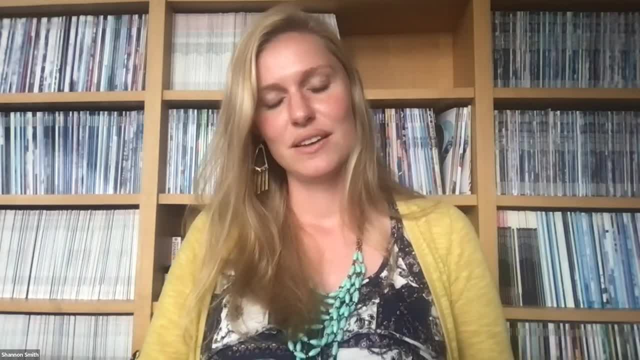 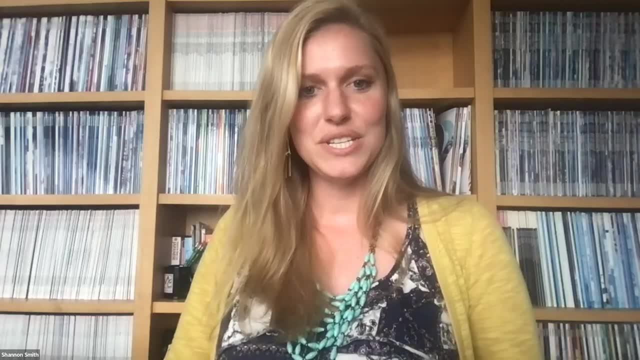 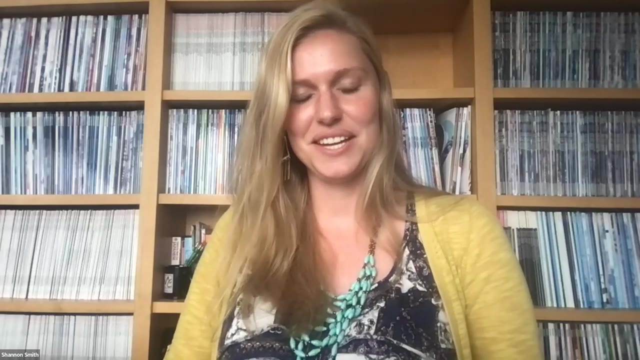 at the individual protein level, looking at their structures, using within the AI realm to help us with these tasks. So looking at individual proteins and their structure and their function and then going from there and designing a drug to hit that protein. That's kind of the realm that I work in. Thank you So, Jesse, you're our real expert on. 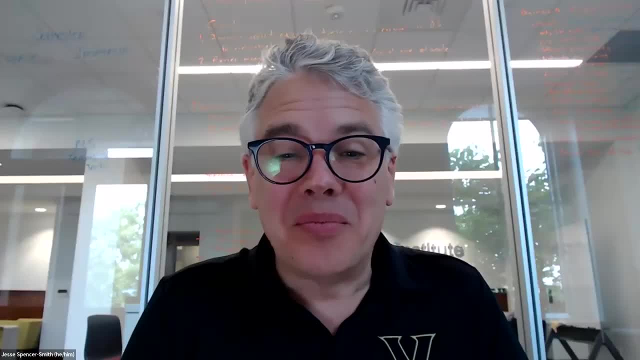 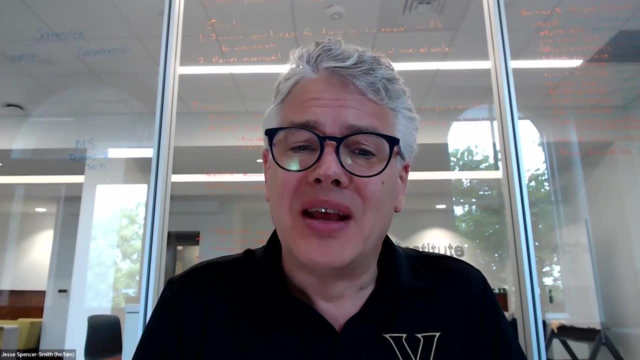 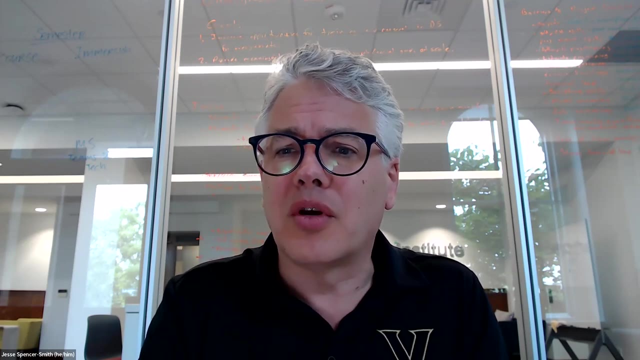 AI. Well, so I'm Jesse Spencer-Smith and I'm Chief Data Scientist at the Data Science Institute at Vanderbilt University. I'm a cognitive psychologist and cognitive scientist by training and I have academic and industry experience. Previously, at University of Illinois, Urbana-Champaign, I was an assistant professor in their quantitative psychology department. 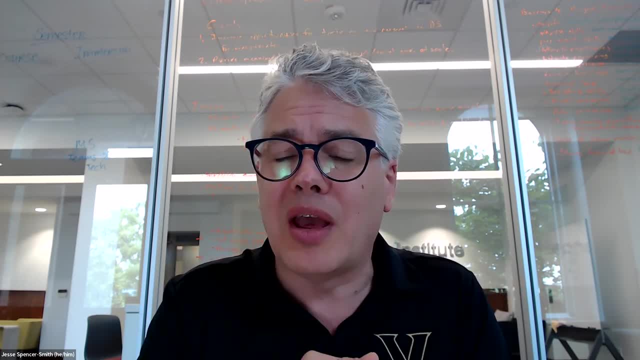 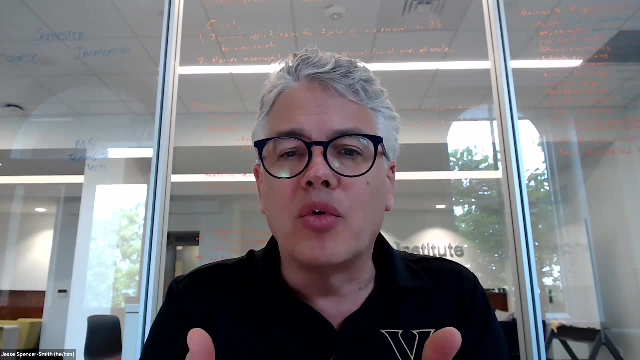 in industry. I founded the first data science team at HCA Healthcare, But here at Vanderbilt I lead a consulting data science team. We collaborate with researchers across the campus in applying data science to the data science field, And I'm a professor at Vanderbilt University. 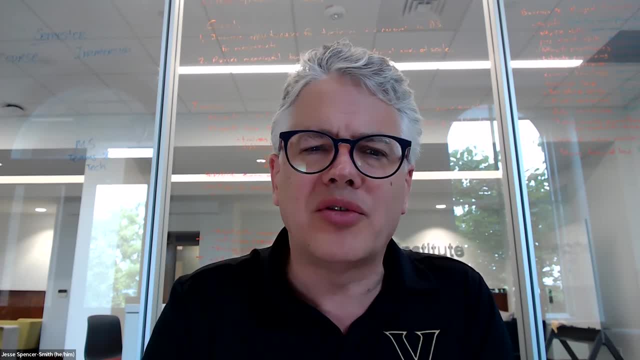 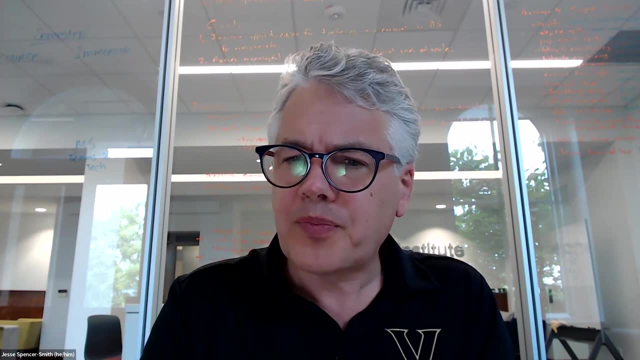 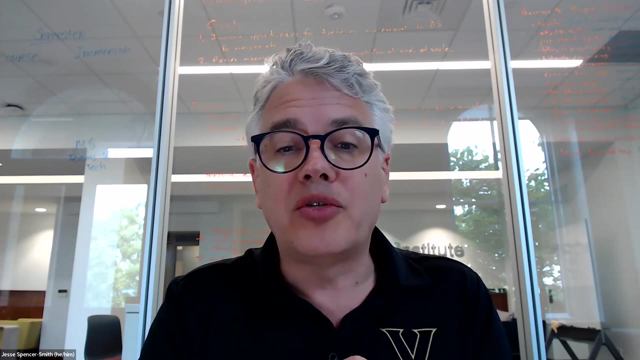 in the data science and AI to their areas of research, And we've had projects applying AI to areas from archaeology to education, to basic sciences. Also, note that we do offer free consultations, workshops, trainings, and I believe that we'll be sharing a link at the end of this. 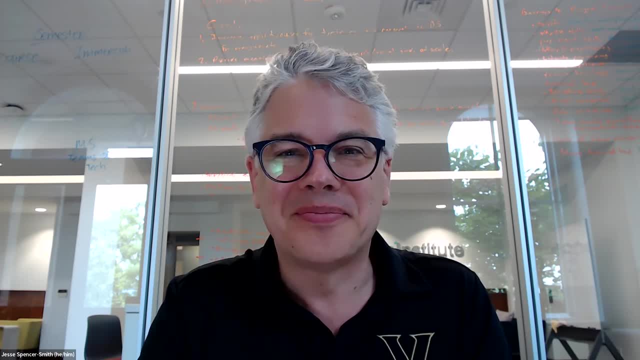 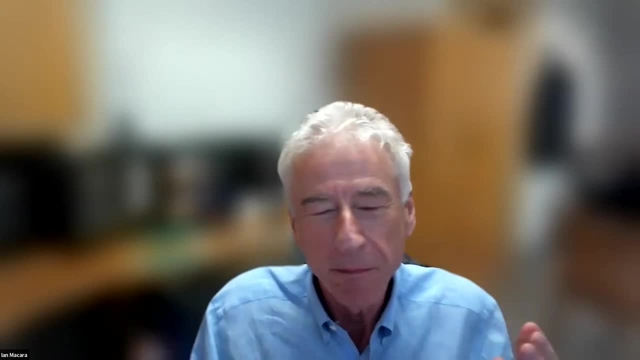 if you'd like to learn more about how to access those Great. Thank you very much. Okay, so let's begin, Just sort of introduction. So I'm Jesse Spencer-Smith and I'm the chief data scientist at Vanderbilt University, And I'm the chief data scientist at Vanderbilt University And 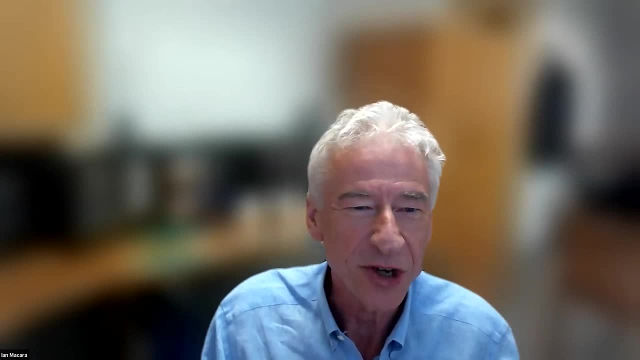 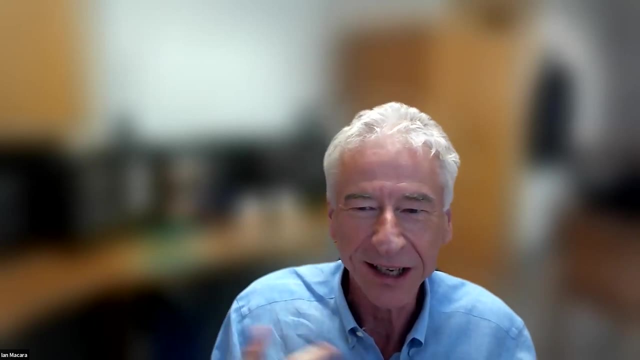 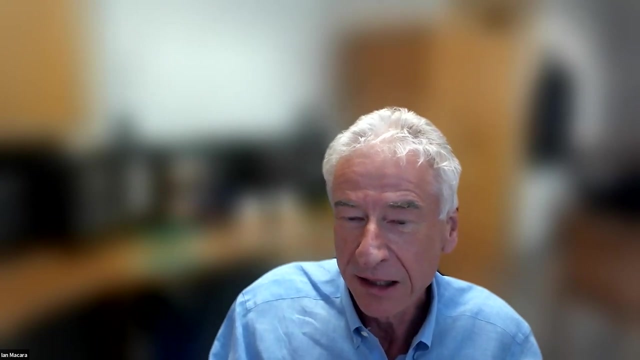 my impression is that, after decades of false starts and slow progress, AI is now advancing at a really breathtaking rate and, with no indication that it's slackening off or it's not going to continue, probably will continue to improve exponentially into the foreseeable future. And you know, I get the impression that it's transforming almost every field. 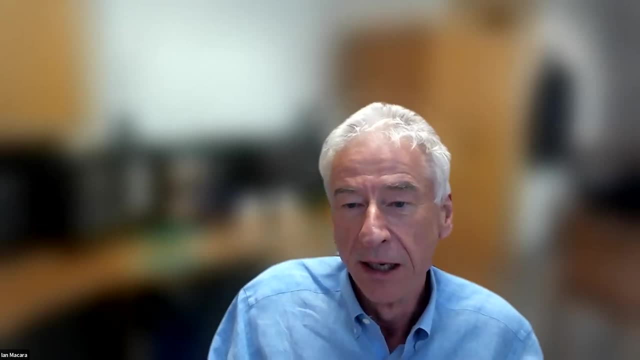 of human endeavor, including scientific research. But you know, I always wonder, well, what exactly is AI? What do we mean by intelligence? And you know, I think, you know, I think there's a lot to be said about it, But you know, I always wonder, well, what exactly is? 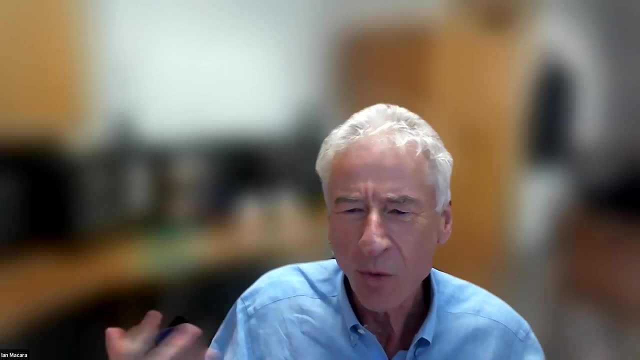 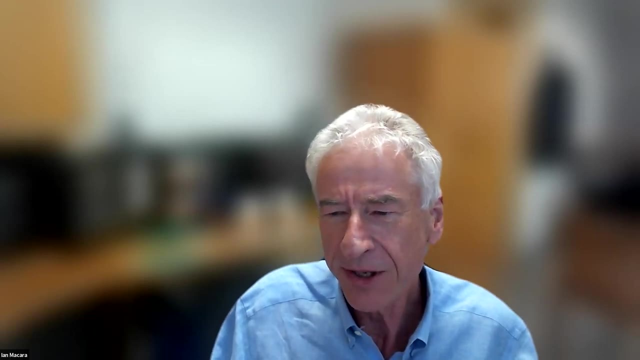 AI. What do we mean by intelligence anyway? Is it related to self-awareness, Or can machines be super intelligent without really being self-aware at all? How is we're going to talk about? how is AI impacting biomedical research specifically, how it's going to change. 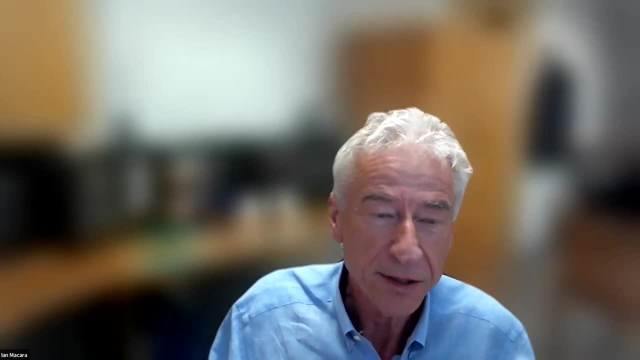 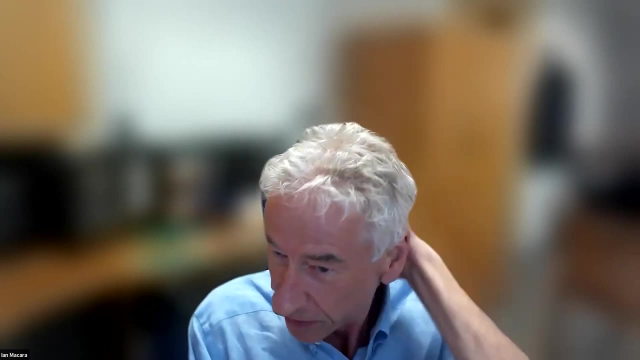 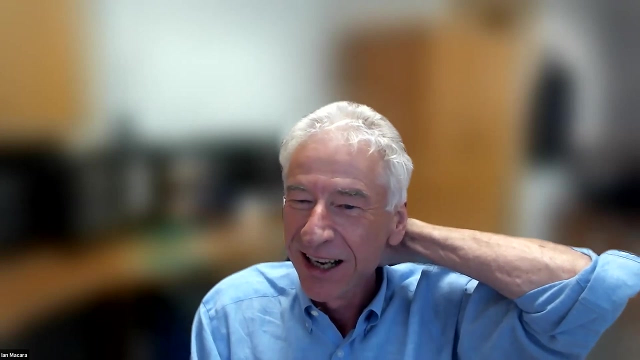 perhaps the way in which we do research and what ethical dilemmas are associated with using AI in general. So perhaps we could begin, maybe, with this fundamental question about what AI really is. So AI is intelligent. Artificial intelligence is intelligent, And how is it likely to evolve? 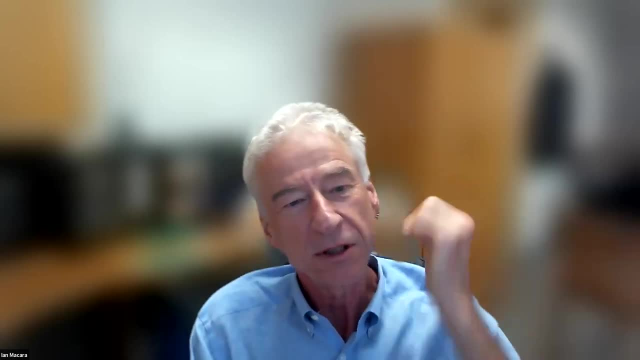 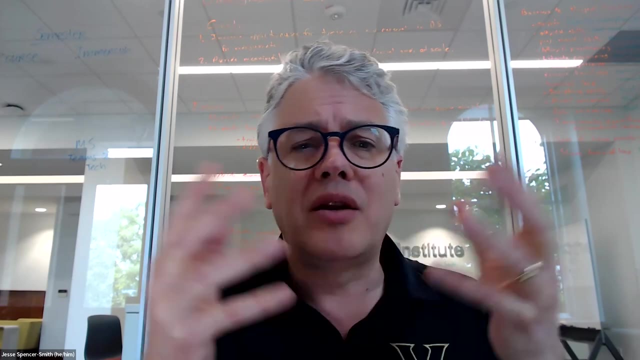 over the next few years. So, Jesse, maybe you could go first and then I'll ask André, Absolutely yeah. So artificial intelligence has certainly been a moving target. So you know, we've bandied the term around for you know, 50, almost 60 years and it's changed. 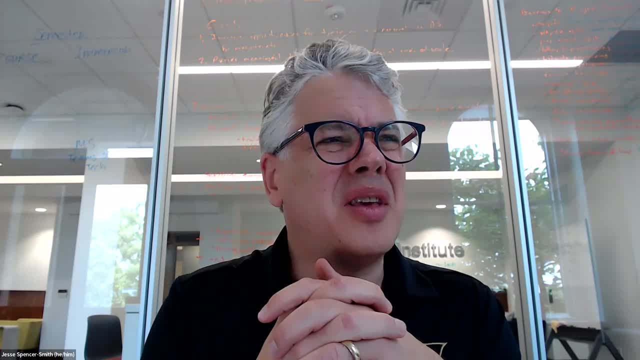 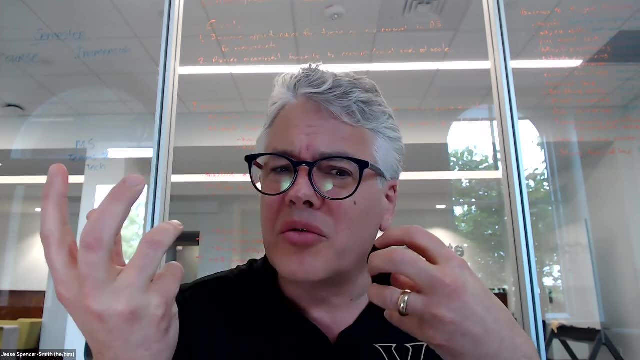 over time. I've worked in the area since about the late 80s, but I've never been comfortable saying that I worked in AI, Mm-hmm, That I work on memory or decision-making. Now I'm perfectly comfortable saying that. 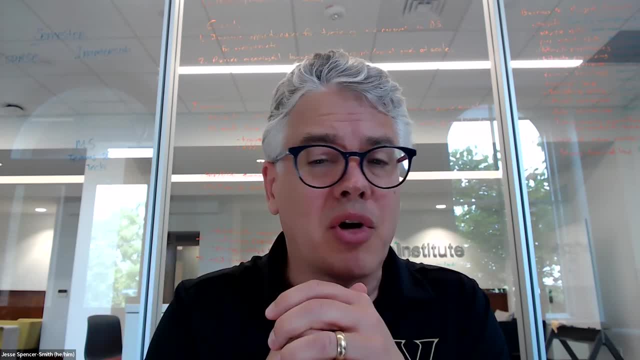 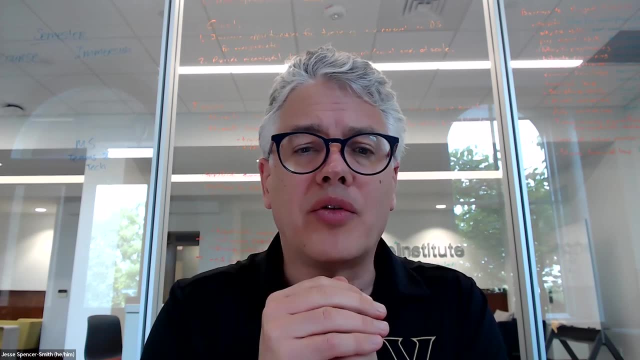 I'm working in AI because things have changed that much, really primarily in the last three years. So if you had asked me four years ago whether awareness and self-awareness was necessary to get these types of levels of performance that we're seeing, I would have said yes. 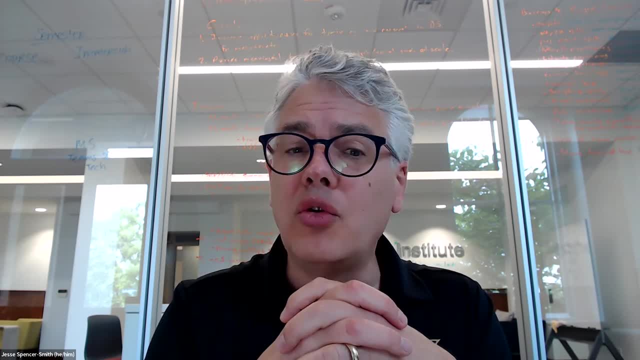 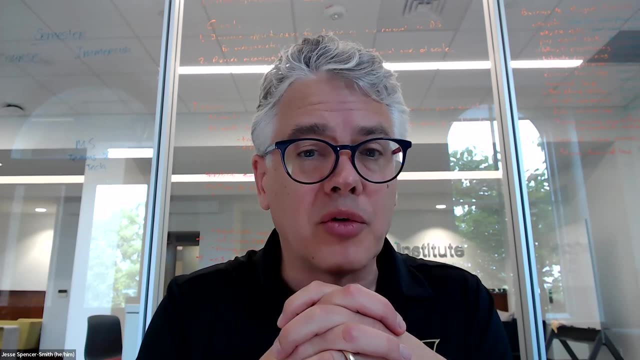 So don't count on it anytime soon. But then we had the advent of a new type of very powerful learning system. I mean, still today we're developing a deep learning network called transformers. That, combined with the additional compute that we have now combined with an idea that's 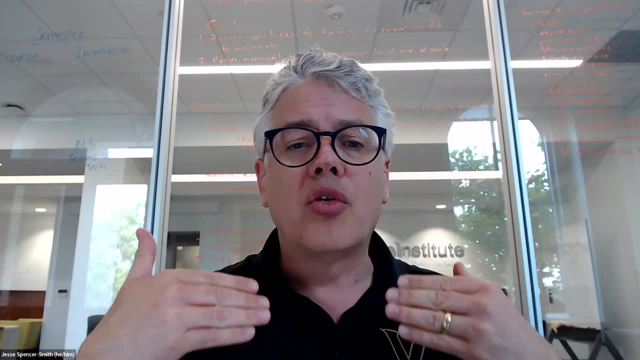 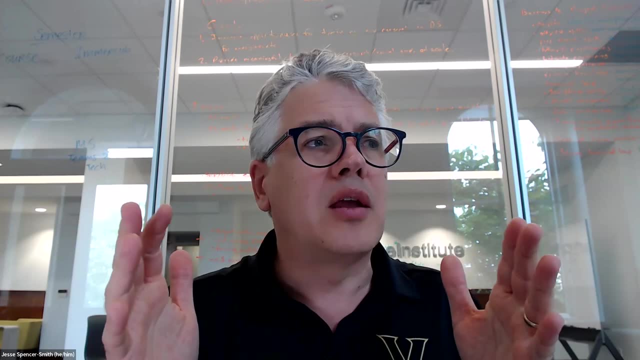 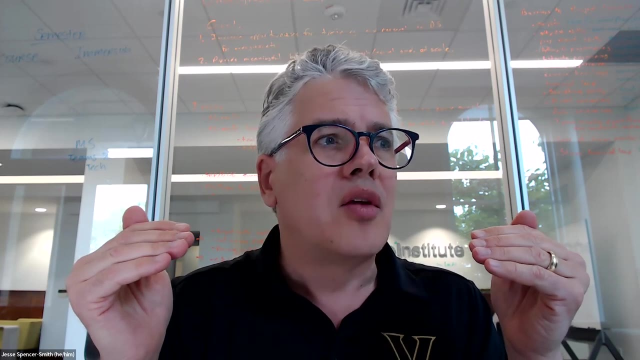 called self-supervised learning allows these machines to learn on unstructured data. They can learn languages from being exposed to large corpuses of text. They can learn language by being exposed to large corpuses of audio of spoken language. You can learn language. 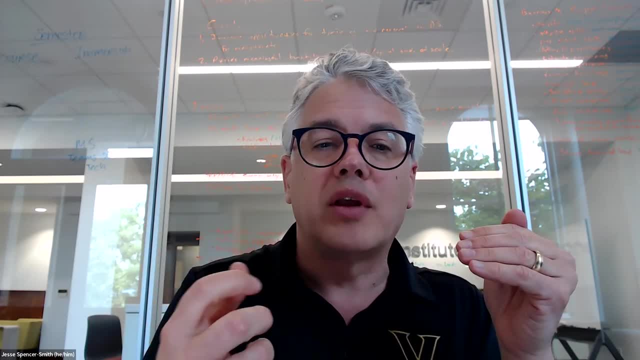 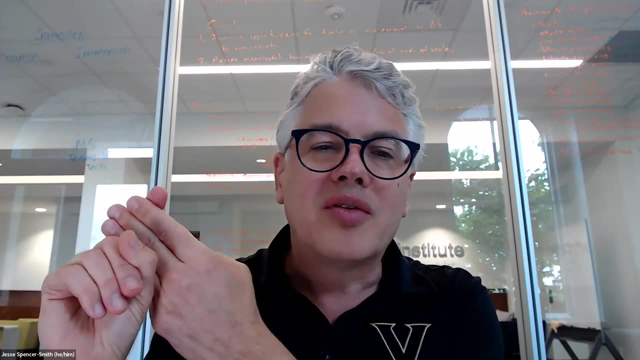 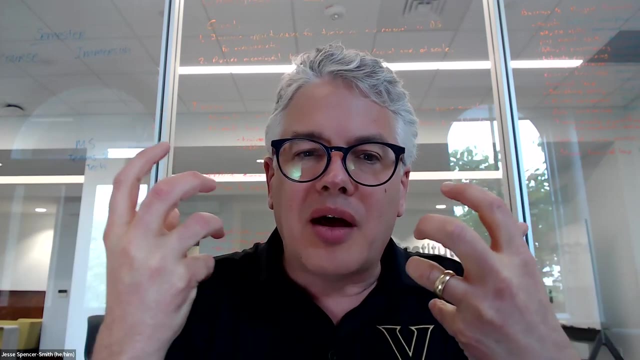 from that- Yeah, symbols- over time, So they can learn whatever language you would like them to learn. If you show them proteins, they can learn the language of proteins. If you show them the language of readings from astronomical observations, they can learn about anything that you would care for them. 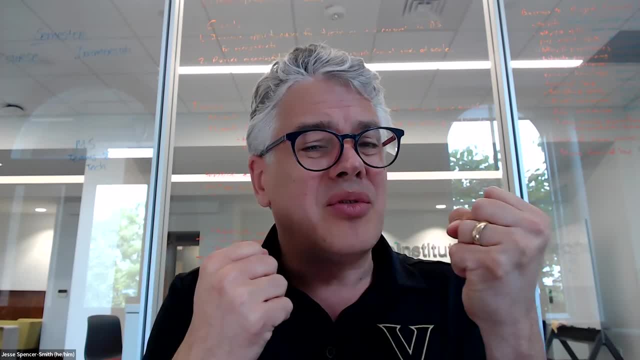 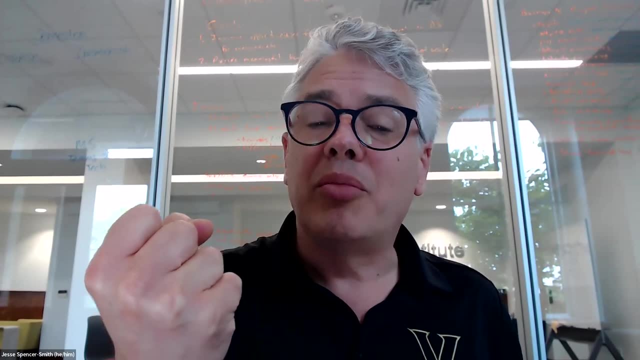 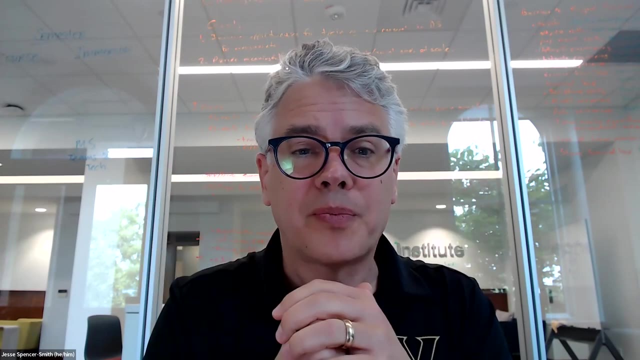 to learn, And the big change has been: we don't have to have labeled data. now They can learn from unstructured learn in a different way than we learned, but learn in the sense of just being exposed and doing self-supervised learning, And this is not self-awareness. 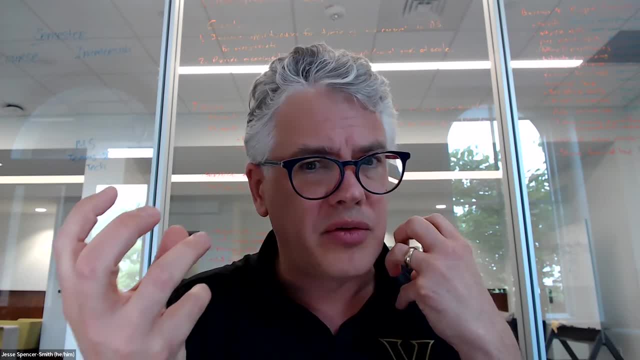 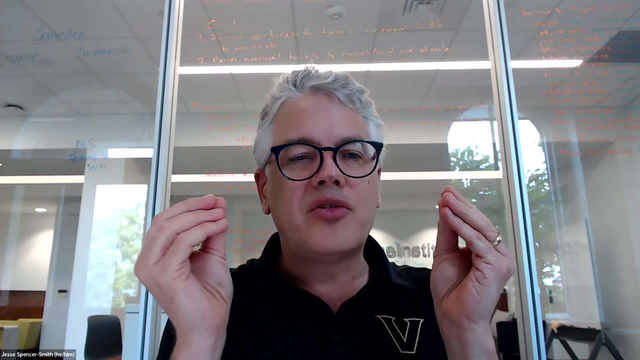 I think of these large language models that are driving a lot of this development as representing a crystalline knowledge. It's knowledge that you can use. you can ask it to reason, you can ask it to solve problems, but there is no self-awareness there Instead. 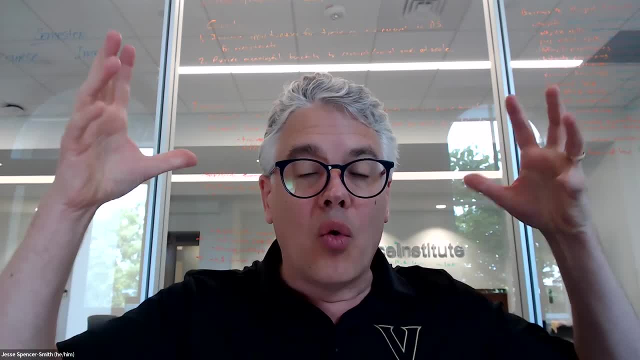 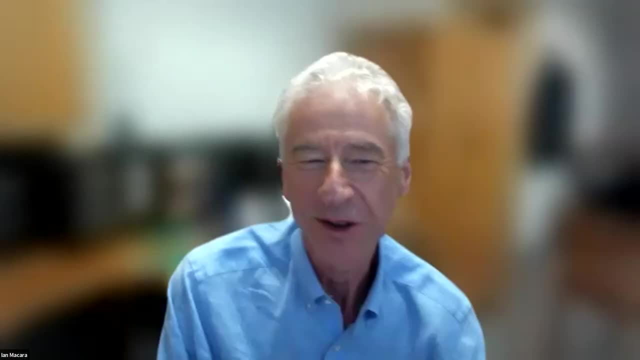 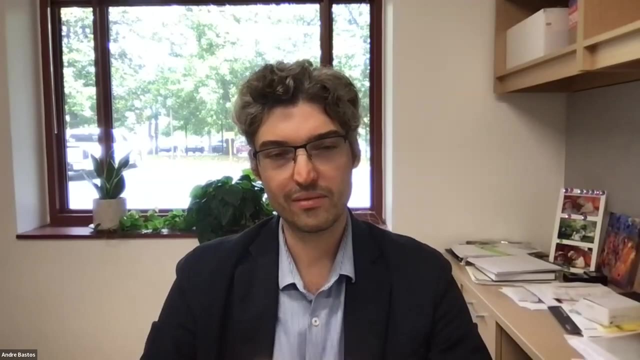 it is a highly capable collection of well-organized information that you can draw on to solve problems. It augments Great. Thank you, That's really interesting. So, Andre, I mean you work in cognition, so I'd be very interested in how you perceive this. you know, when we talk about artificial. 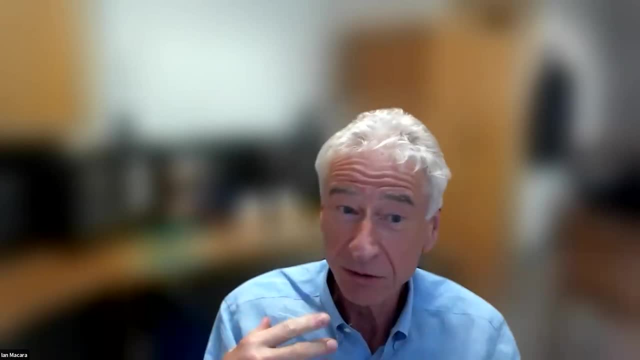 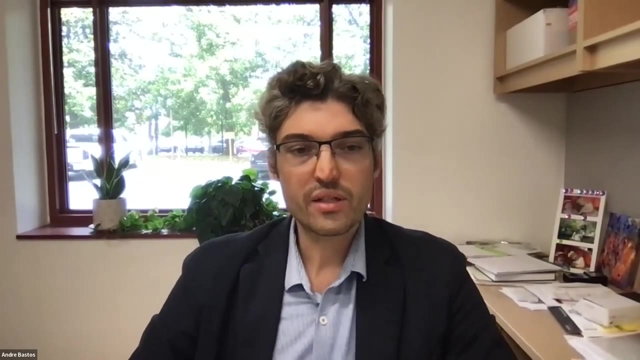 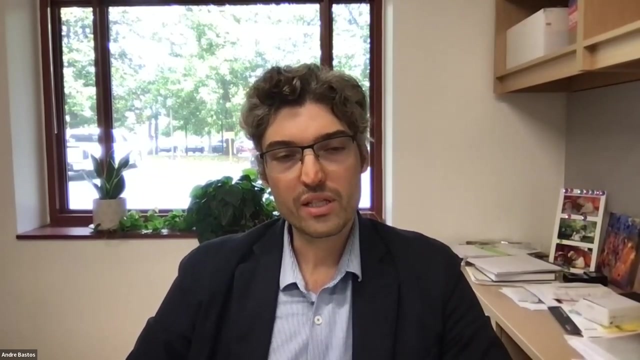 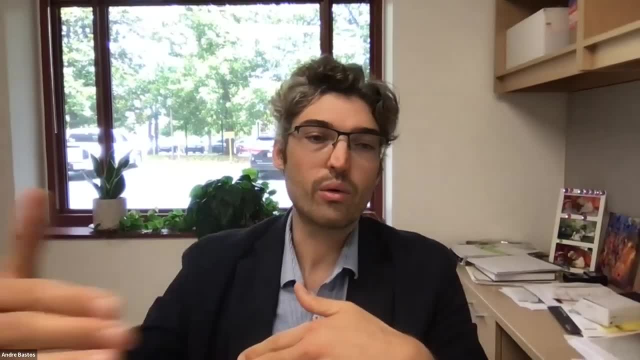 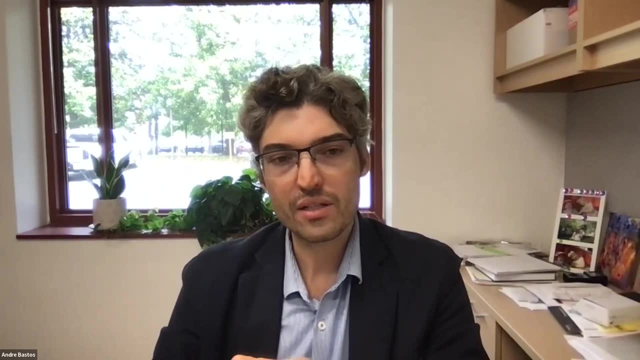 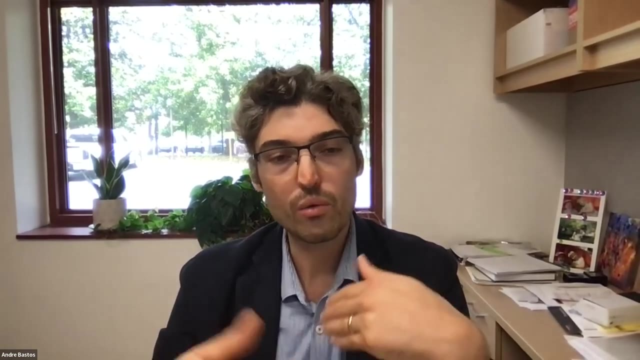 the deep learning network. it has been shown that that deep learning network can perform in a very human-like way on tasks such as image recognition, And these tasks involve, for example, identifying faces, identifying objects. things like that have been very well validated And 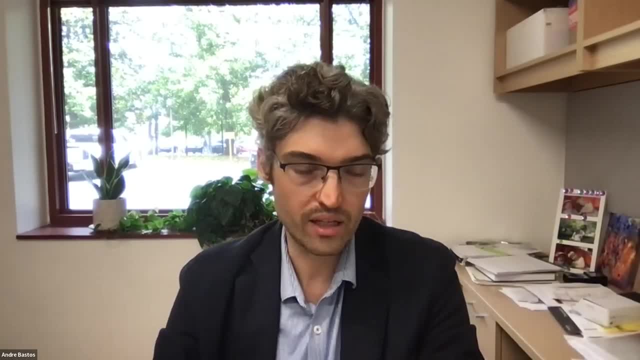 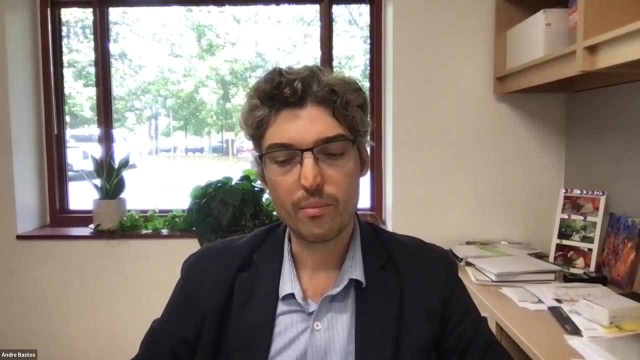 the performance of those networks, while not exactly the same as human level and primate like performance, does approximate it fairly, fairly well. But then the question is for me, as a neurobiologist and a neuroscientist, is why? 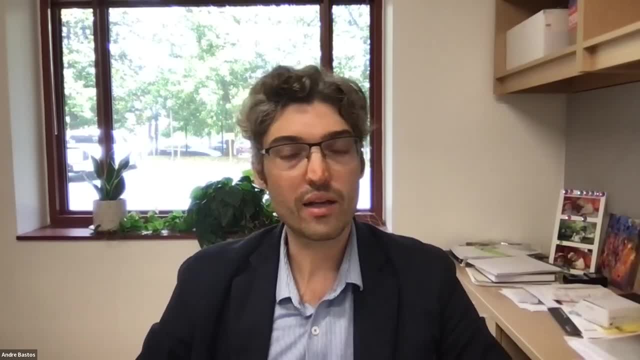 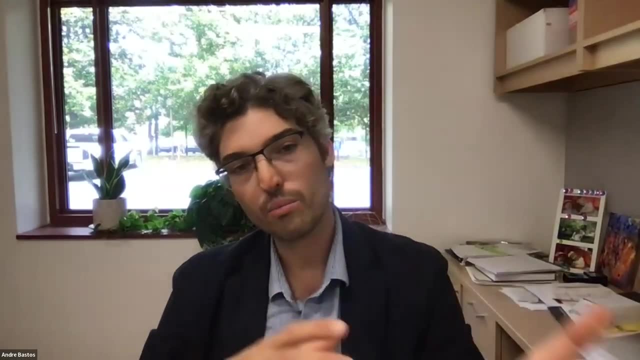 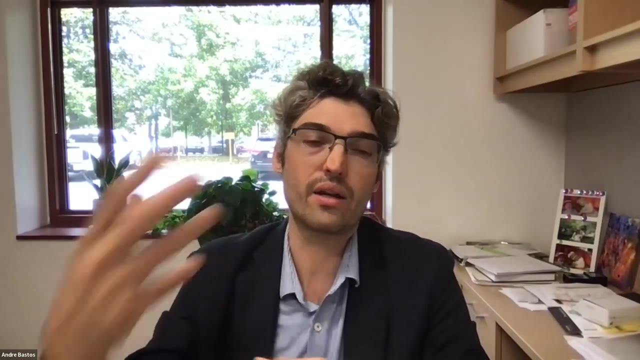 Why is it that it approaches that level? And for that you need to go inside of those models and to understand what those models are doing and how an input which is like, just say, a bunch of pixels, is then being transformed into this high-level output, which is the categorization. 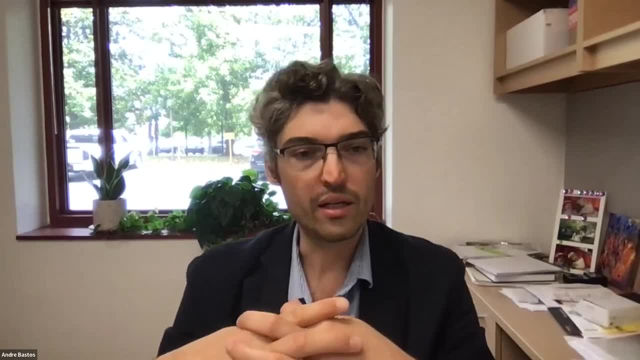 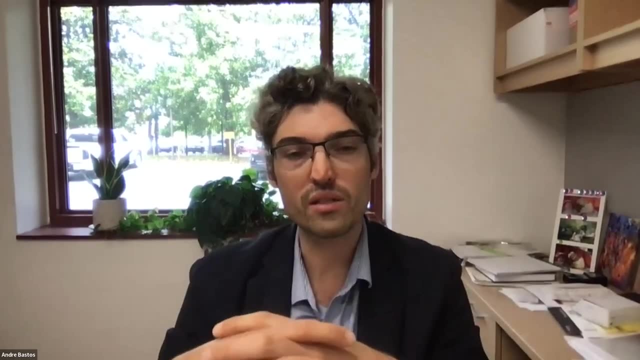 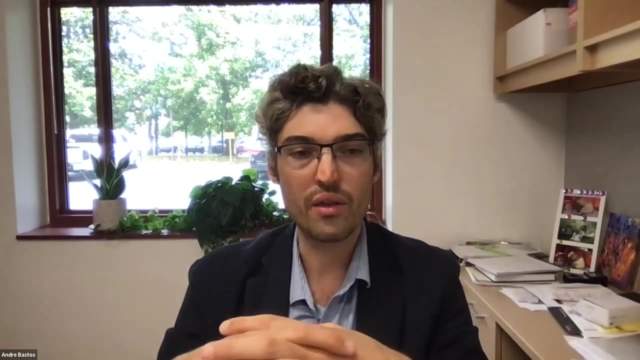 This is a face, This is a house, This is a car And in order to understand that transformation, we almost have to open up these AI tools and study them, almost as if we study a brain. And that process is also happening, but we are much less along on that. 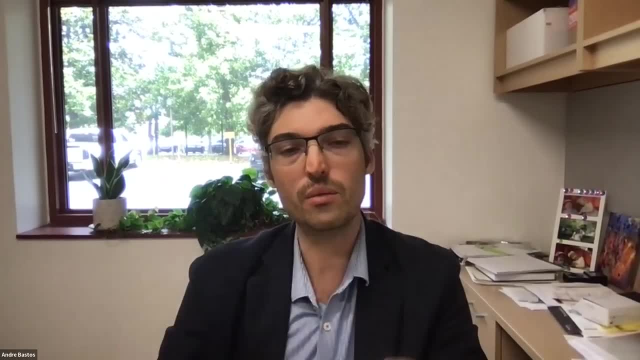 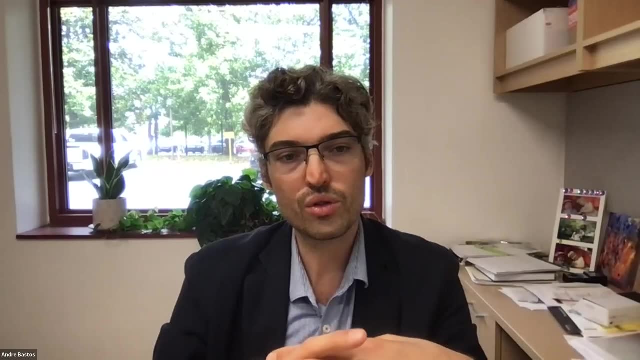 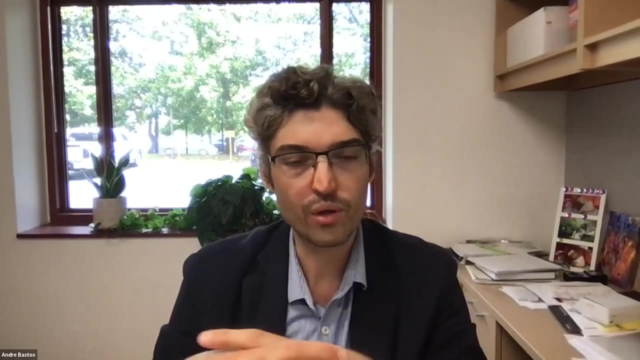 And that limits a little bit our ability to extract deep mechanistic neurobiological insights from taking only a machine learning approach. So the most, I think, promising work is going to be to combine the so-called wet lab approach and the dry lab approach. 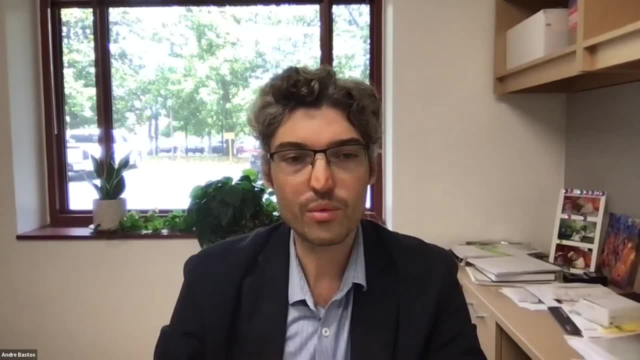 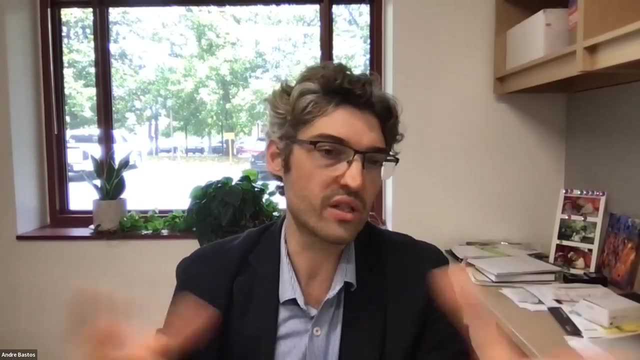 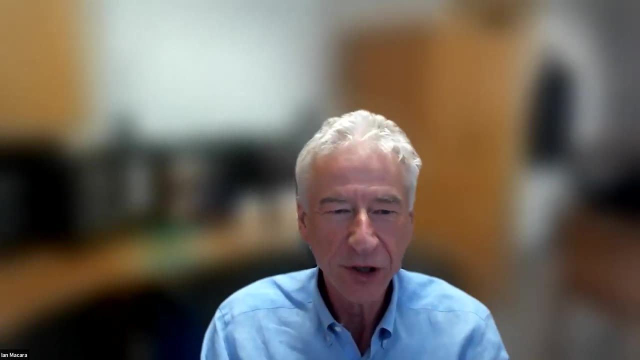 And that's something that we are hoping to pioneer in my lab- a so-called amphibious approach where we're taking both sides on the question of intelligence and the question of, for example, how memory works. So you think that studying deep learning and artificial intelligence could ultimately provide 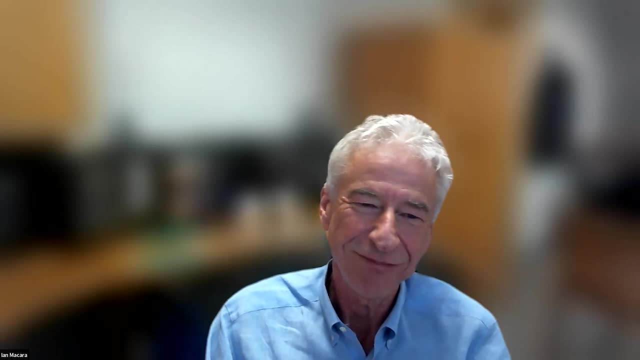 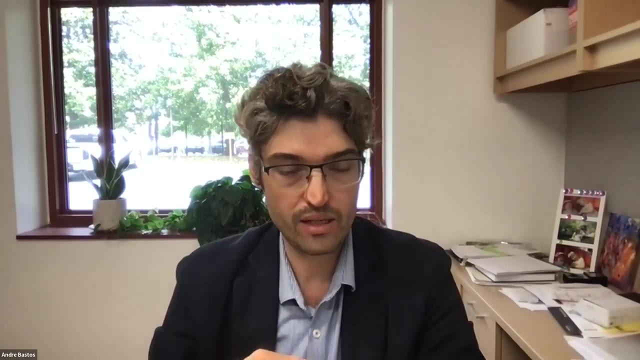 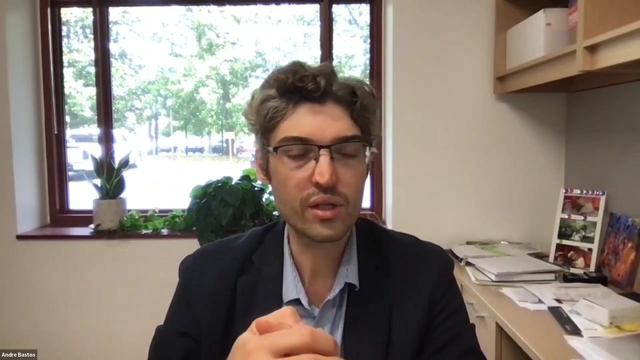 insights into how the human brain thinks: Yes, Yes And of course And of course. it could also provide insights onto how it does not perform those tasks, And so what some people are doing is comparing the internal representations inside of those AI tools to actual neurons that we can record in a number of different ways using a number. 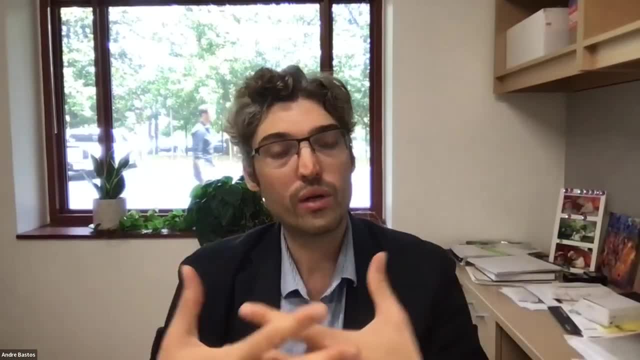 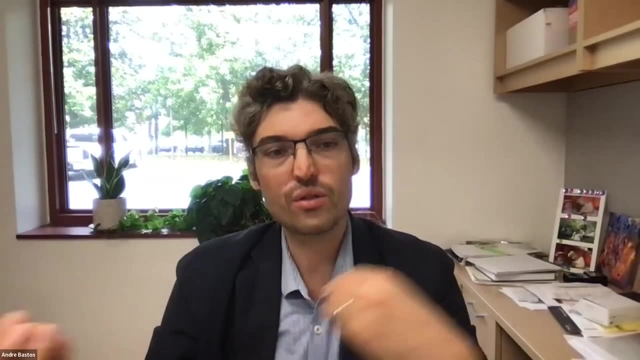 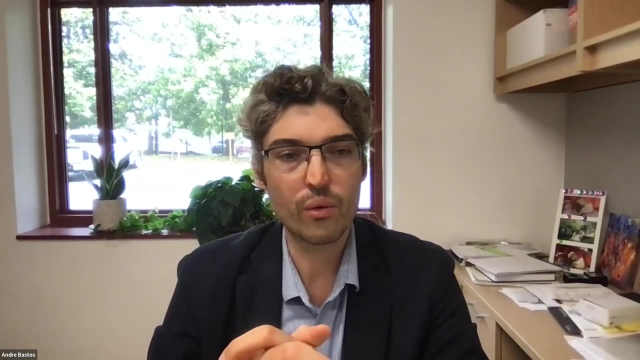 of different techniques, And then you can actually see how representationally similar or representationally dissimilar the brain is to actual neurons, Artificial neurons in an artificial neural network or a deep learning neural network, And then you can test different instantiations of those machine learning networks which 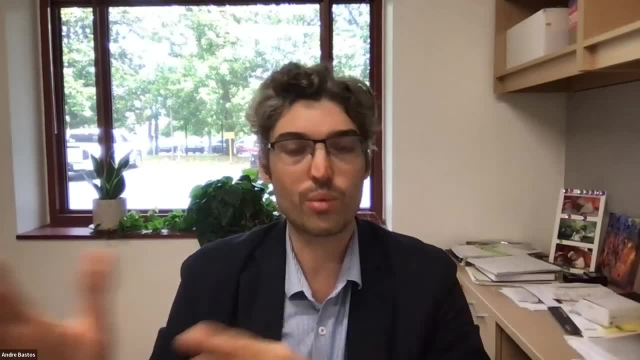 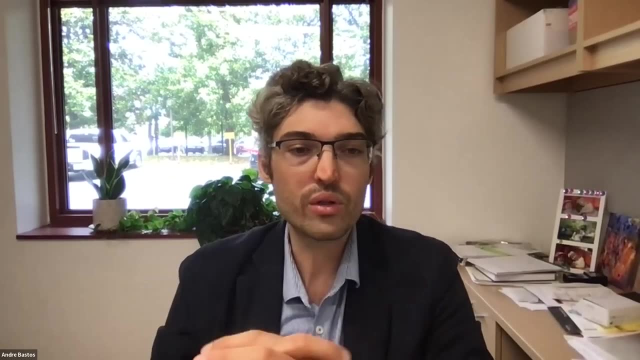 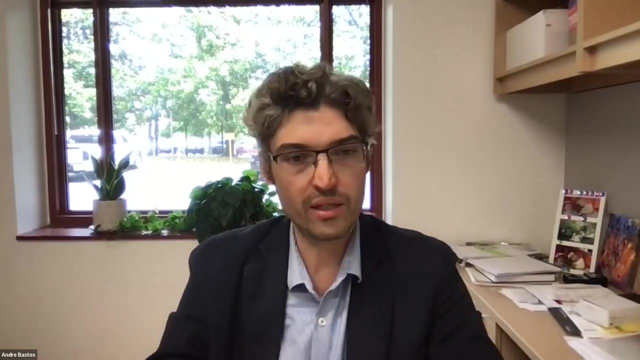 you can fine tune by hand and see what best approximates the brain. Now, that's also a very academic exercise to be doing that, And people in industry- I wouldn't expect to have a very deep appreciation for that or a large desire to want their tools to look like the brain. 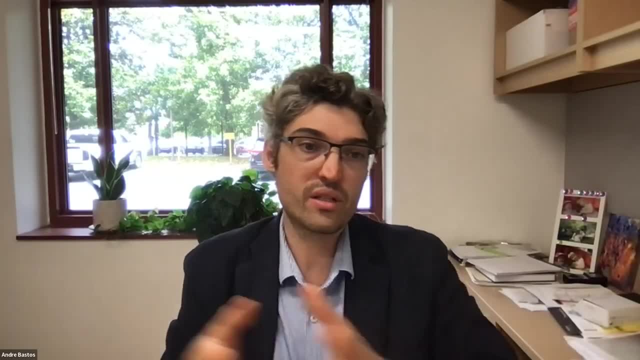 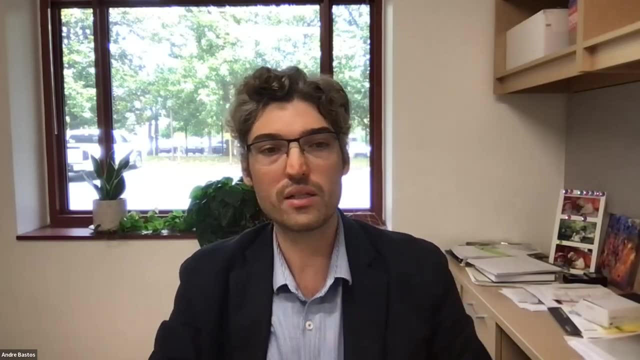 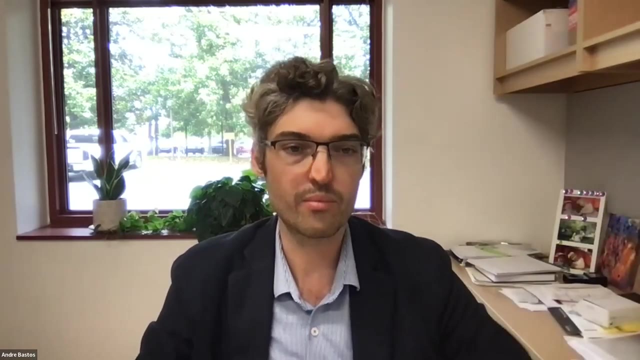 And that's a little bit. the problem I see as a limiting factor on how this can be used in neurobiology is that the machine learning and AI tools are advancing again at this record clip, but they're advancing with a different function in mind, which is to best create a product or to best approximate. 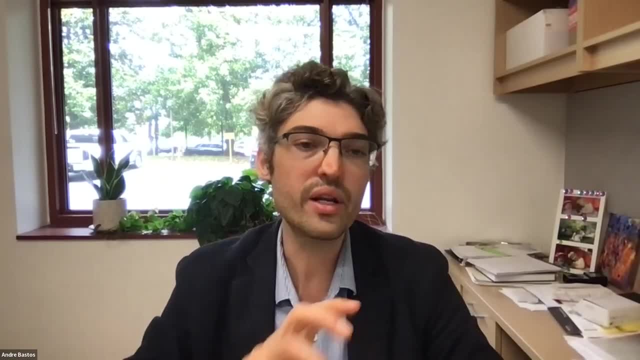 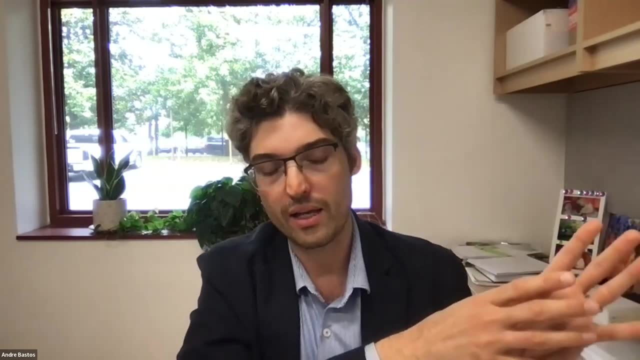 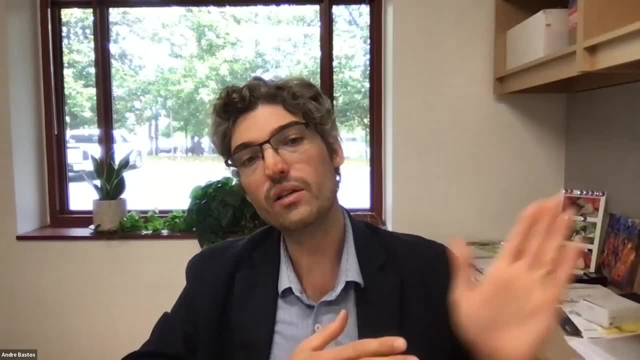 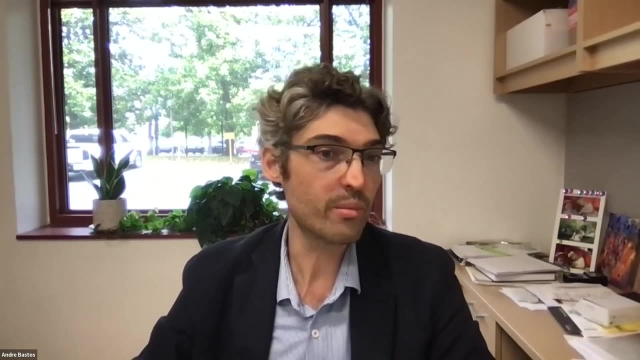 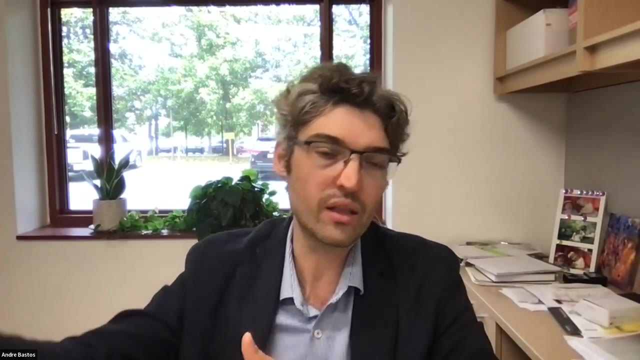 That's a significant endeavor And it's not a naive application of machine learning to brain data, for example, won't get you there. You need a lot more tools, some of which may not have yet been developed, even to understand the parallels there between AI and biological intelligence. 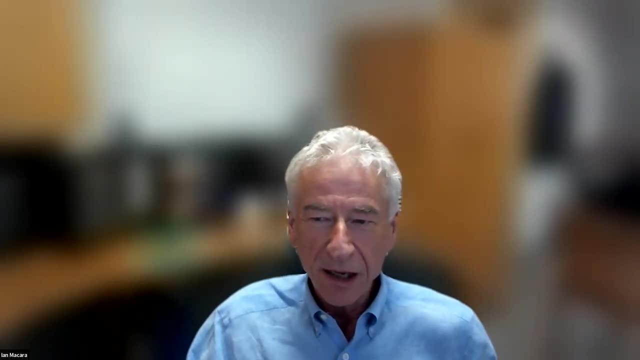 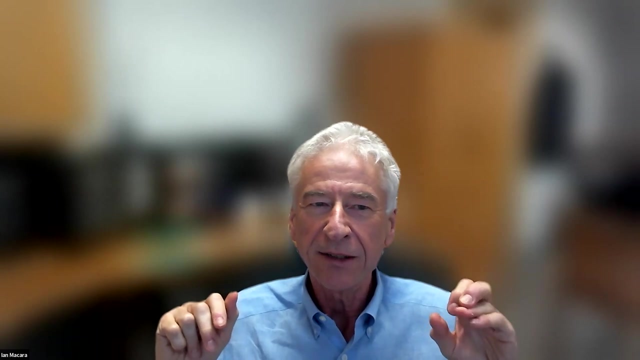 Yeah, That's very interesting. Actually, I'd like to get a sense, both from you and maybe from others to understand. the ask, Shannon, first, is how artificial intelligence is impacting your approaches to research, Because you're tackling very different problems at different scales, And so perhaps, Shannon, 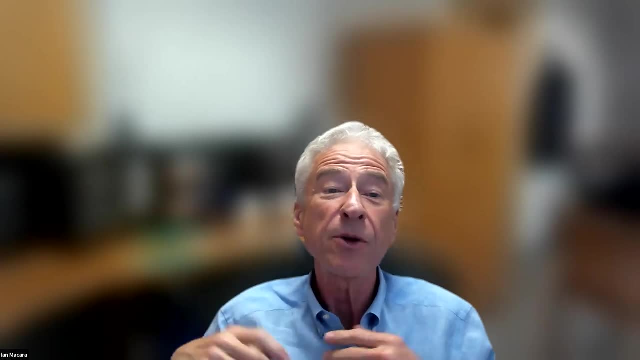 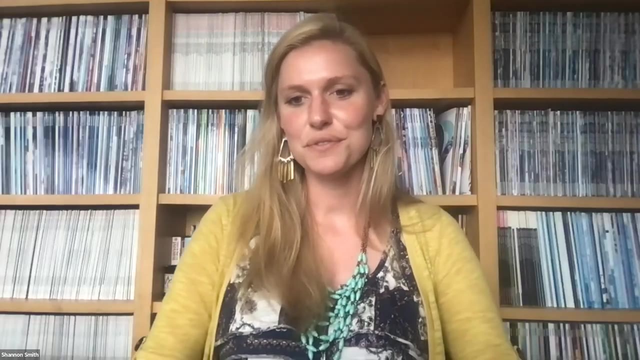 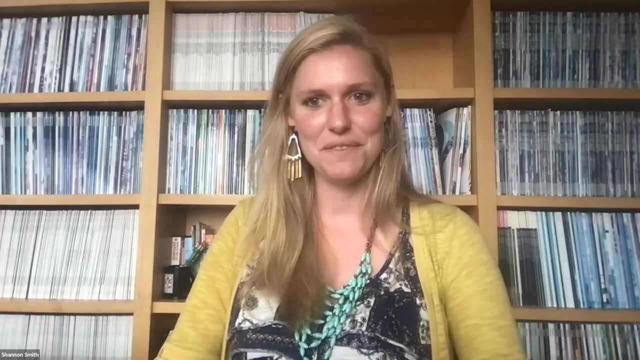 maybe you could sort of talk a little bit about how it's changed the way you're doing your research project. Sure, So, like I said, I do more of drug discovery And that's a really complicated process. For one thing, it's a very drawn-out process. Typically it takes over a decade to develop a single drug that gets to market, And there's a lot of different stages in that. You have to figure out what's going on in a certain disease that you're looking to develop a drug for and what kind of proteins are involved, what kind of you know at the organismal level. 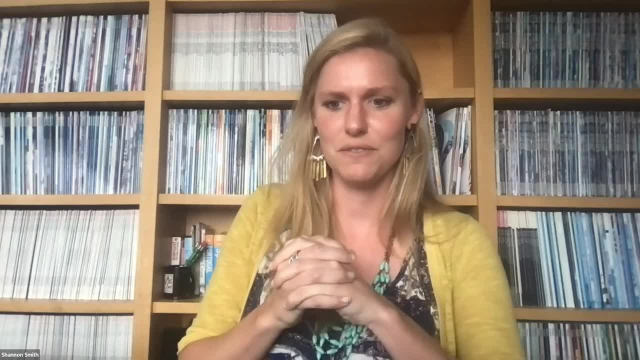 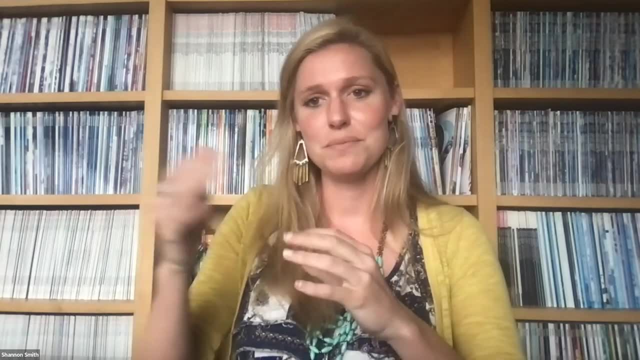 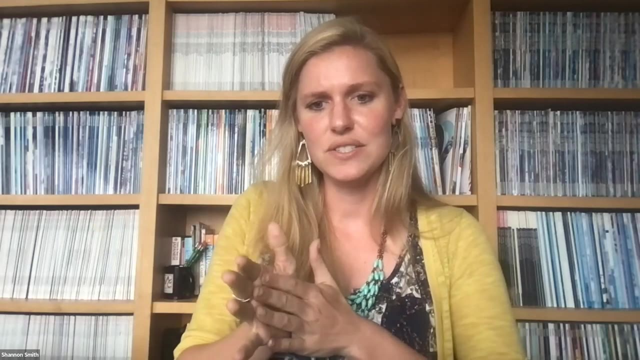 kind of what's going on and what can you actually target with some sort of a small molecule or something? Then you have to find that small molecule And then you have to optimize it, And then you have to test it and validate it for safety and for efficacy. So that's a really drawn-out process And typically 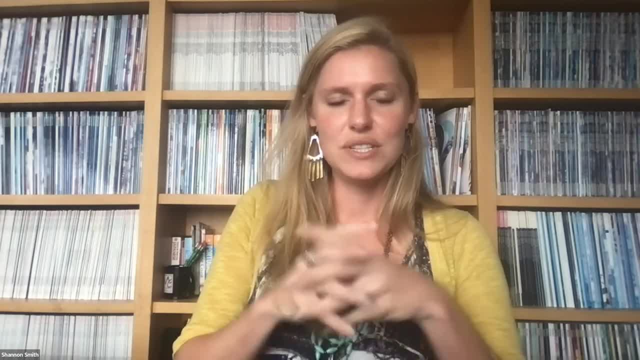 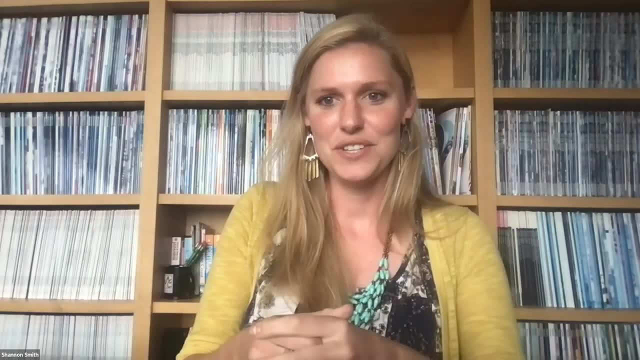 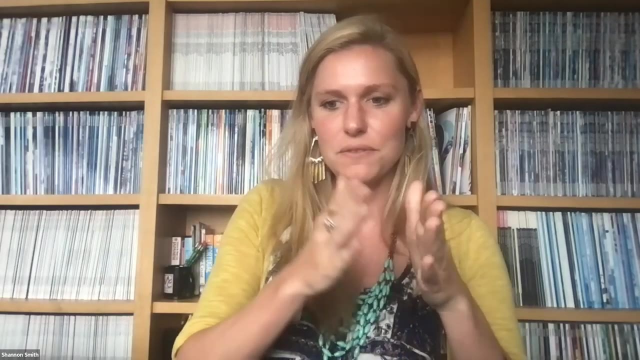 you know, we're not to the stage yet where you can do this in an end-to-end fashion, where you can say: we have this specific disease that we're interested in finding a cure for right, But we have, you know, ways to implement AI in each of those different stages. 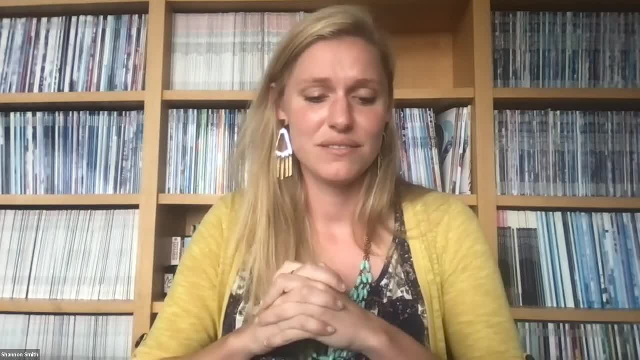 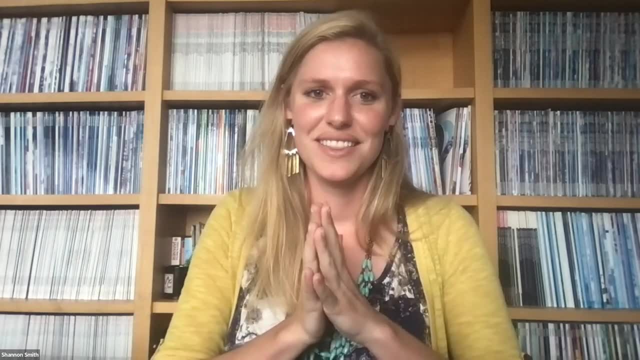 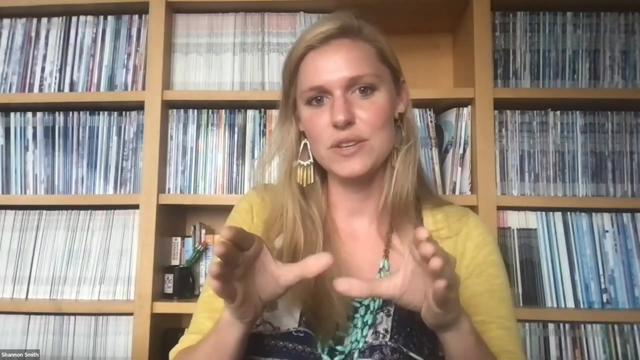 And that's kind of where it's and I'm being, I'm using it in my work. I specifically work in the. you know, let's find a compound that hits our target and let's optimize that compound. And that's just one stage of that right, And when we use a lot of AI. 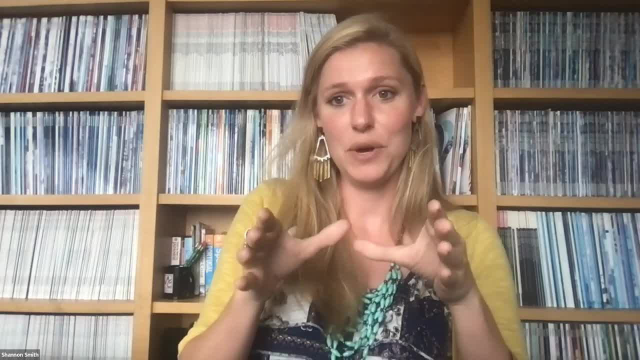 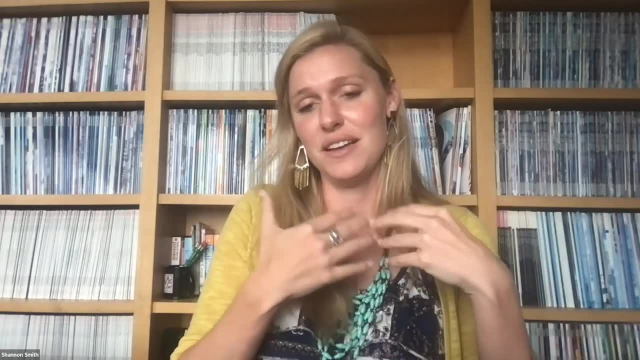 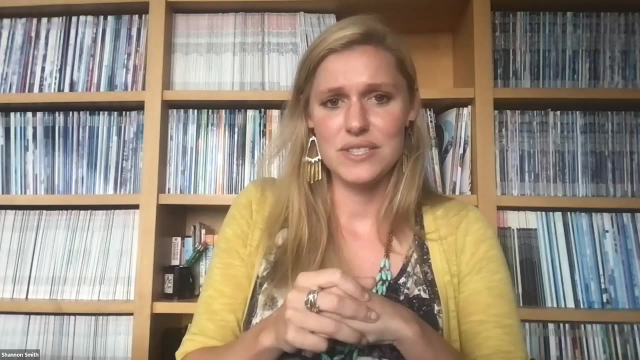 within that relatively small part of this entire pipeline, but people are using it at the very beginning, where they're trying to find a protein target that's involved in that mechanism of disease, And also on the back end trying to basically get these things you know through the clinic and see if we can test for. 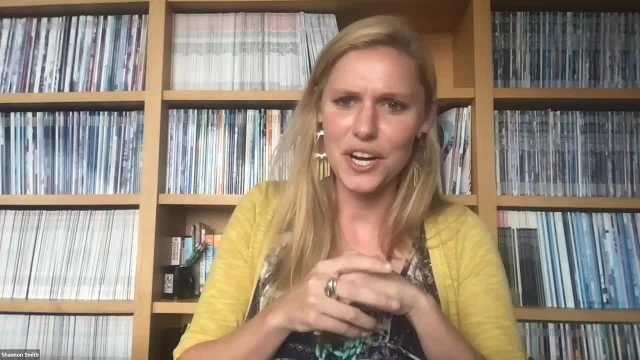 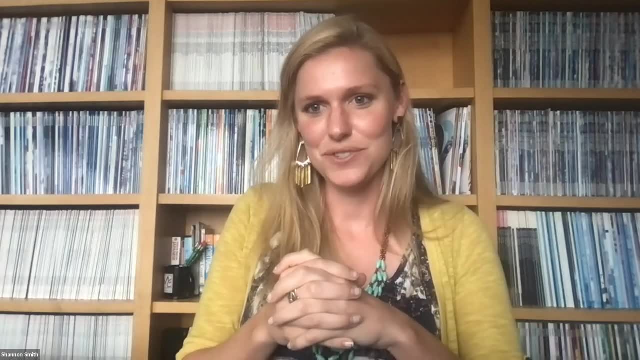 you know, test for efficacy, right, Especially in diseases that are hard to test for efficacy for, for Maybe you're looking at a preventative disease, right? Are you going to wait years to see if this drug prevents a certain event from happening? You know how do you do that. 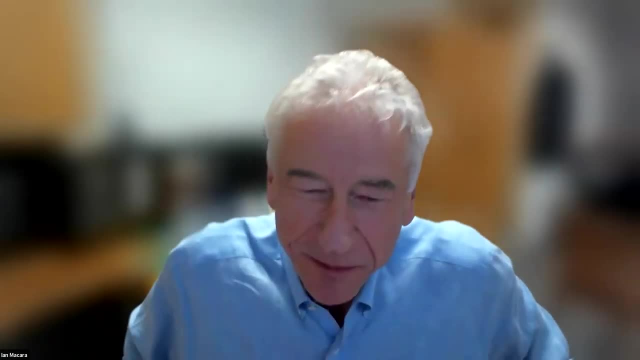 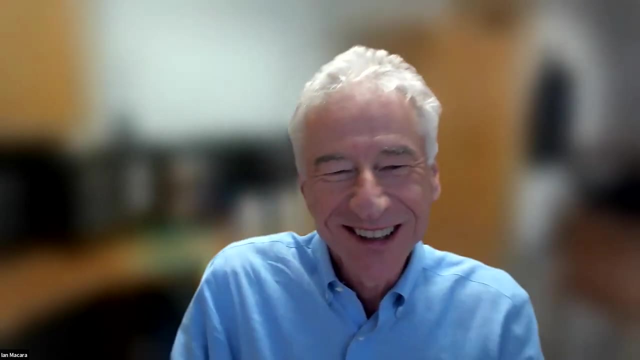 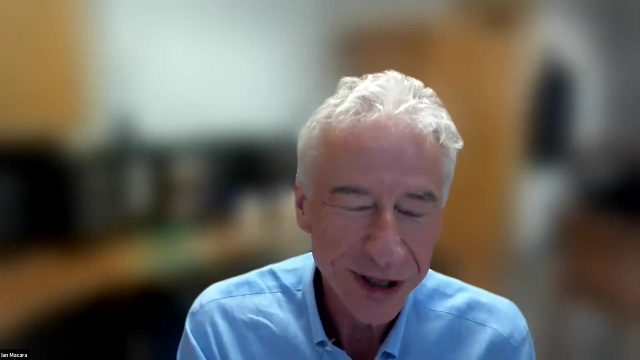 and how can we speed that up? Perhaps you could explain to people about AlphaFold, because you know artificial intelligence. recently, you know David Baker's group and DeepMind in the UK have totally revolutionized structural biology. I mean, overnight it revolutionized a whole field And maybe you 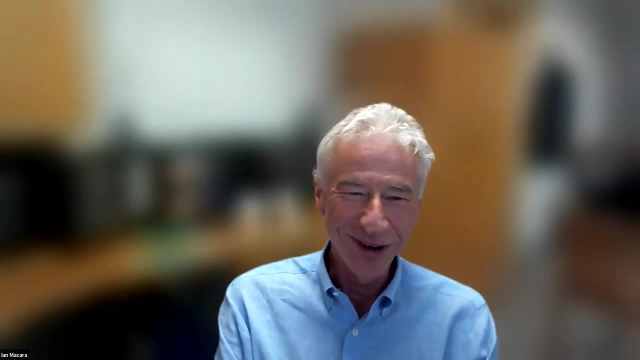 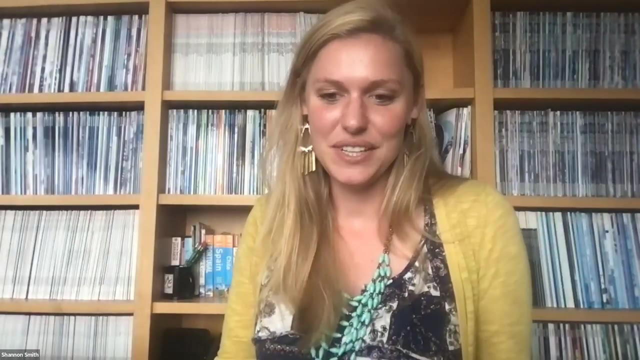 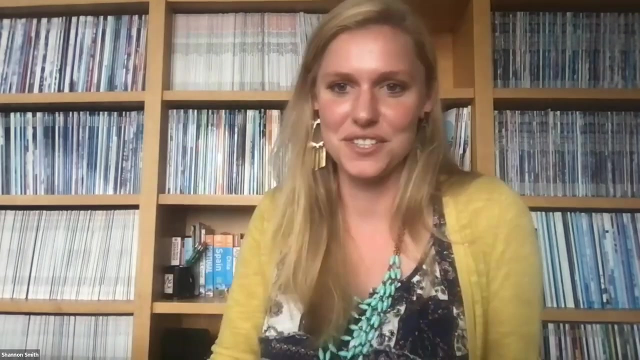 could just briefly sort of say why this happened or how it happened. Absolutely, I love talking about this. So basically, last summer, you know, AlphaFold, basically just you know, beat the competition in terms of the protein folding problem. People have been trying to do this. 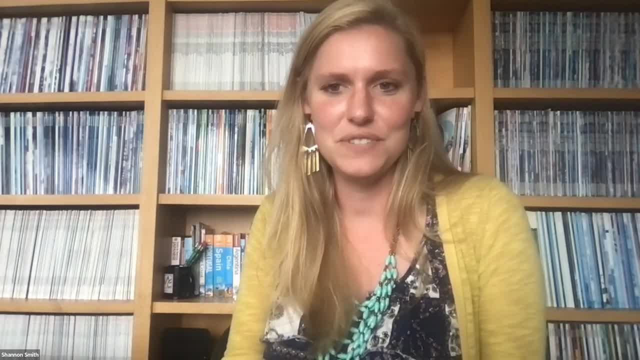 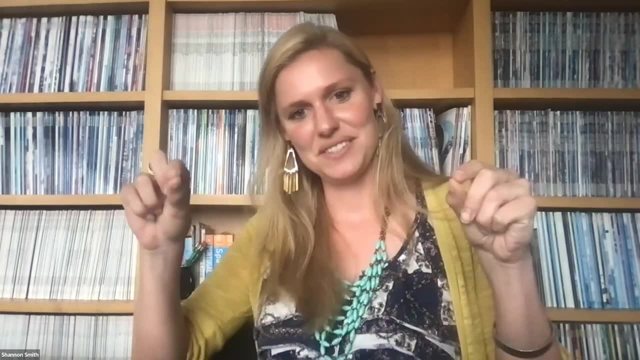 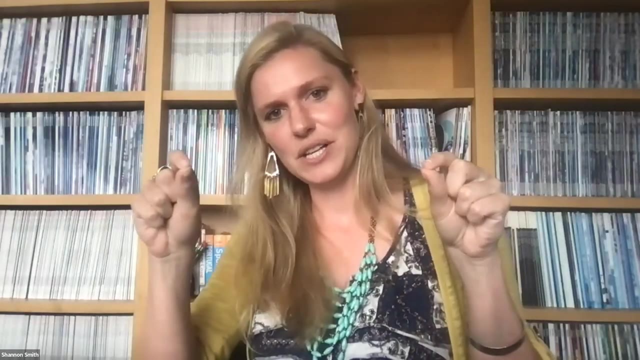 Yeah, Using all sorts of different methods for the last 50 years. And what the problem is? it's called the protein folding problem And you're given a sequence you know coming from your DNA. sequence goes to RNA, goes to protein, And you can think of these proteins as a long 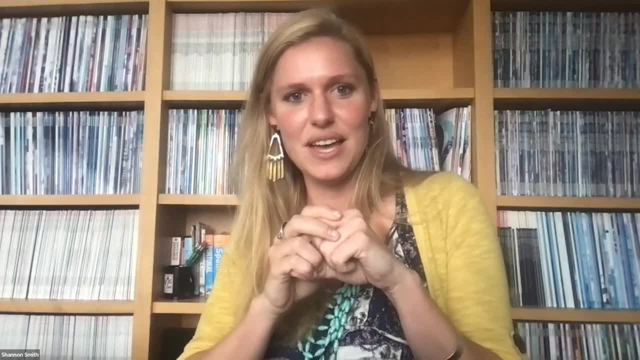 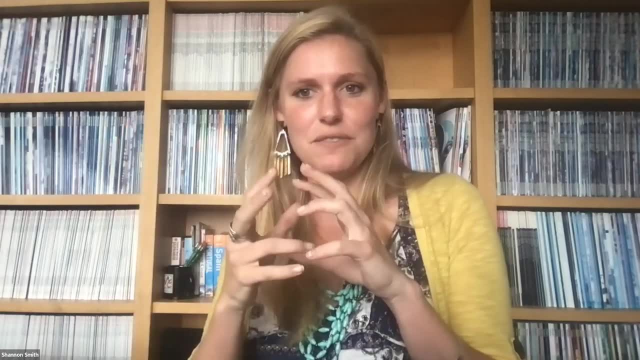 beads on a string right And there's 20 different colors of beads and just using those colors, the sequence of those, What does that look like in 3D? Yeah, How does this thing fold up on itself? And that's really important for designing a drug, or? 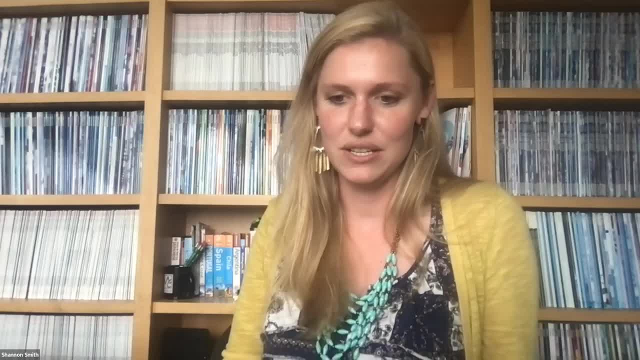 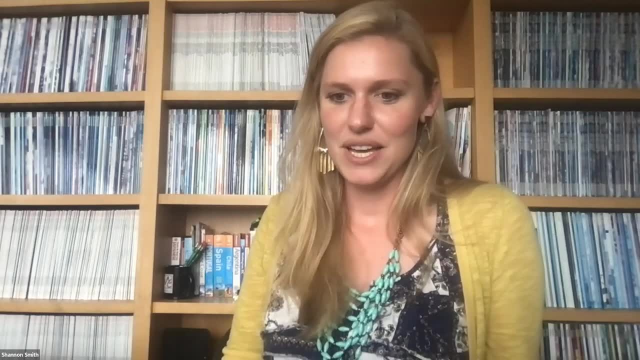 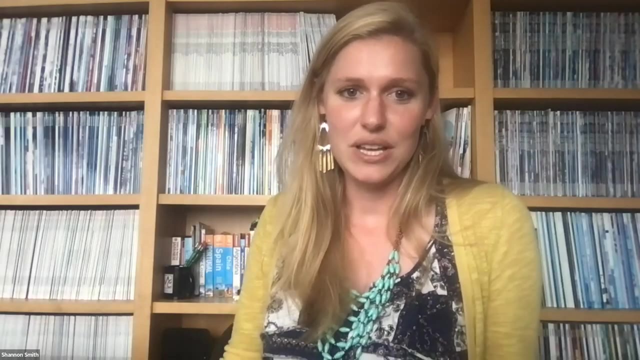 understanding the basic science of that, of that protein in that system. And people have been trying to do this for the past 50 years with all sorts of approaches. And then last summer both David Baker's group and also DeepMind within the same week more or less kind of came out with: 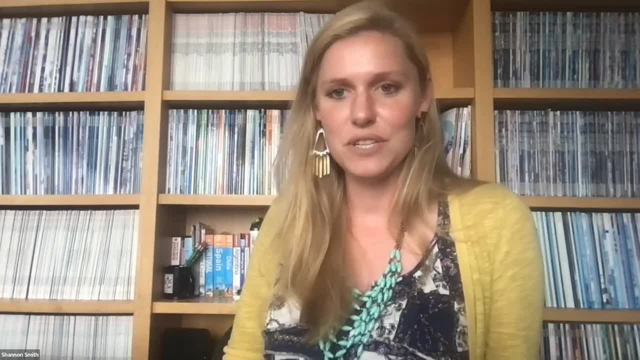 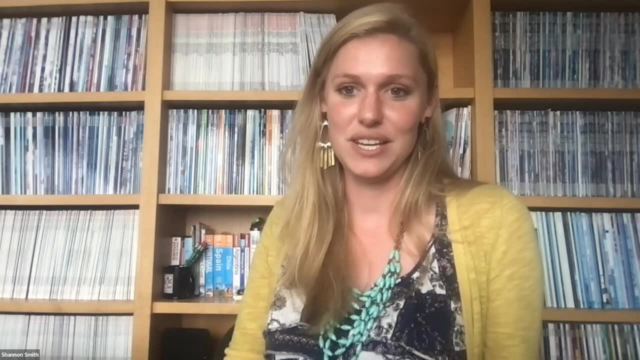 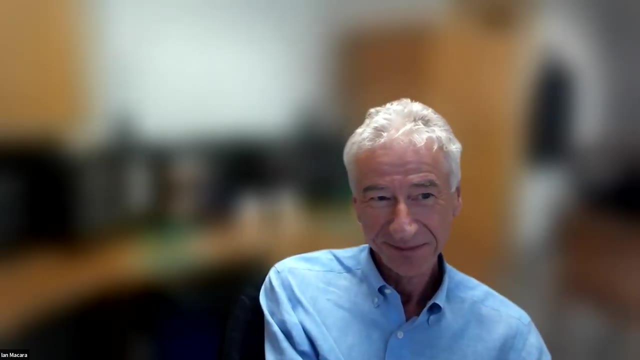 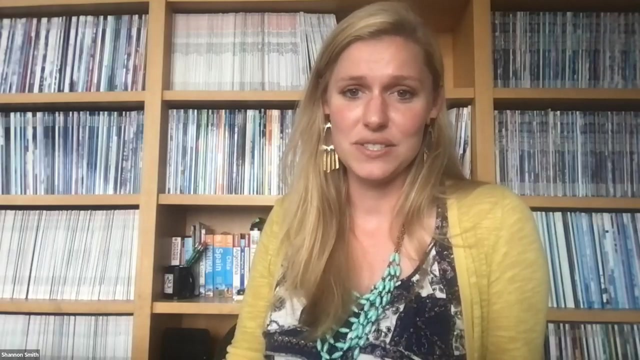 these, you know, data-driven approaches That people have been trying to do for years. but really just overnight, like you said, just kind of came out and said, Hey, we kind of solved this problem, Solved the problem, And they, they sort of did. I mean they took a huge step in the right direction, Absolutely. And they also provided a database where it's, you know, anybody who has internet connection can go and search for their protein that they're interested in and get a predicted structure out. 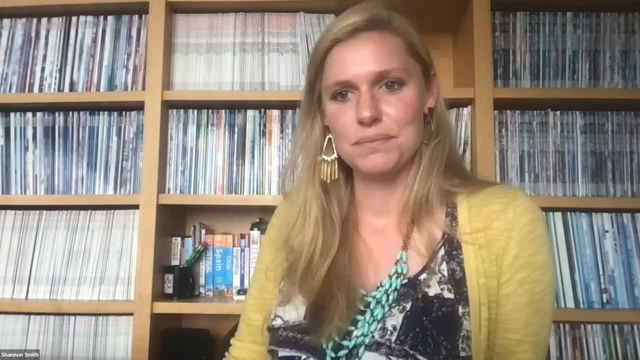 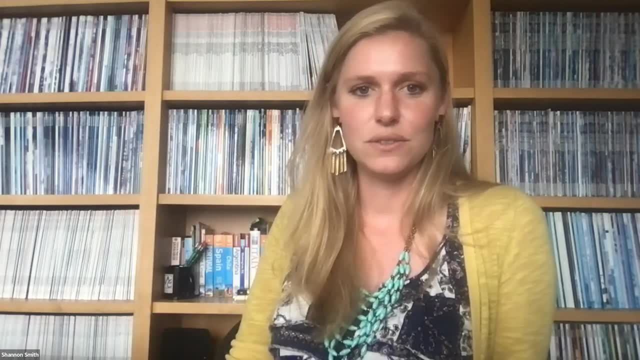 And that was just a database, Yeah, Yeah, And they really really played into that, And so that's where they got the data problem Right. That was, they did it simply. They didn't use any sort of biochemical or biophysical, you know, simulations which we've been working on trying to understand the actual mechanism of folding. 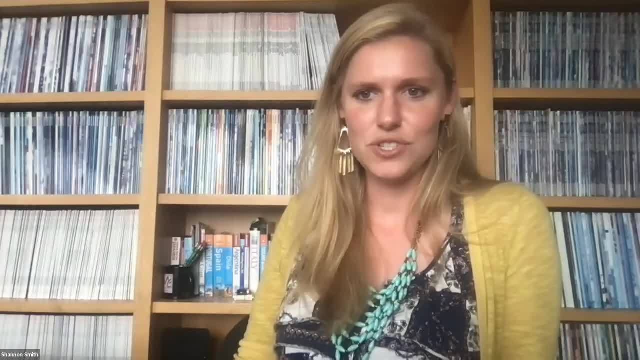 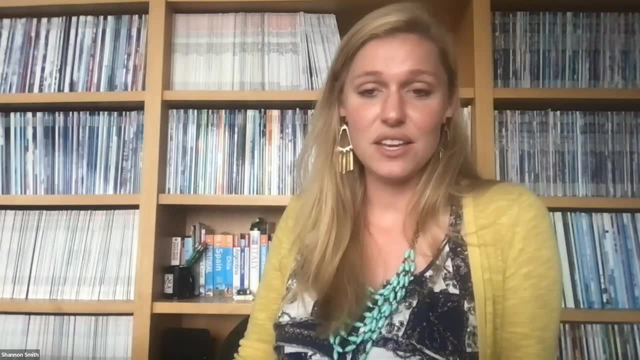 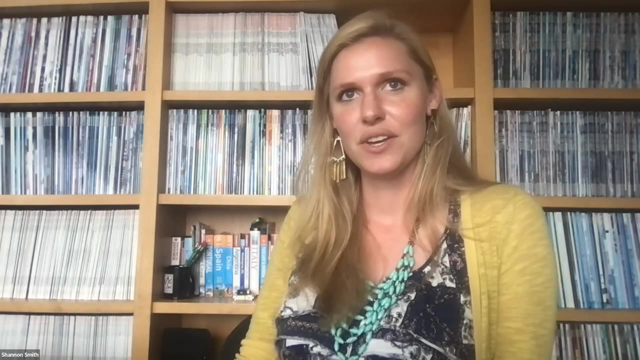 They just took these huge sequence and structure databases and put them in and made it a big data problem And they were able to solve it that way, And that completely is changing the biomedical research landscape. things that were once untouchable from a structural perspective are now. we at least have a. 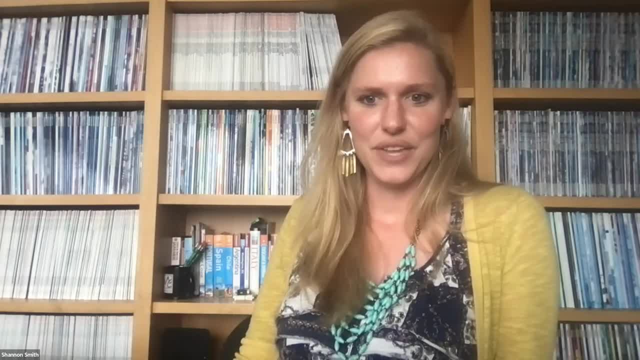 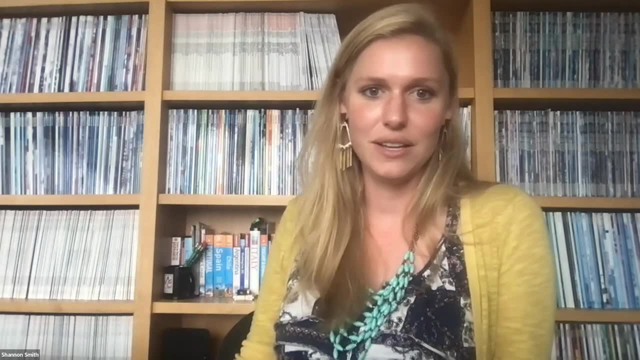 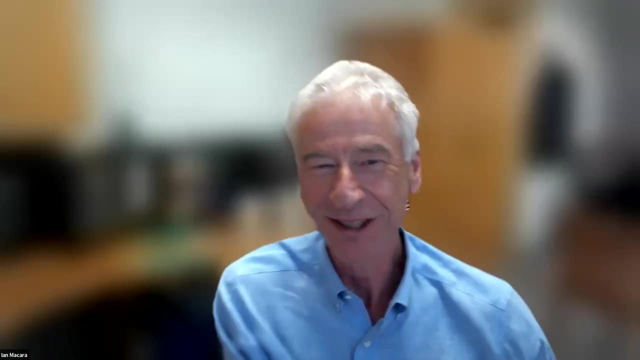 have a first step, first big step, in understanding what that looks like and how we can begin to use it, and something that could potentially be medically clinically relevant. and it's really cool, really, really cool. it was absolutely mind-blowing when it first came out, really. 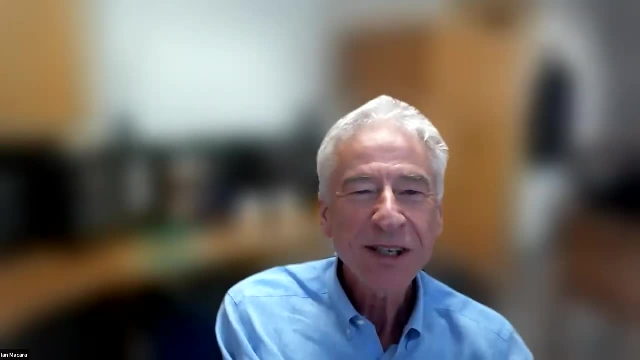 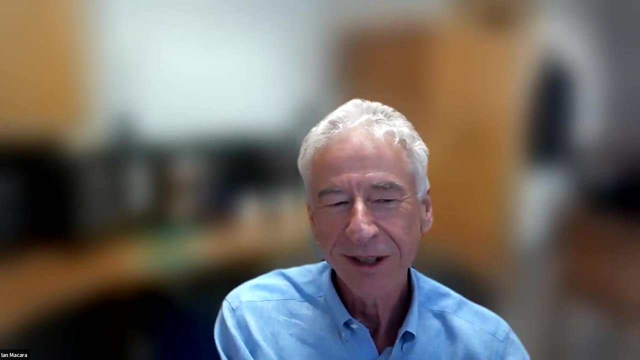 absolutely astonishing. yes, so actually i just want to go back to something andre said. i asked jesse about. this is this idea that that really you know the way machines think is right is could be quite different than the way humans or primates think and they're not really designed to think in. 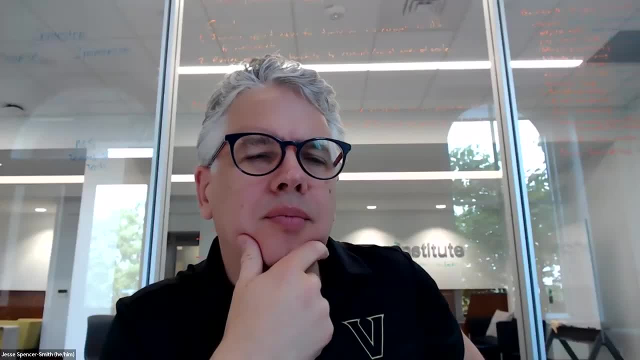 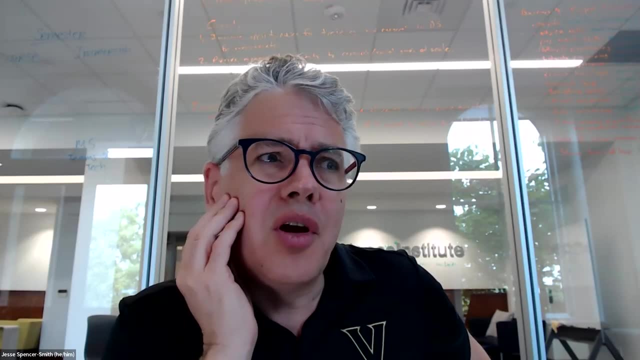 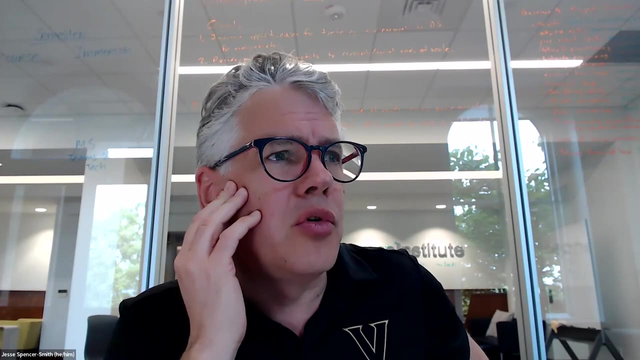 the same way. no, that's right, um, but but so, yeah, how, what's your take on this, jesse? no, i know, that's, that's absolutely right. uh, you know, early on, when we first started to make progress with, with vision models, um, these were convolutional neural nets and the convolutional 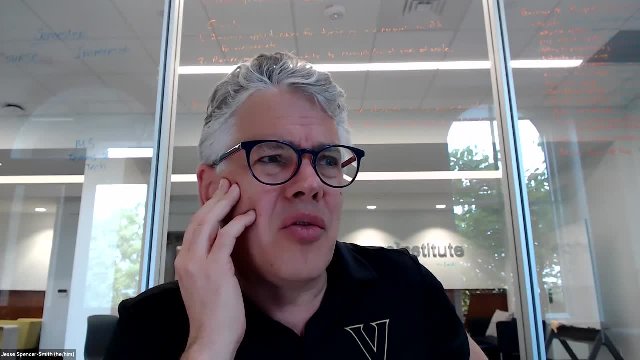 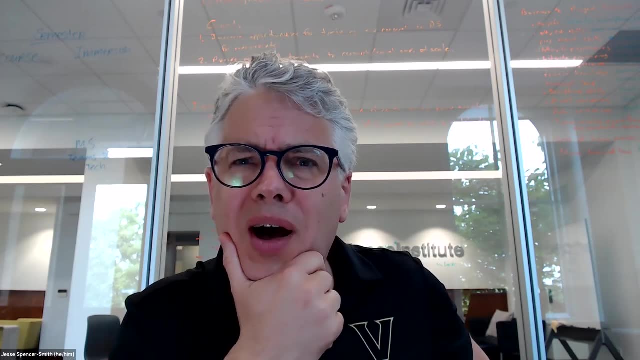 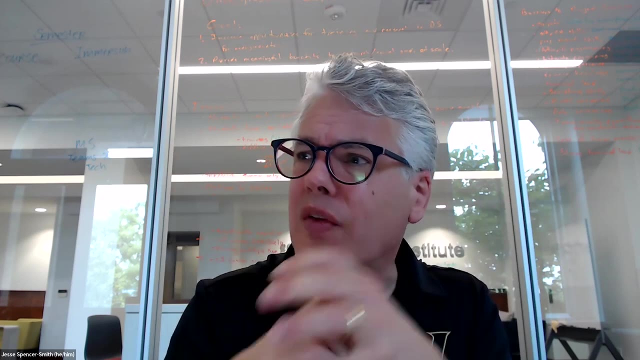 neural nets were designed to sort of ape, uh, the, you know, v1 visual cortex. we we sort of took a page from there to sort of figure out how to make these, these networks, work better. uh, and some of the representations might look kind of similar in terms of similarities between objects, but man, the 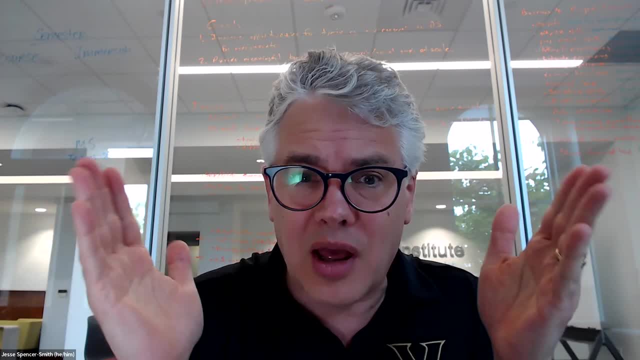 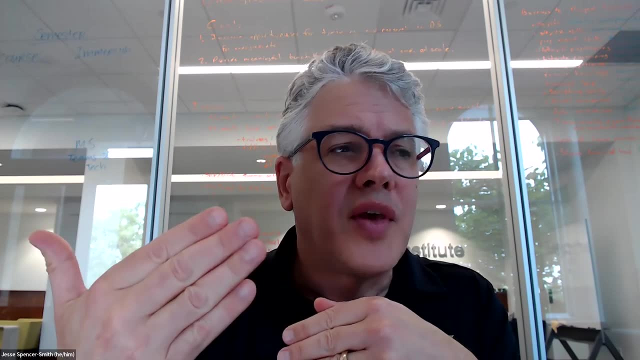 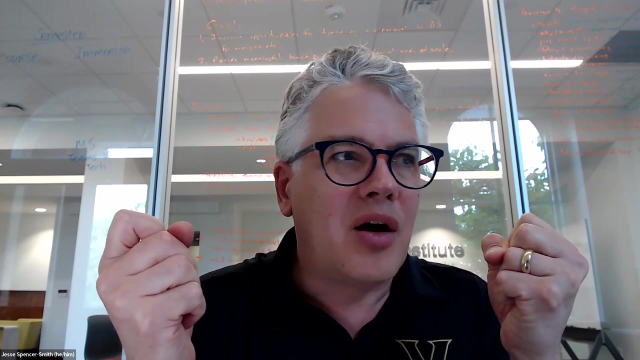 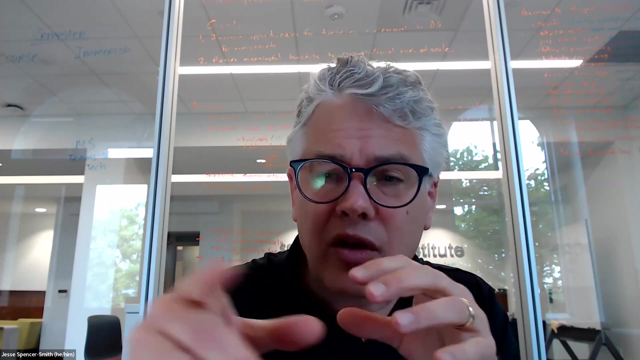 learning mechanism is completely different than than how we, than how we do it biologically. and and now, with this new generation of models, these transformer models, that looks completely different. the representations that you see, uh, you know what's being attended to. uh, you know how this is distributed across the network. it is very, it is very alien. um, and the questions ken lau mentioned: 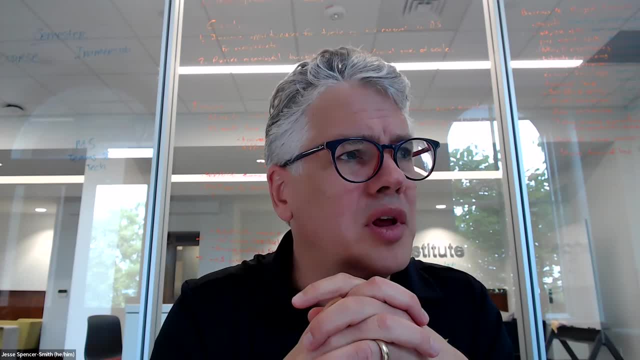 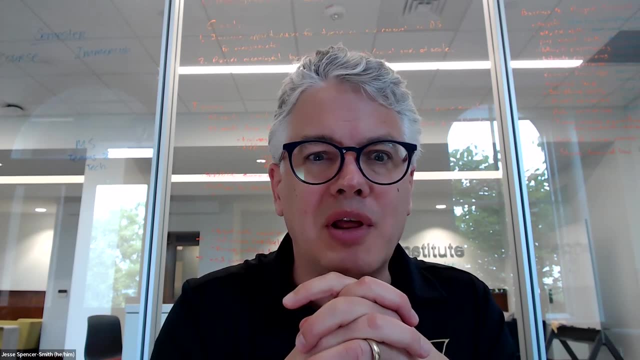 alpha star, which was uh, uh, early, early, uh effort to uh, uh to see if an ai could play starcraft 2, and it did, and it and it's. you know, one of the things that we've been trying to do over the last couple of years is we've been trying to figure out how to do it in a way that's not you know. 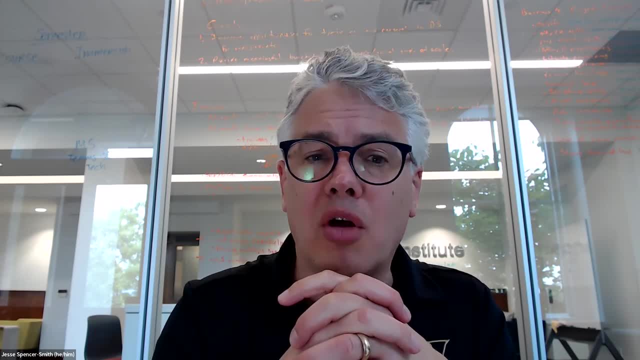 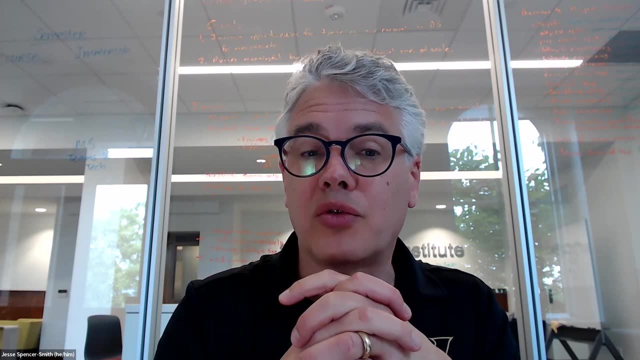 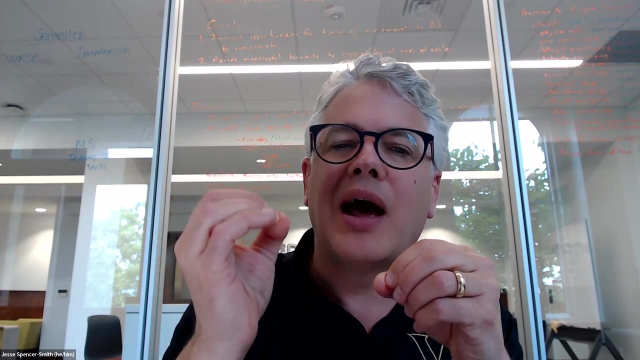 world-beating, but it plays it in a way that humans don't play, so absolutely. these are very different ways of solving solving problems. it doesn't mean that they're not useful, because they can provide solutions or suggestions for solutions, and you can also probe a bit to understand how it's being. 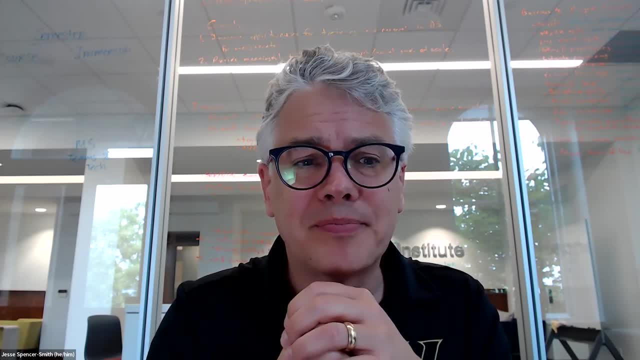 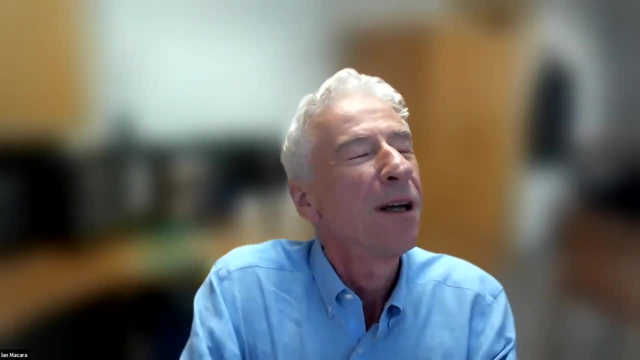 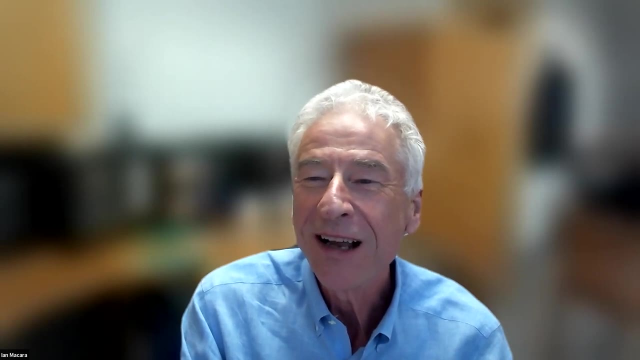 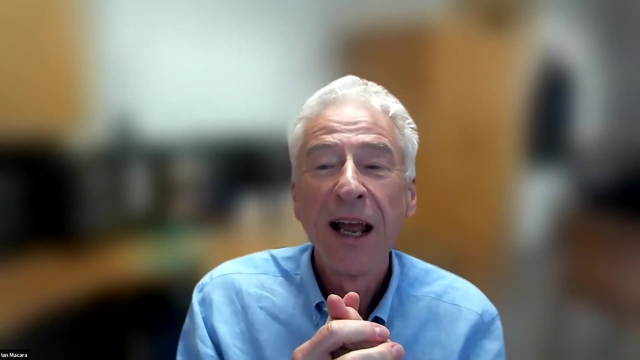 represented and how things are happening, but but by and large, it's not gonna. it does not look like humans. what is interesting is because, um, what you know- i'm just reading ken's question here about, since we don't really look inside the black box to see exactly how it's coming up with a answer. you know, and how. 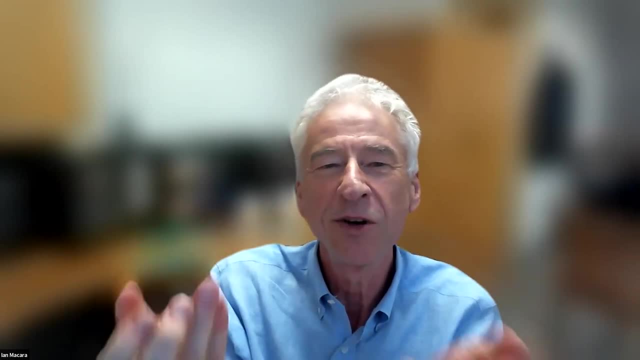 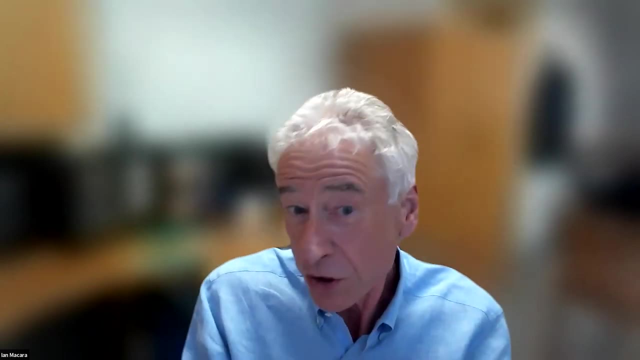 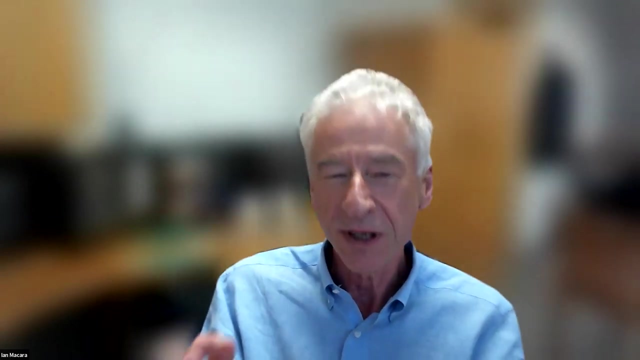 trustworthy is it so? for instance, if you know shannon or andre are using these tools to try and probe the research question, you know, if you don't know how it works, how trustworthy can the answers be? And I've heard that even small changes in parameters can give you completely different outcomes, or at least 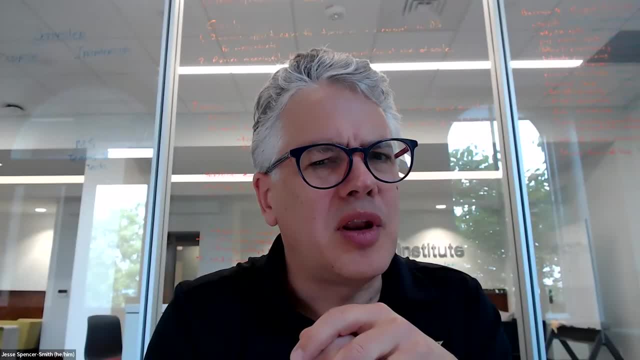 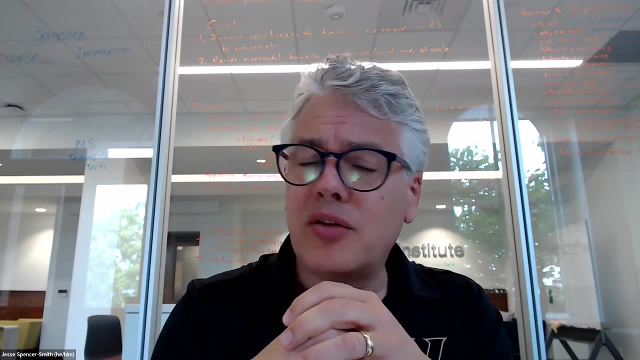 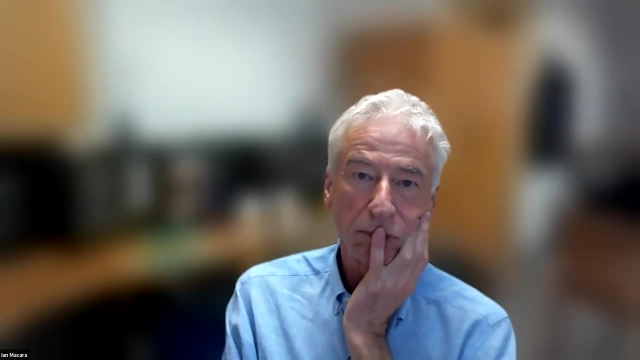 in the past. whether that's true now or not, Depending on the network, you'd be more sensitive to that. The interesting thing about these large language models now is that in some sense, you can ask them to show and to represent how they arrived at some of their conclusions. It's 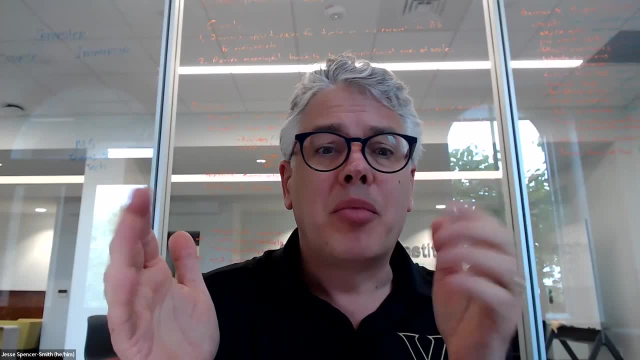 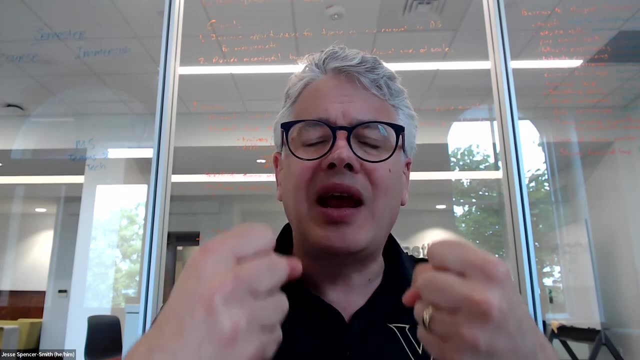 becoming more and more feasible. But absolutely, you know you have problems with. you know, if you think about it, these networks learn off of the data that they are shown. So they do self-supervised learning on the data that they're shown, whether it's text. 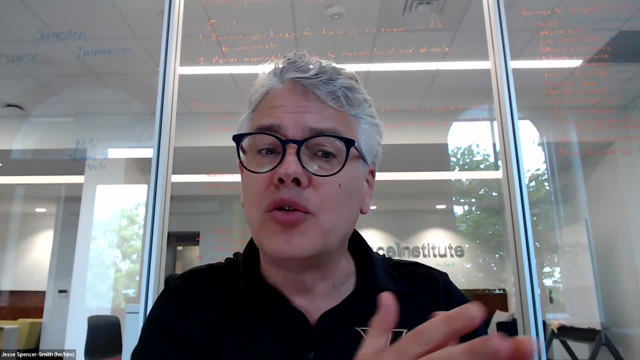 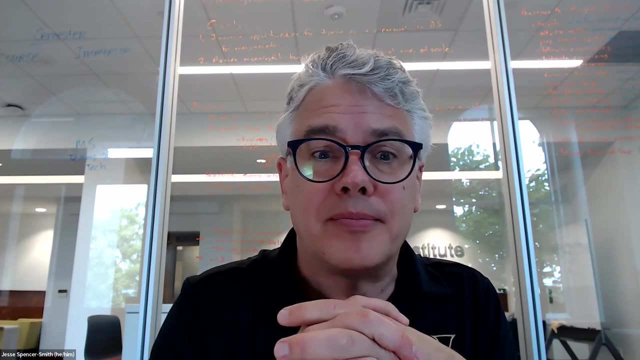 proteins, audio, you know- images. they're learning on this. So think about where the text comes from. For the large language models in particular, it comes from the internet. You know, is there ever anything problematic that you ever read on the internet? 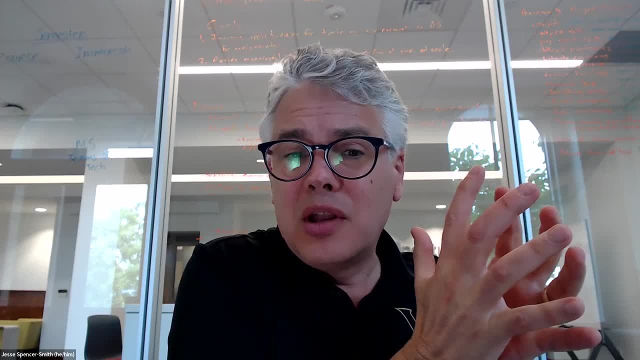 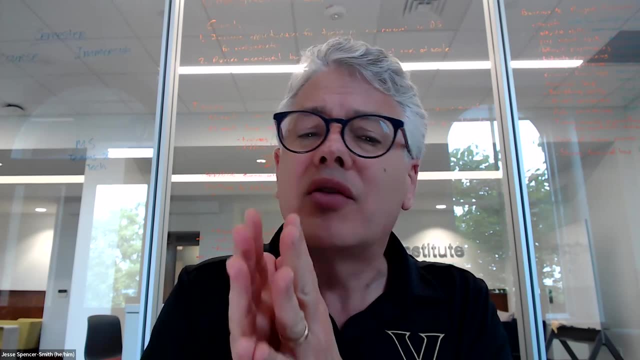 Well, these models are learning that. So it's not just that it's a little bit unclear, but there is also a large problem with bias as well. So it's a huge area of research and of understanding. There are some ways to mitigate, but it's something that's important to recognize. 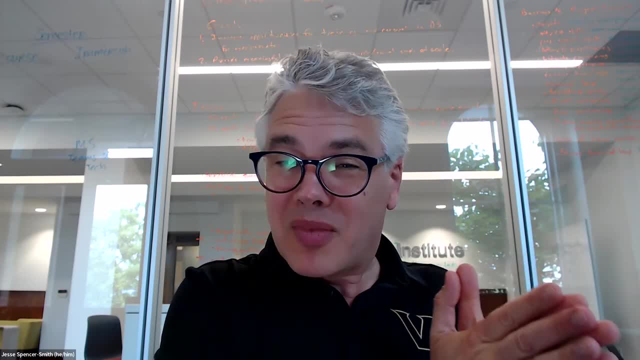 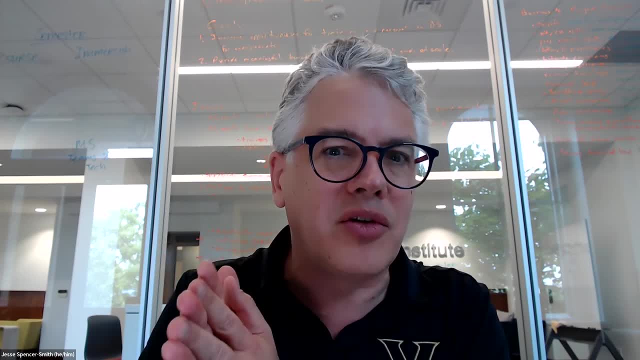 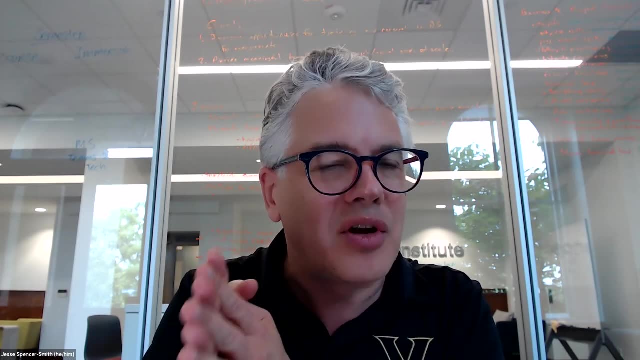 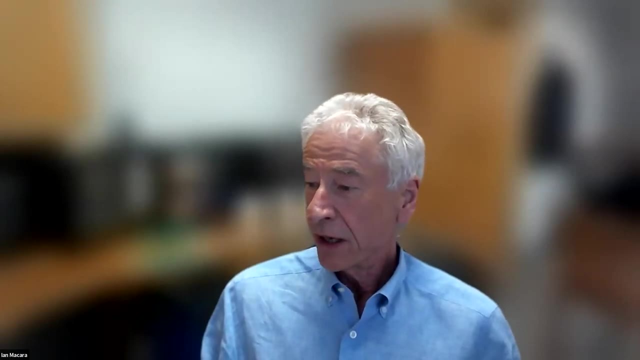 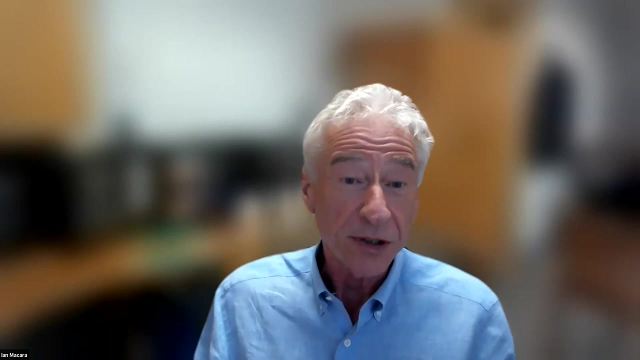 where we're careful in how we apply the models, We augment decision-making rather than replacing decision-making. We have checks. We have ways of validating. That's going to always be important. I can see this being a problem with things like using artificial intelligence in radiology, for instance, doing diagnosis. 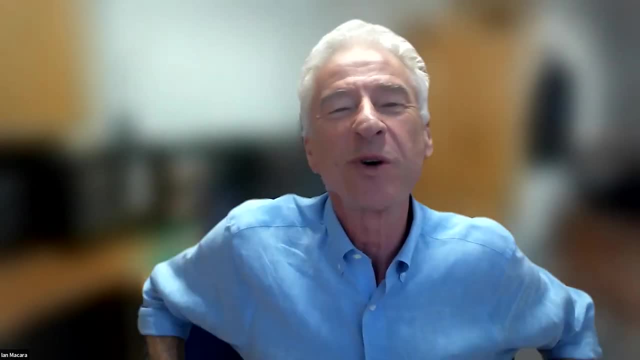 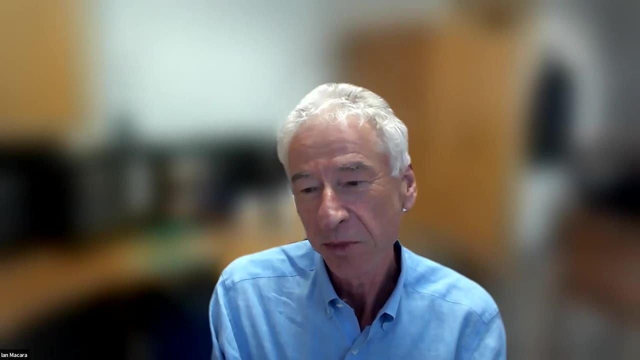 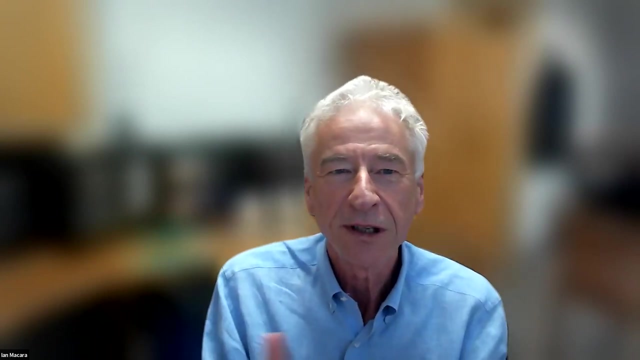 right If you don't know how trustworthy will the diagnosis be right If you don't know how they're arriving at those diagnoses in a medical area Actually? so, Andre, maybe we could go back to your research and how you're using AI for studying cognition in primates and how you see 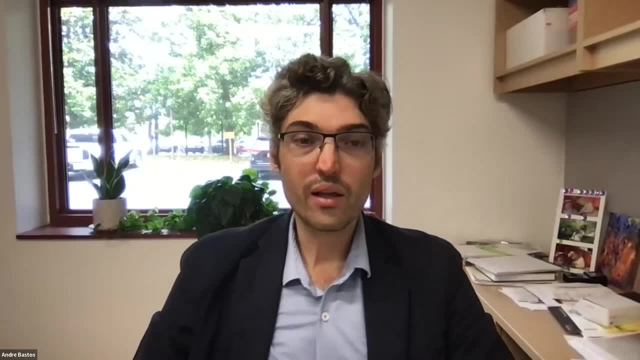 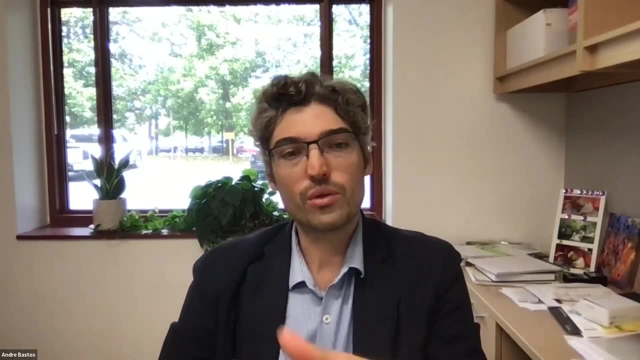 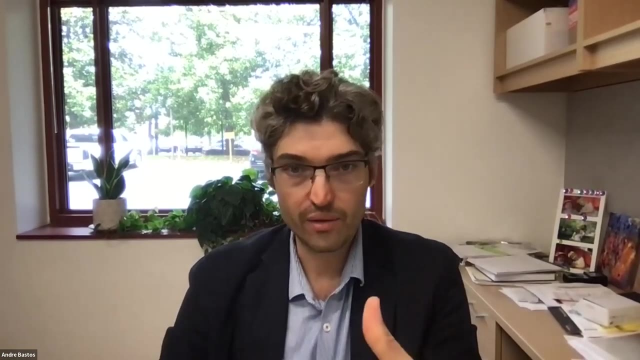 in the future that that's going to expand Absolutely, Yeah. So for us as neuroscientists, over the last few years we've been able to scale up in a really radical way the amount of data that we're able to collect, And so, for example, if I want to look at the brain, right then I'm going. 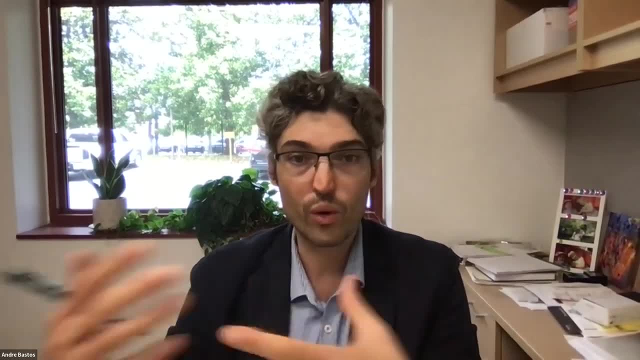 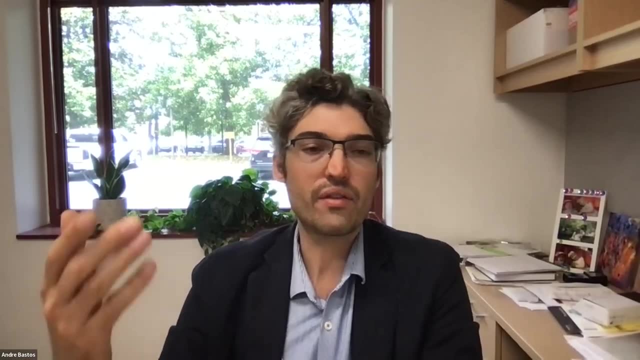 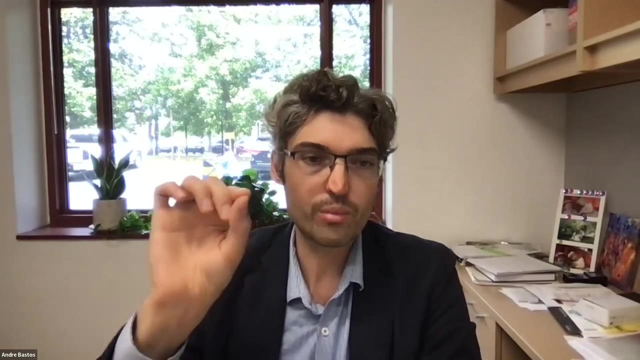 to do an anatomical study which will involve looking at where neurons are and what different neurons are expressing, what kind of proteins they're expressing and so on, And it used to be that you would have to perform a few of these sections and then under a microscope individually. 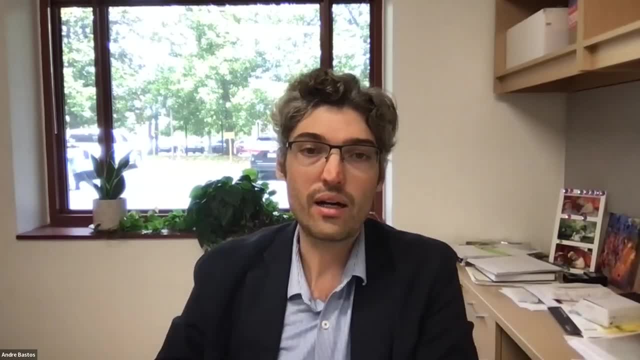 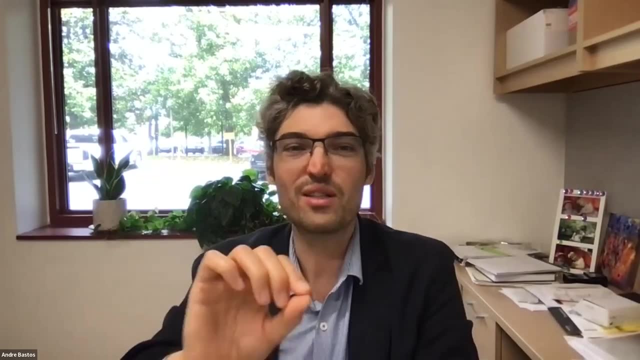 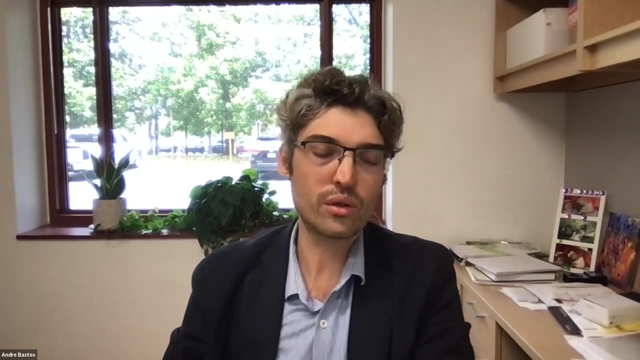 by hand and count neurons by hand, And that's still how a lot of our fundamental knowledge about the brain was done- was by, you know, a poor student, usually sitting under the microscope. you know, counting for hours these neurons. So imagine that now you have a tool where you 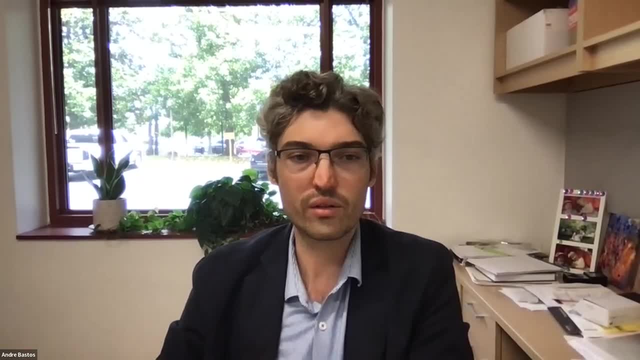 don't have to do that anymore. You can train the machine learning algorithm to recognize what a cell looks like, potentially recognize what different types of cells look like, And now all of a sudden you can get a very, a much higher throughput, And the amount of throughput that that would increase can be. 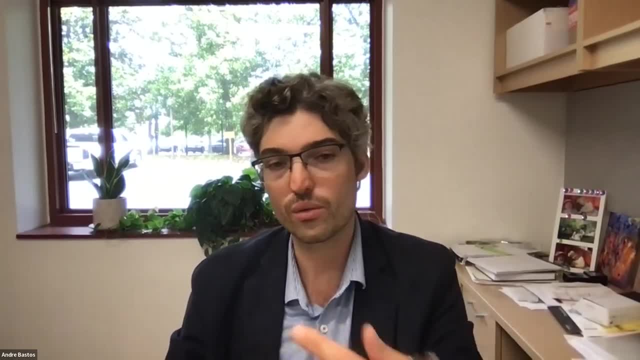 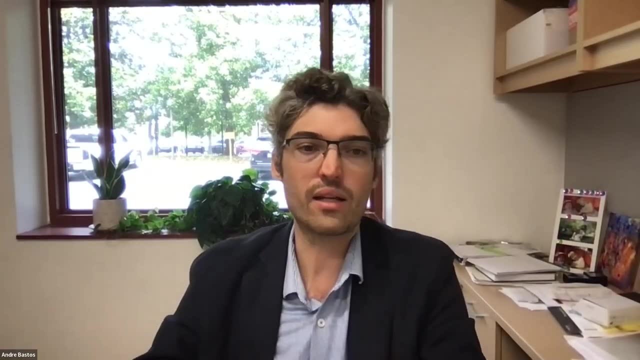 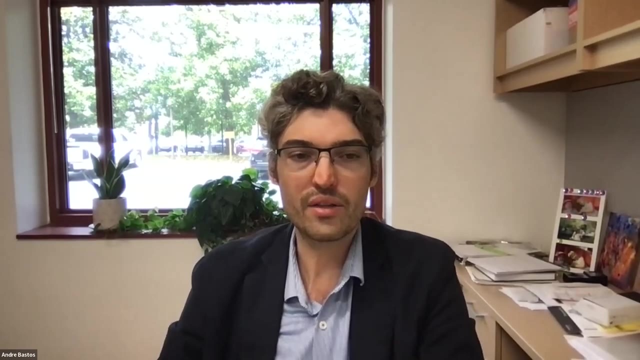 measured, you know, in multiple orders of magnitude. So we're talking about times 10, times 100, times 1,000, or the same amount of data can be gathered and analyzed in, let's say, one-tenth or one-one-hundredth of the person hours. So you can think about it either as 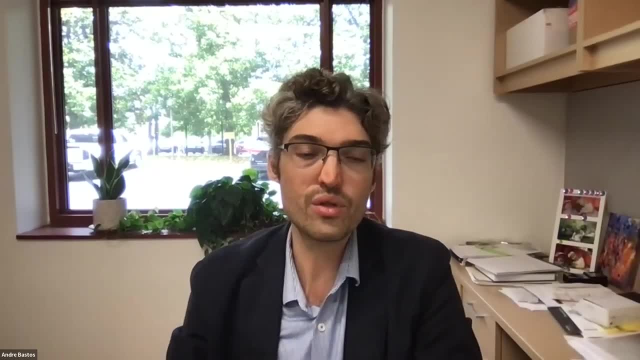 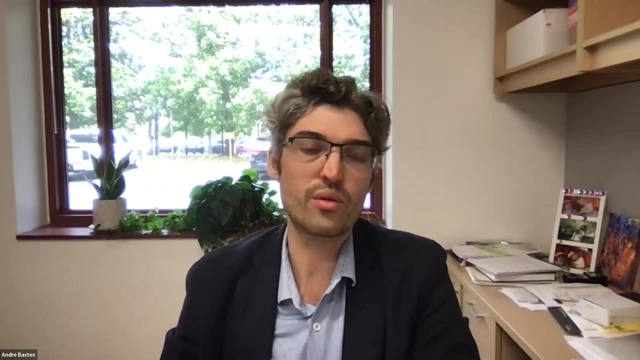 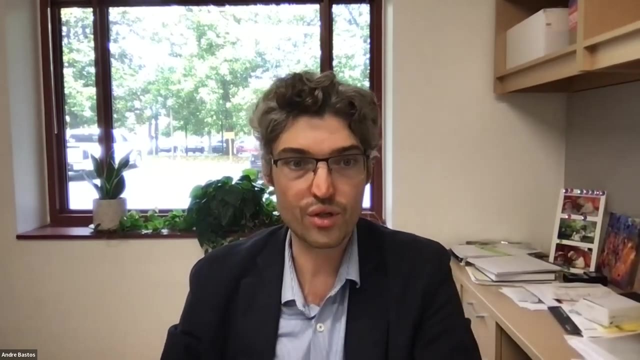 expanding the amount of data you have access to or radically reducing the amount of time to process. In my own experiments, I've used these types of tools in order to be able to make sense of more neurons that we record electrophysiologically, that is, recording their electrical signatures, in 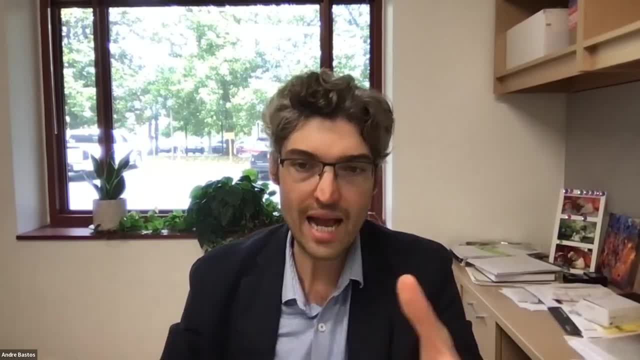 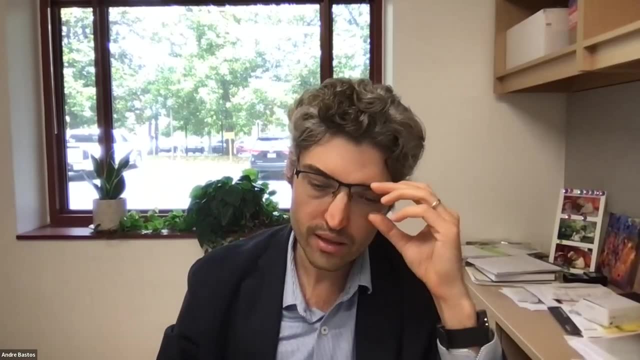 the brain. As you all may know, neurons fire action potentials. Those are changes in the electromagnetic properties of the neurons which we can detect And that's how we think the language of the brain works. We think that it works through action potentials in one particular type of neuron. 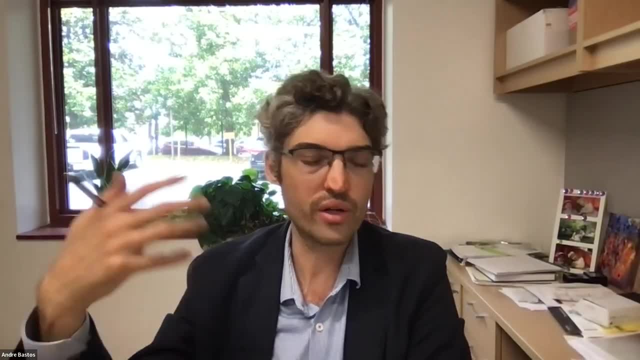 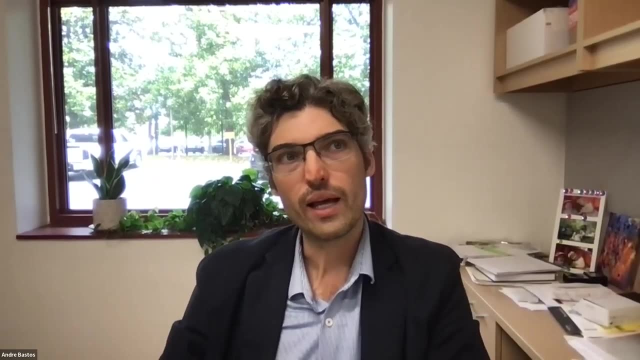 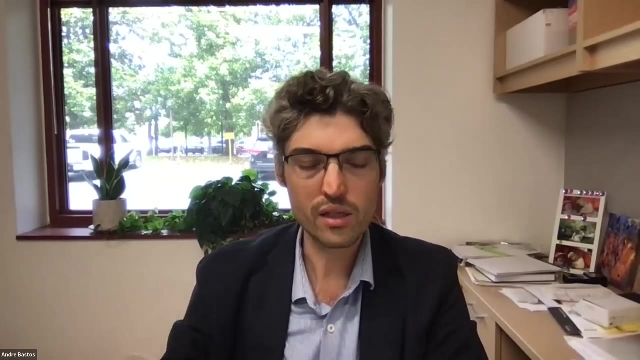 signaling the presence or absence of something in the environment or in the internal milieu of thoughts and then relaying those messages to other neurons And at that level, in terms of being able to record from multiple neurons, we've also made tremendous progress on the data front. 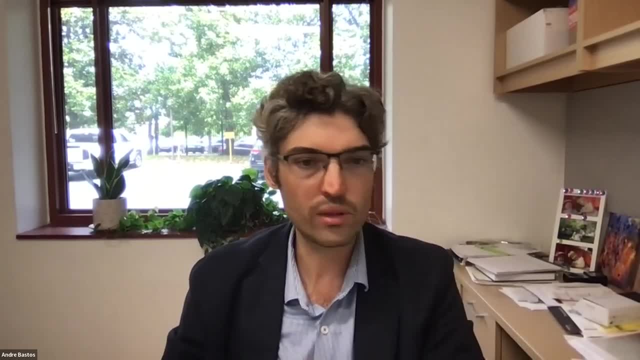 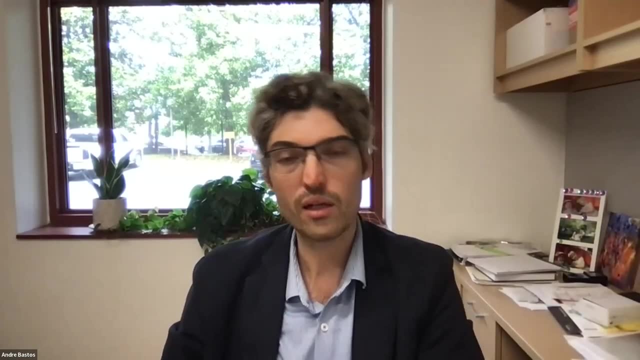 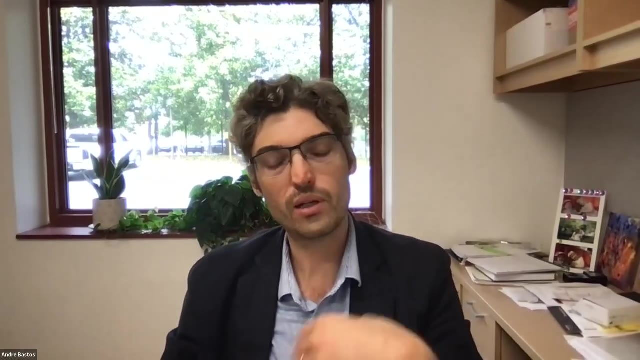 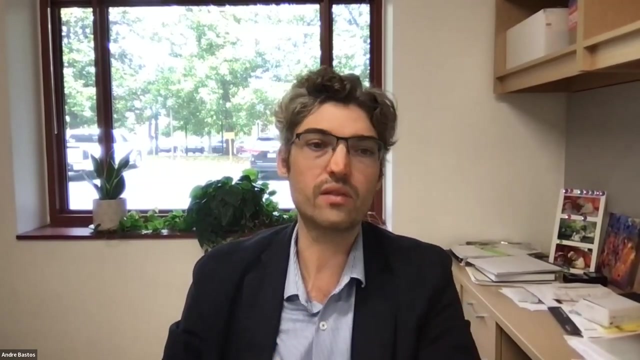 So about 10 years ago it was only feasible for a typical laboratory to record maybe dozens of neurons simultaneously at an incredibly huge cost. But now we have access, for example, to data sets containing thousands of neurons, and that's becoming increasingly available to middle-sized laboratories, And so we've really seen an expansion of about 100 to 1,000,. 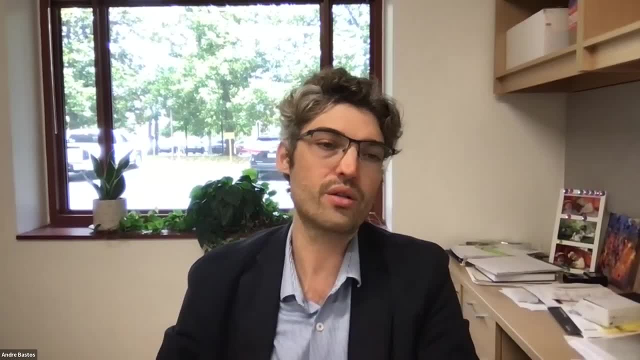 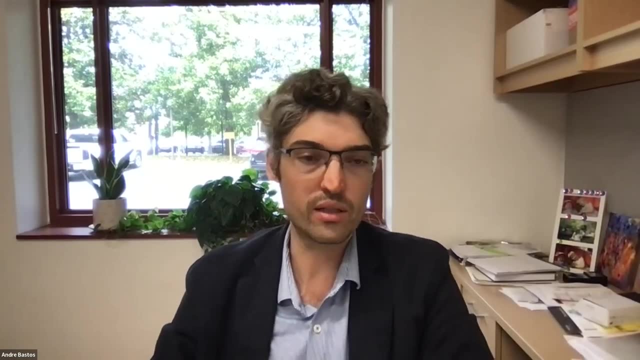 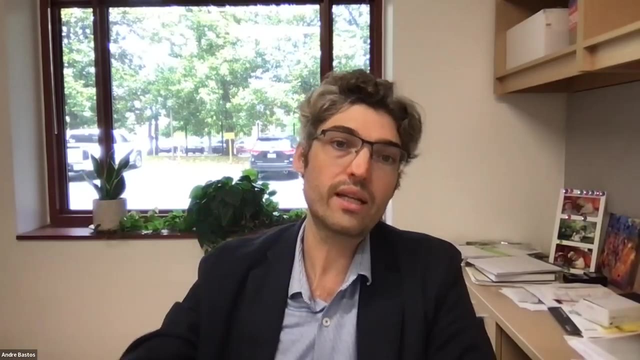 and that is going to continue in the next coming years And we can look forward to another expansion of around that one or two or three orders of magnitude in the coming years. And so increasingly and then again, in that field we're seeing some improvements, but also we're seeing more of a shift in the way that we're. 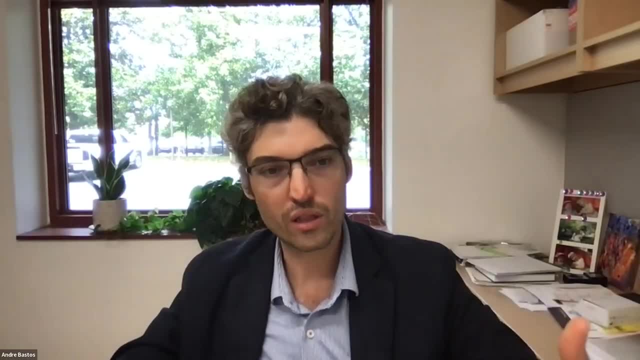 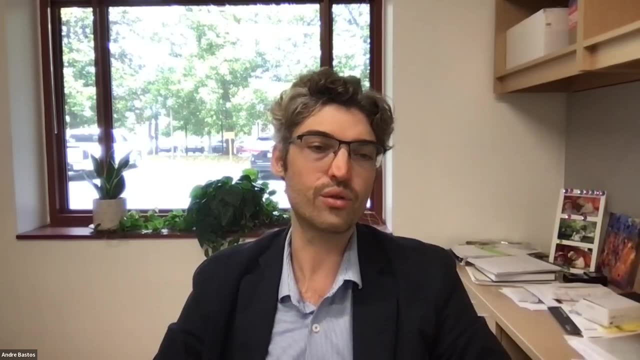 using these data sets. So that's really good for us. and then the next slide. So here we have a really interesting picture of the data set that we've been looking at, And we're going to give you a little bit of a sneak peek at some of the data that we've been 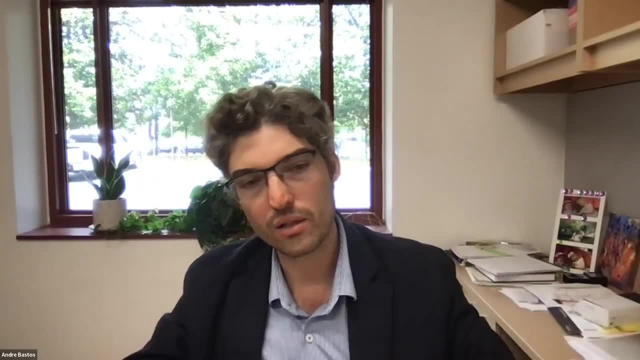 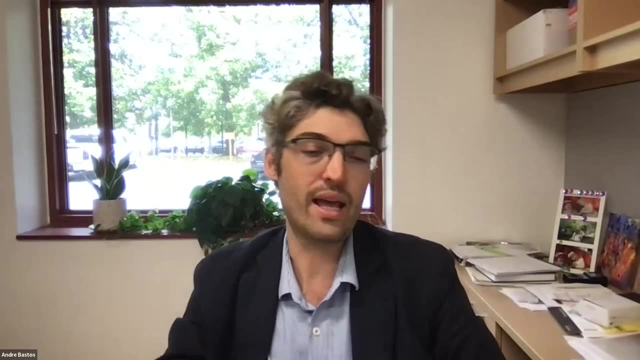 looking at, And then I'm going to give you a little bit of a quick overview of what's going on here, And then we're going to go ahead and quickly get into our second part, which is a little bit of a little bit of a walkthrough of what we're going to be doing with this data set. 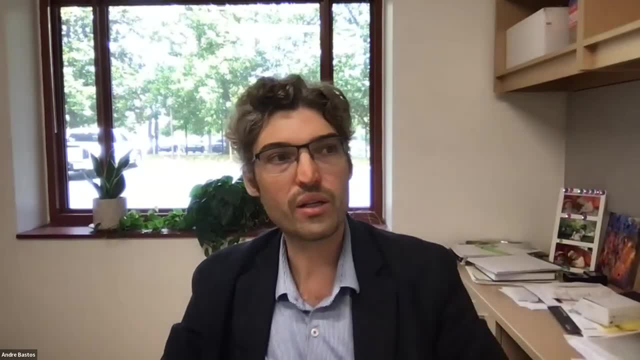 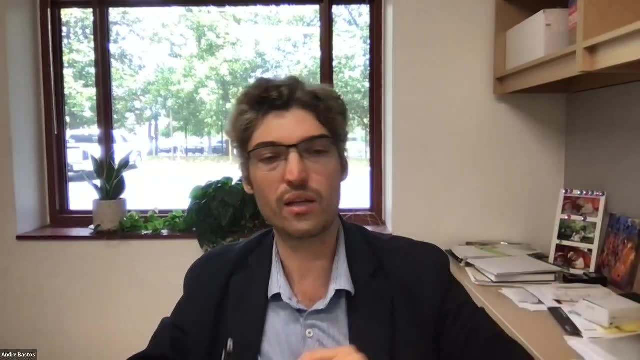 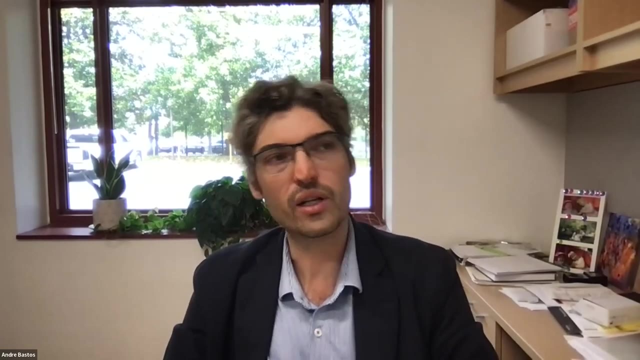 analyze Where we haven't made, in my own opinion, too much progress on in terms of working with machine learning is on asking the right questions or gaining mechanistic insights into the brain from again that naive approach to machine learning. But that being said, 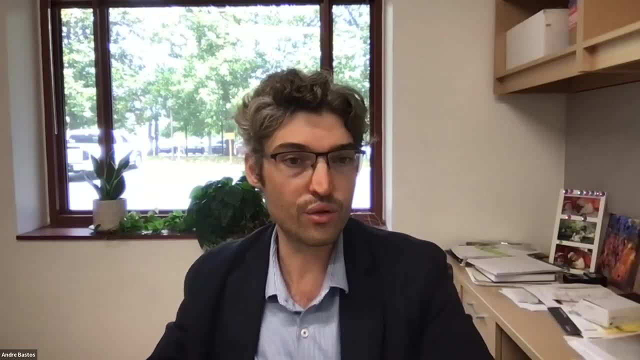 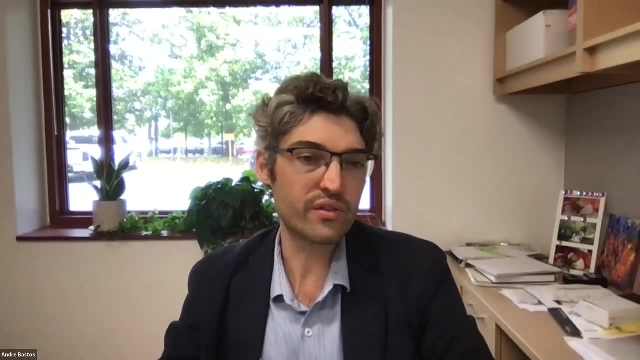 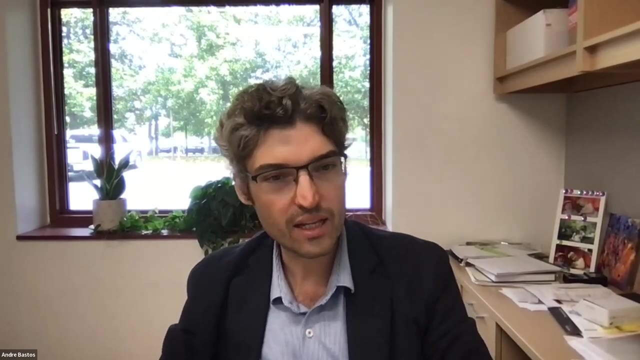 that naive approach is now enabling us to use massive data sets. So even that naive approach is, I would say, a transformative endeavor within neuroscience. So that's where we are now. Did that answer the question, Or was there another question tucked in? 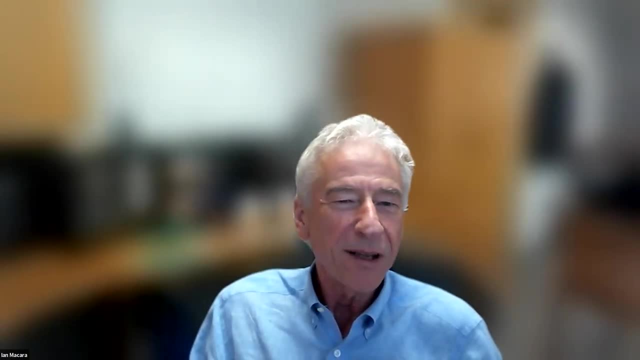 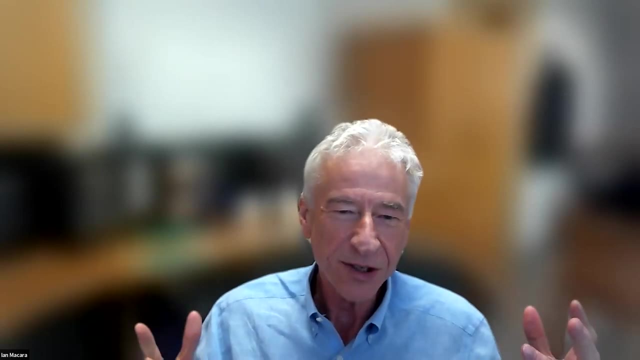 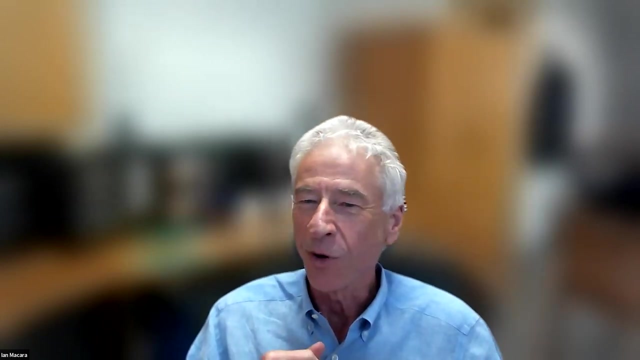 Yeah, no, I think that really does, But it makes me think- I mean listening to what you're saying- I wonder, in five years' time from now- I mean we already there's been huge advances in understanding neural circuits that control all sorts of behaviors. you know, hunger. 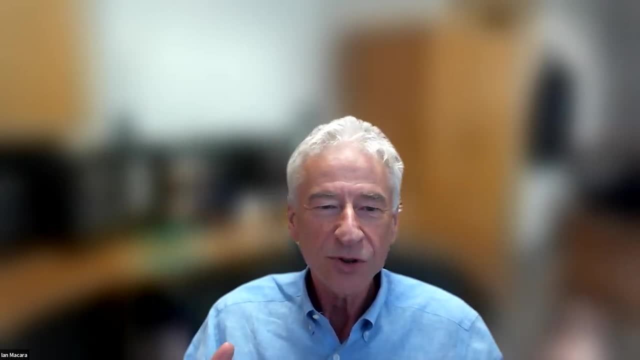 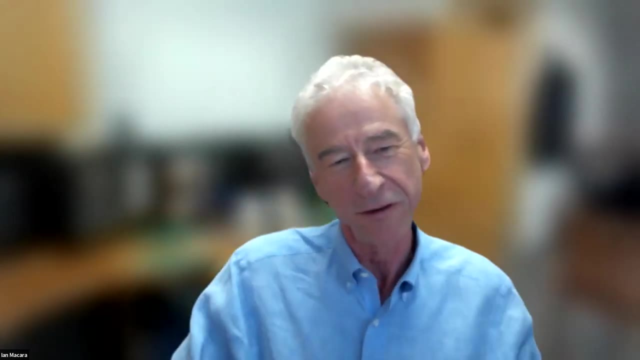 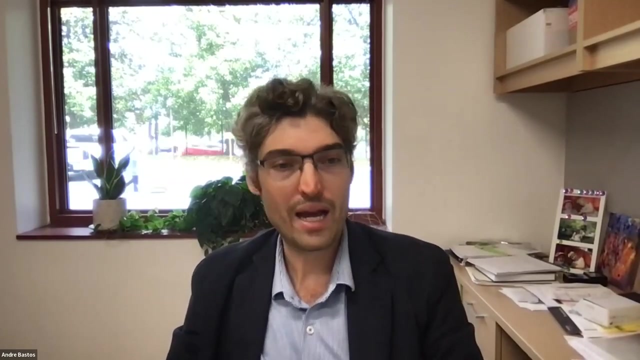 or whatever, And how that's going to change, say, five or 10 years from now, where, especially when you say there might be a thousandfold increase in the density of information that we can extract, Yeah, Yeah, then there will be an even larger machine learning or pattern. 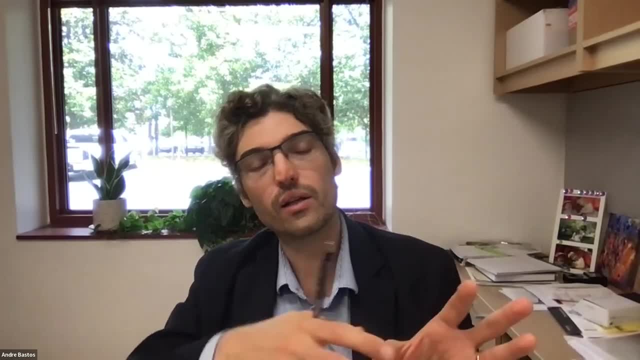 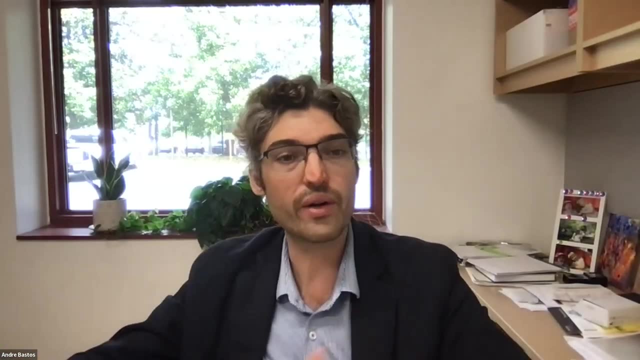 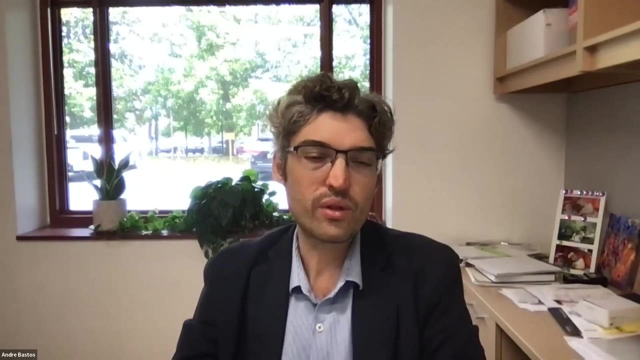 recognition problem. right, And that is not just recording and trying to figure out where the neurons are, but then trying to figure out how those properties of those neurons, those firing rate properties and action Potentials, the language of the brain, how that translates into thought. And that's really what. 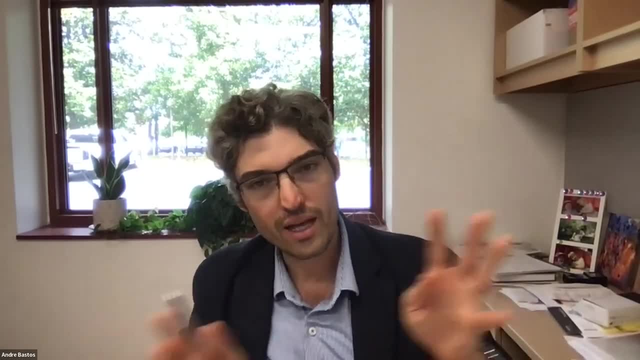 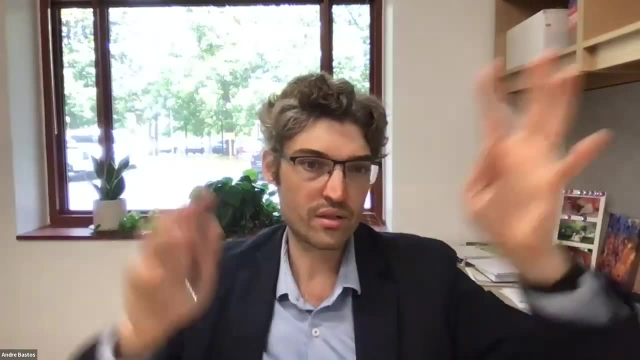 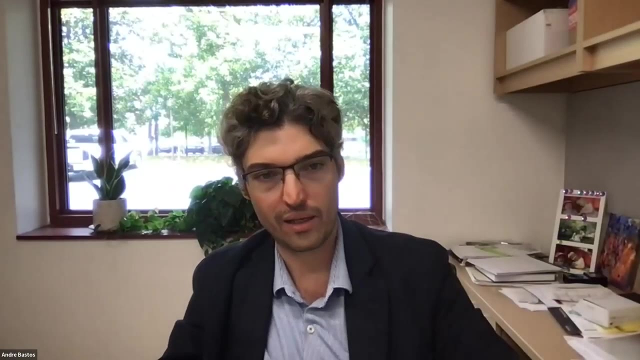 we are after And that's where I see that a current application of machine learning is perhaps going to give us the ability to categorize different types of cognition, but it won't give us a mechanistic insight again of how those things are happening. And there could be an argument to. 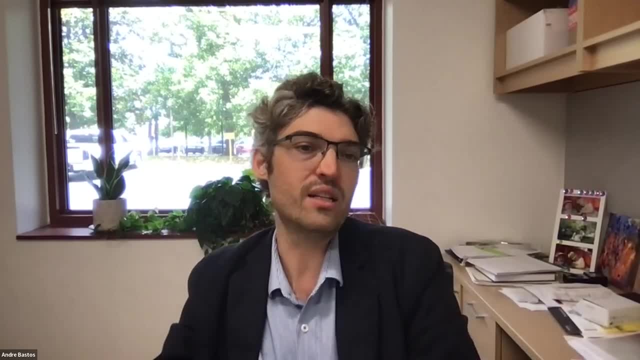 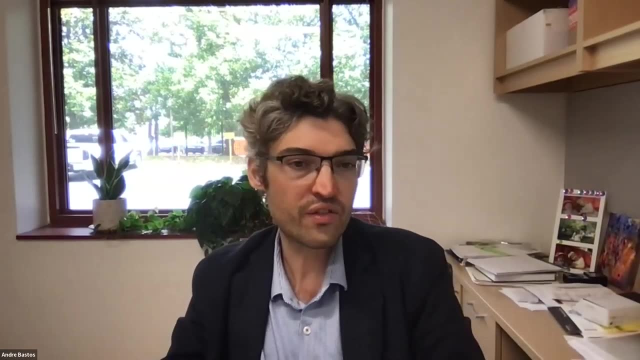 it to say: well, do we actually need a deep mechanistic understanding of how the language of the brain produces thought and action, Or is it sufficient to have a black box approach where we have the data, we have the trained models? that gives us? 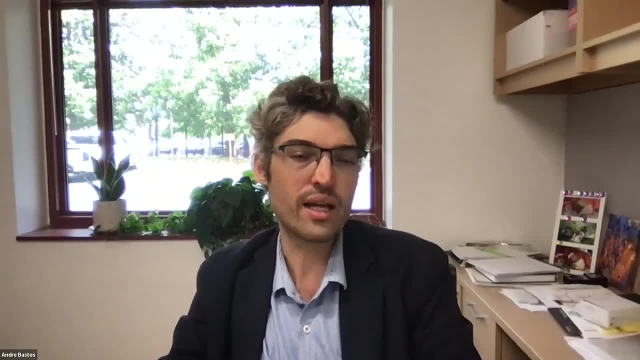 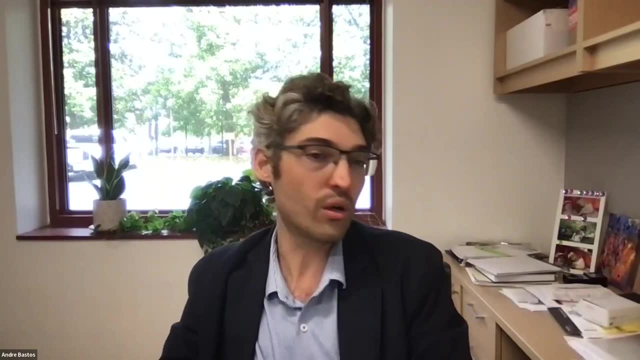 the outputs that we want. So that's one approach, that more bottom-up approach- To me as a neuroscientist I don't find that particularly satisfying, but there could be a whole host of good applications to that, For example treating brain disorders, if you can figure out how that. 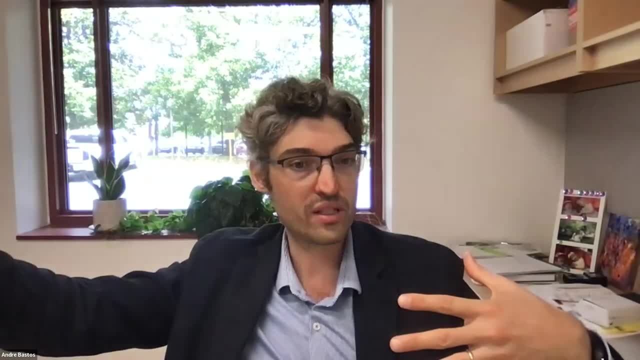 mapping between the brain and the brain is going to work, And I think that's a really good example of learning that over time, if you can do something that can go from neural language to deficits in a memory function, for example- works, you might be able to reverse it within this. 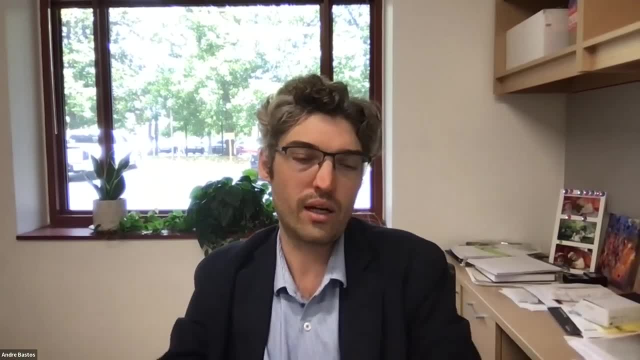 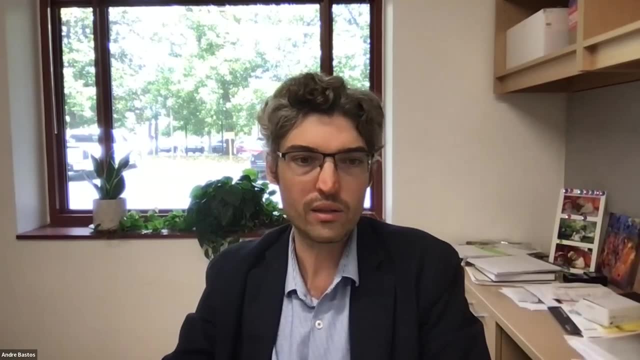 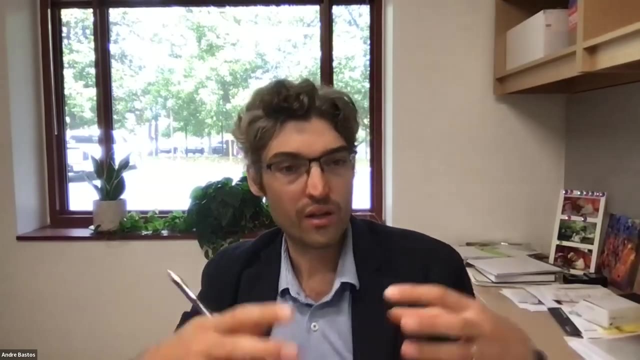 black box style engineering approach. I would hope, though, that we could move beyond that as well, in order to really be able to understand the how and the why questions. How are neural circuits functioning to give you these emergent properties of behavior, and why does that happen in 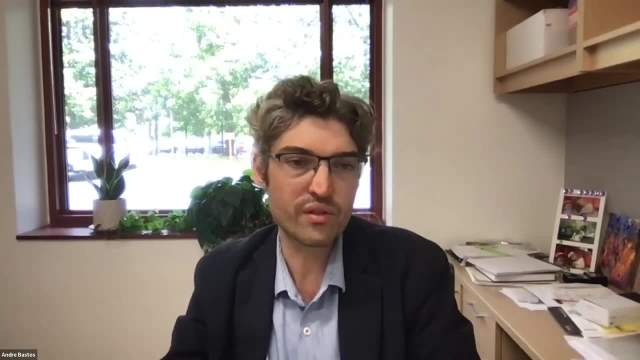 that particular environment, So there's a lot of capacity for that. that's something that's a great question I could ask. Yeah, I think that's a great question. I think that's a great question. Yeah, in a particular way and not in other ways, giving us other forms of cognition, for example. 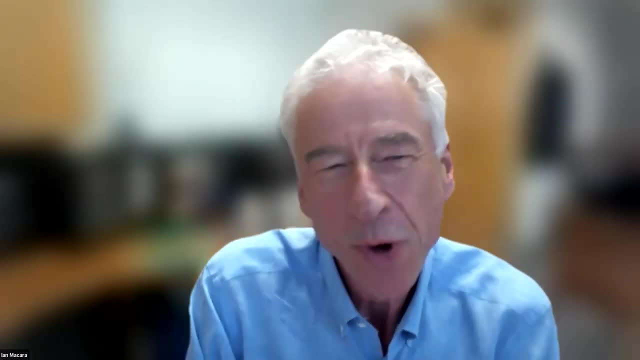 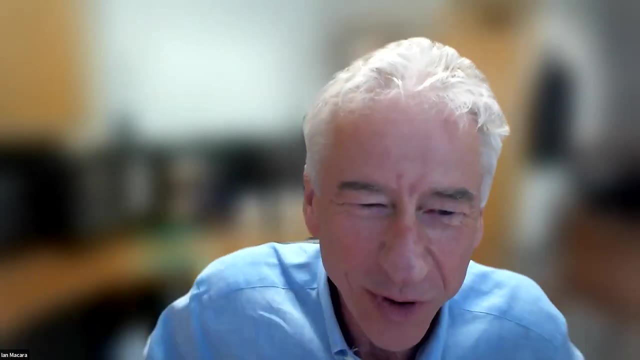 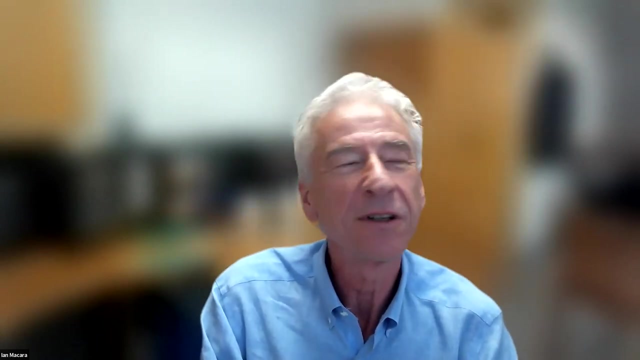 Jesse, do you think that, knowing that we were, we were already know the wiring diagram of the fruit fly And probably, you know, in 10 years time we'll know the total wiring diagram, maybe of a mouse brain? I'm wondering if this will have an impact on artificial intelligence and deep learning machines. 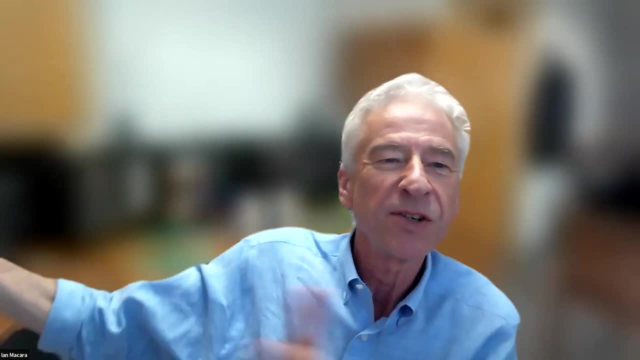 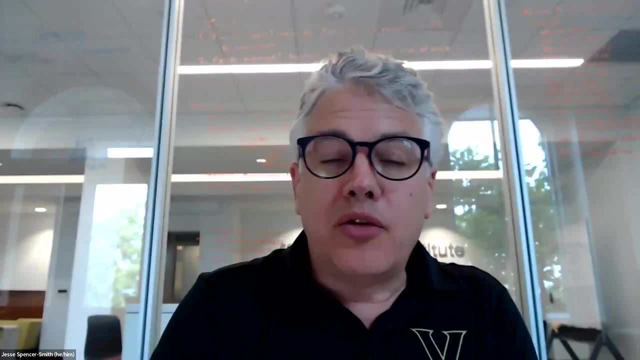 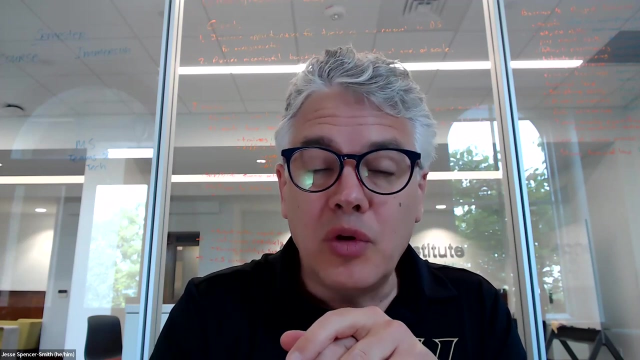 Is this or will it be a completely separate field? No, I think that right now, to train a deep neural net, a large deep neural net and a very large deep neural net, is extremely expensive. You know it. you know in terms of energy, in terms of costs. 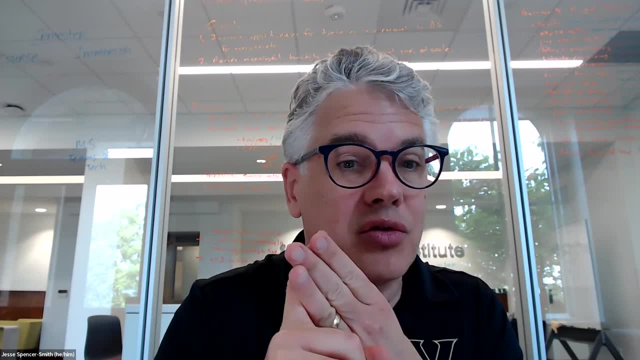 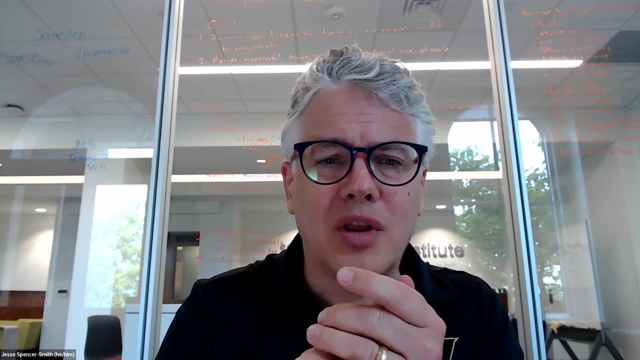 which means only a small amount of energy. But few select companies or organizations are able to do these, And that's because the way that that learning happens right now is is very compute, intensive in a process known as back propagation. This is- this is not biologically motivated. 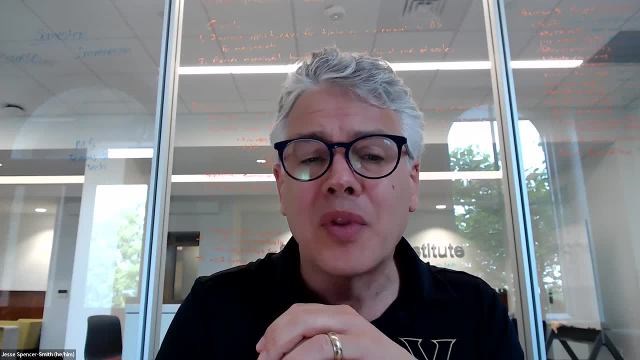 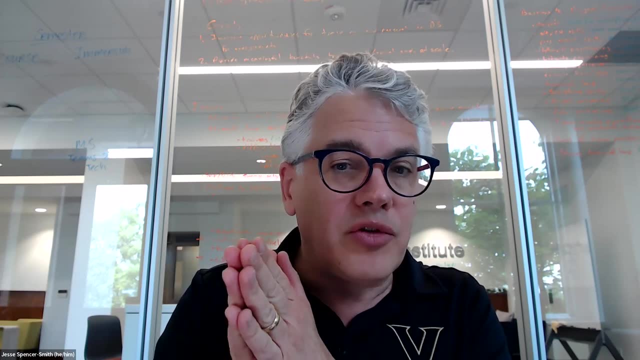 You know this is a brute force way of doing it. So if we did understand how the biological systems worked, then I think there would be another huge advancement in the training of these deep neural nets. So Vishnu just said Just on: the questions was asking: why do we need the larger models? Why not just train smaller ones? You get larger emergent capabilities as you go to larger and larger models. They're able to do reasoning. They're able to solve different types of problems, like logic problems They can solve once they get large enough. 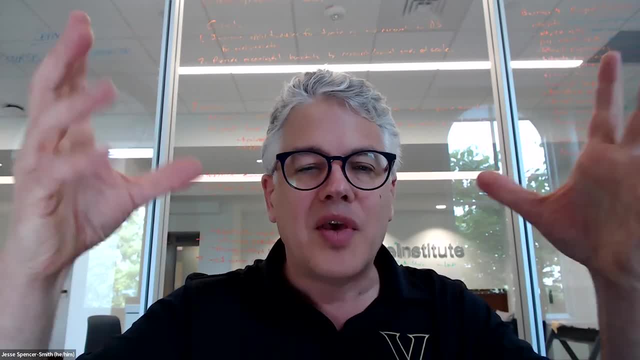 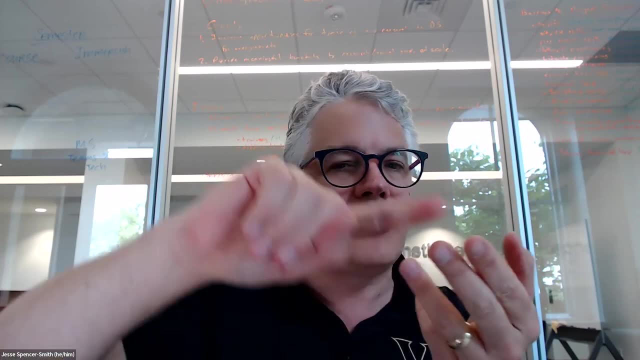 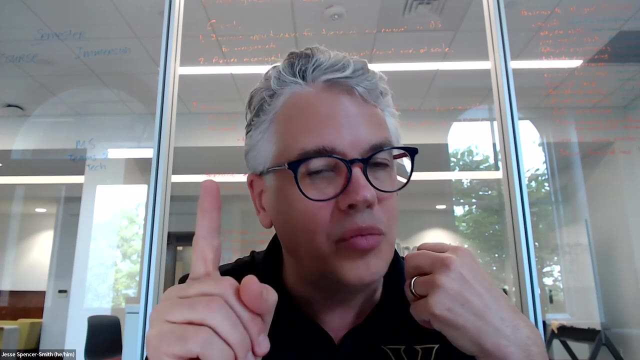 They can solve very different types of tasks, And it's the same model solving many, many different tasks: Visual puzzles, categorization, audio- all in the same model, kind of like we would expect a human to be able to do- Not human performance but human level. 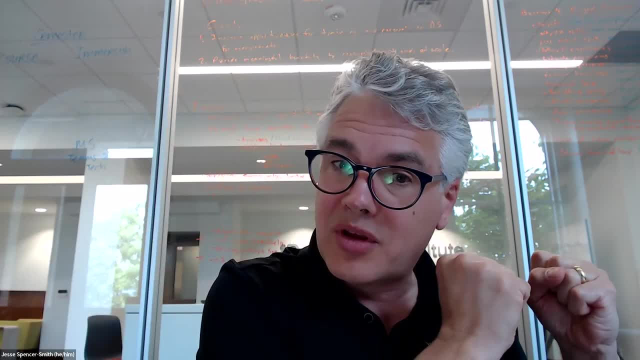 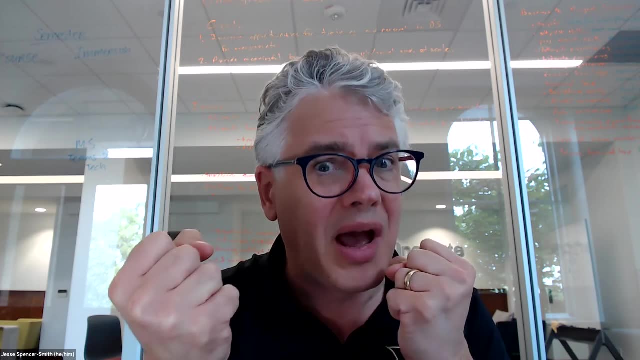 performance, meaning you can perform as well as even you do something completely different. But in order to do this, you have to power a small city for days, weeks or even months- the equivalent power to be able to do that. So, getting more out of the training, getting more. 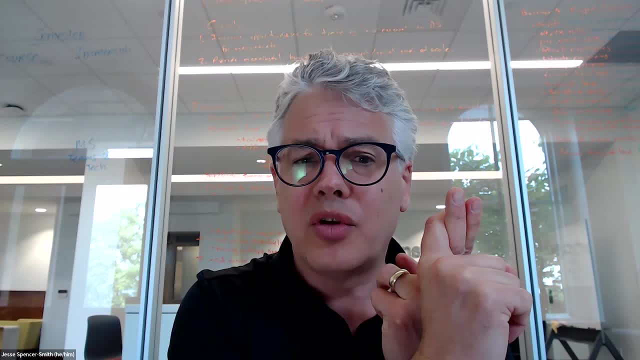 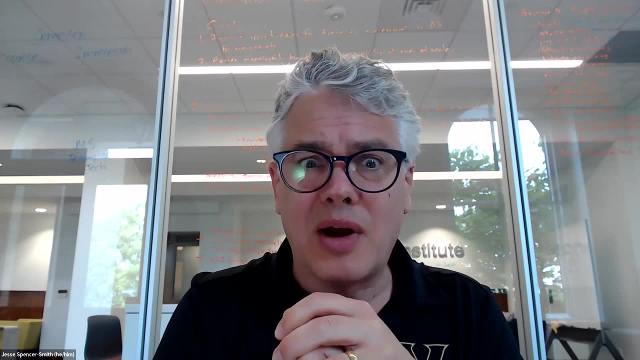 out of smaller models. We know that a great deal is possible now once we go to more and more powerful models, but we've got to get better at training them so we don't have to impact, frankly, the environment so much as we're training these models. Yes, I always think we're very proud of 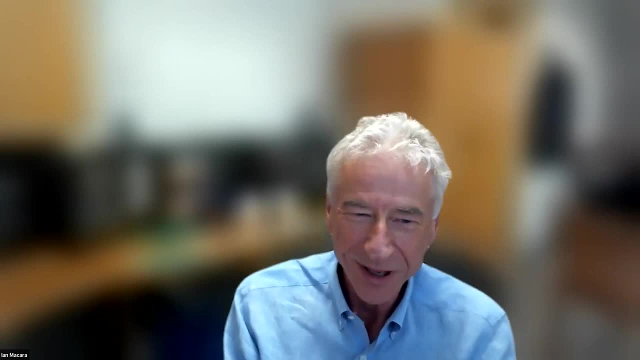 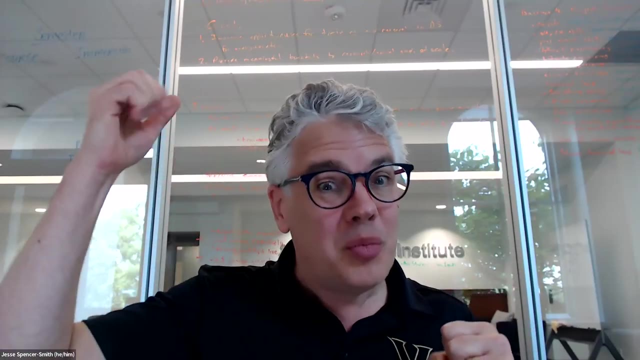 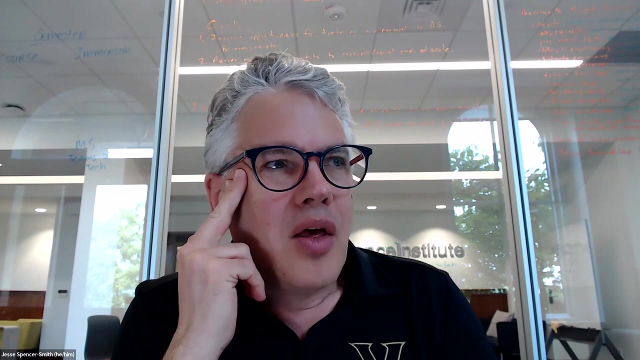 our technology. but then I look at a living organism and I think, wow, we have a long way to go If you compare the number of free parameters that a human has- and here I'm not on a log scale here- that a human has versus what the machines have. Now, that being said, the number of neurons, 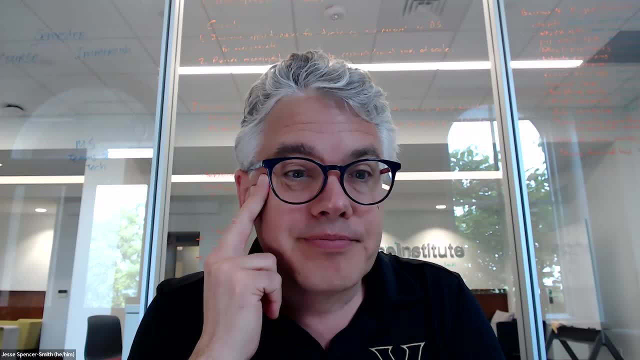 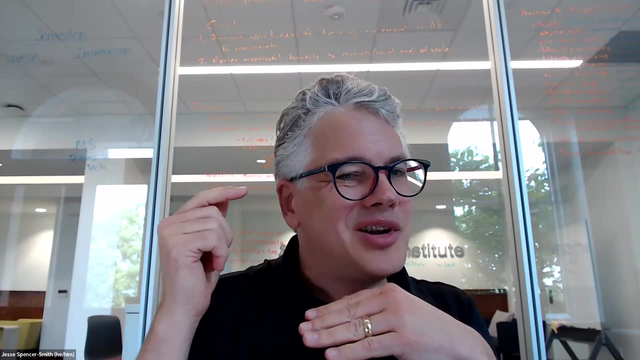 that you have in a frog. the number of neurons in the brain do a really good job of driving a car. It's no longer good at being a frog, but it's very good at driving a car, So you have a lot of capabilities. You don't have consciousness. 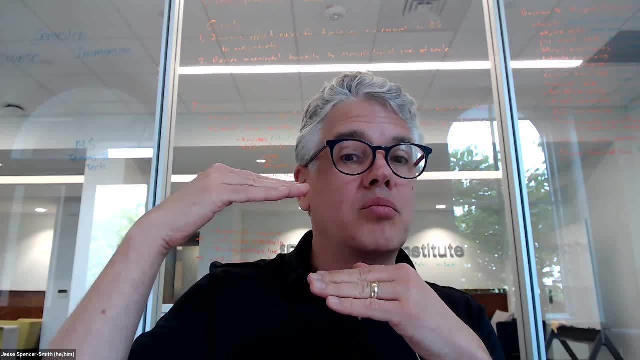 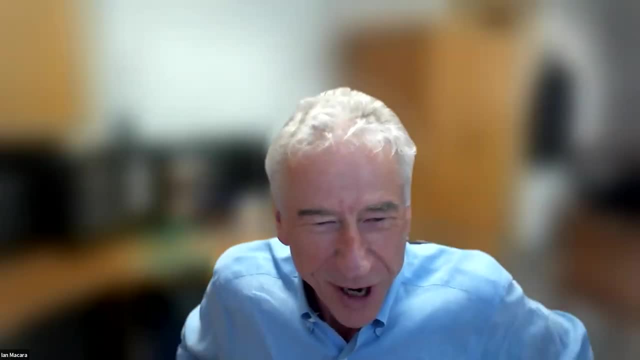 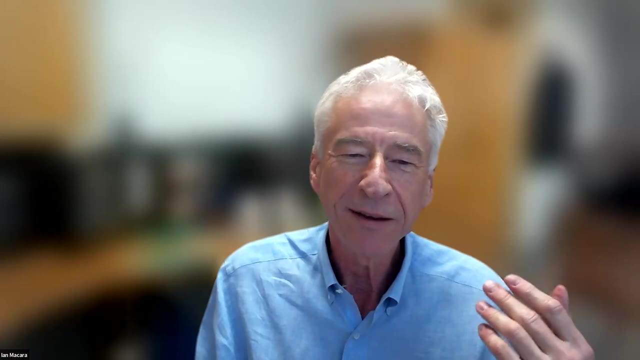 you don't have self-awareness, but you have the ability to solve problems creatively. Yeah, I often wonder. we talked about this yesterday. when I'm driving my Tesla and I'm looking at the screen and I get the sense that it's perceiving the world in a way sort of like a frog, right? 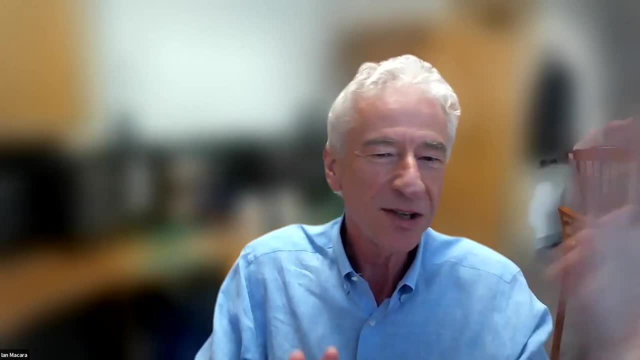 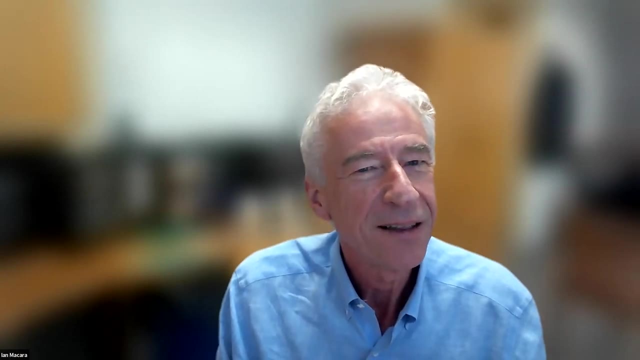 It's perceiving, it's not taking a photograph. it doesn't see the trees or the buildings. it sees a stop sign, it sees traffic lights. you know, That's right, And that seems to me it's perception, it's cognition. that's not that different from the way. 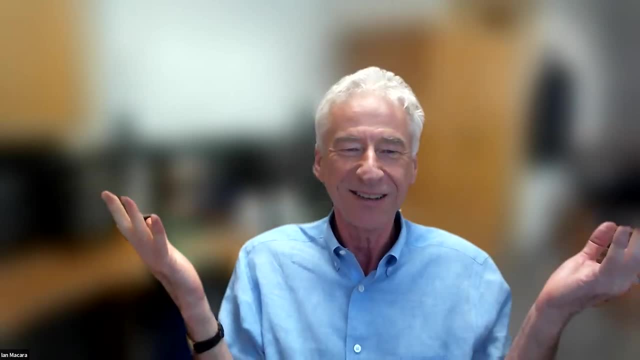 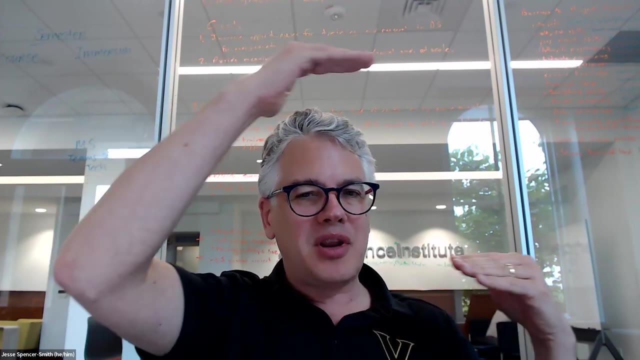 an animal would perceive things. I mean, it's a semantic layer, right? So you're immediately jumping to the meaning and the capabilities and what's happening, rather than: oh, here's the tree, here's the tree, here's the tree, You're just gone. 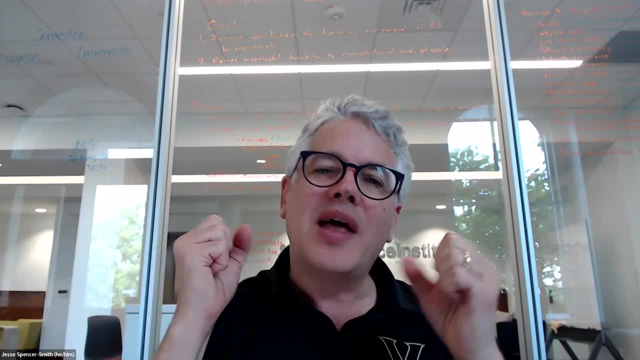 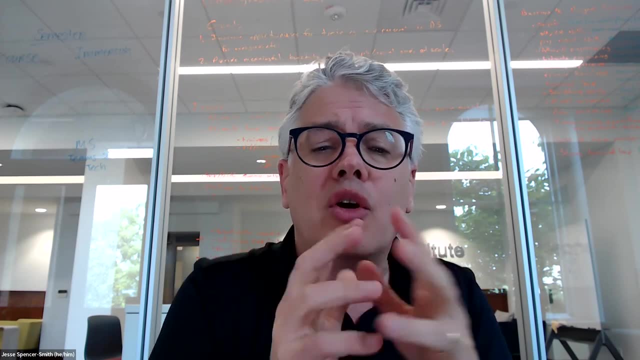 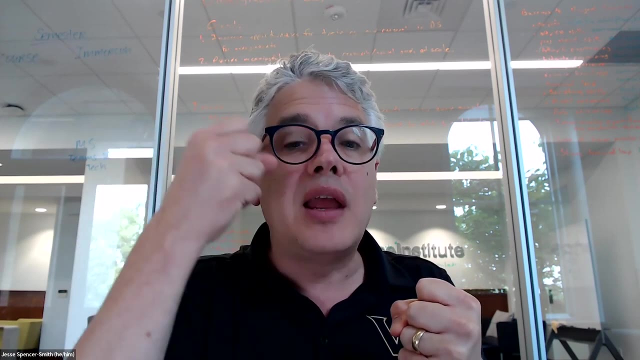 is a group of pixels, very quickly go up to this level. that's what's so different and what's changed in the last just even two years. uh, that these models are are able to to pull out meaning and create representations and learn the language of whatever you're showing it, learning the. 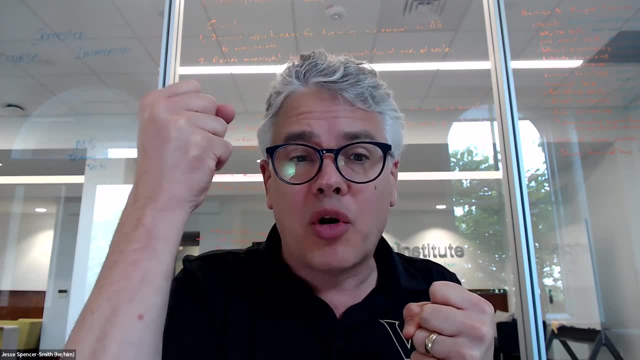 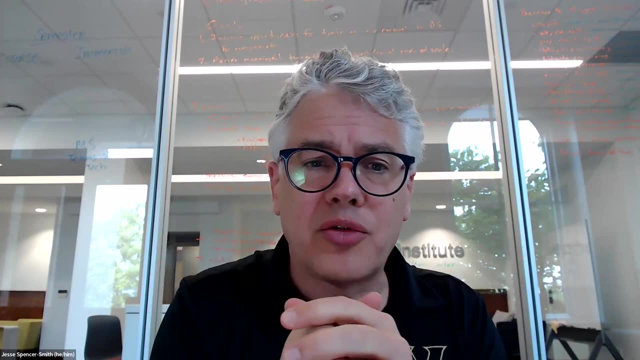 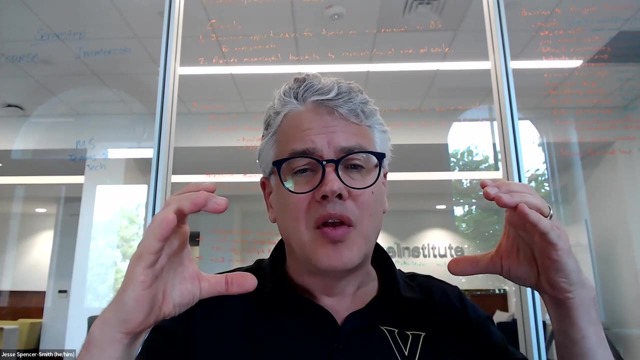 language. you know, like we, like shannon was just saying last summer- learning the language of proteins by seeing, and being exposed to and doing self-supervised learning. transformers are the name of the deep learning models that have these general purpose learning capabilities. these models have multiple capabilities, so they're trained on one thing, but they can be used for. 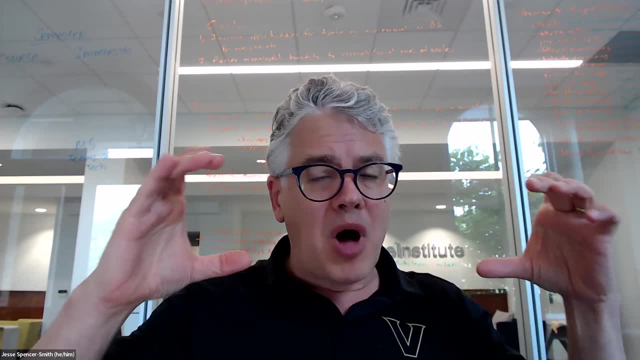 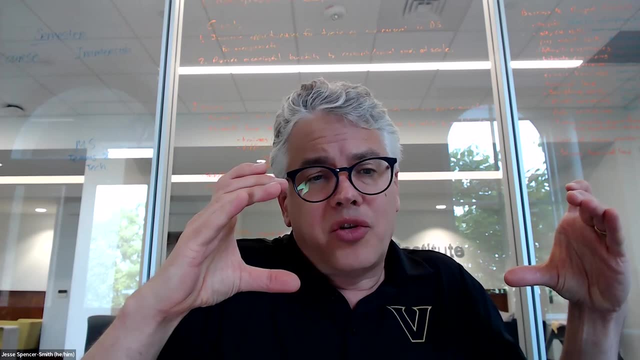 many others. so with tesla, for example, they have a single model underneath and all these other what are called model heads on top. so this knowledge of the world and what you actually see and what you get out of the different sensors one is designed to figure out. stop, stop signs, stop lights. 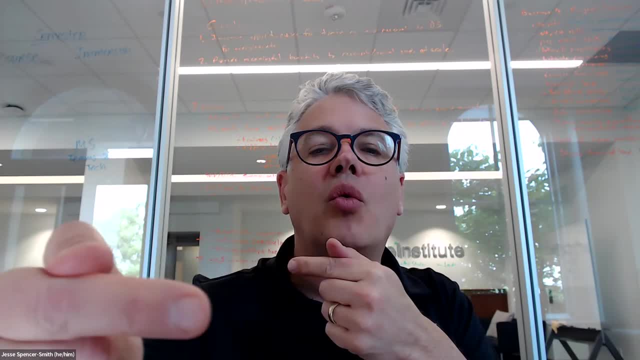 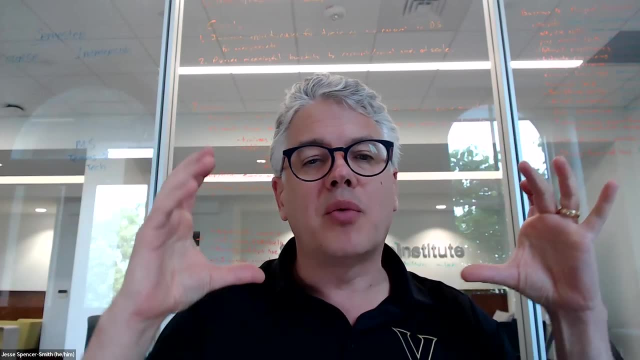 another one is designed to turn out to figure out how far you are from the car in front of you, from vision alone. they don't use radar anymore, right? so all these different capabilities built on this pre-trained model. that's why these models are now called ai foundational models. you don't 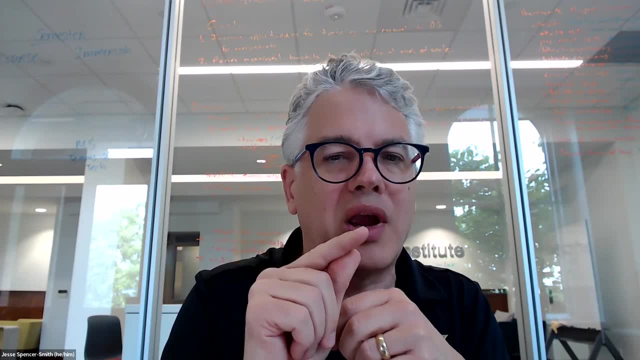 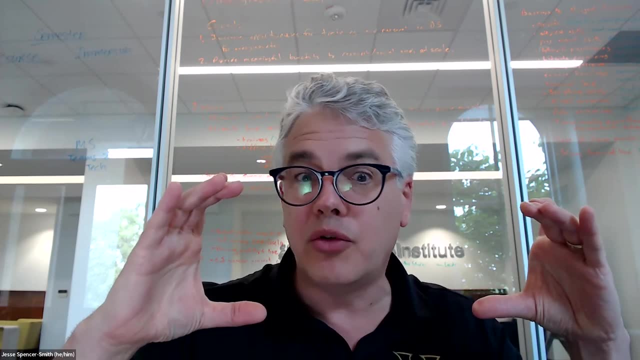 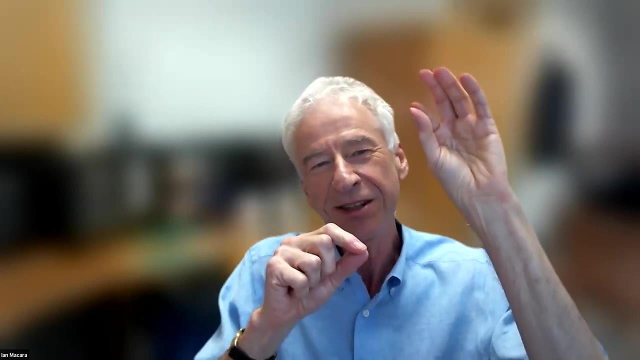 just solve one problem, train and solve one problem. instead you train and train and get trained on another problem and these models are growing and learning and getting more and more capable, as you do that, andre, do you think i mean this cognition idea? there's any similarities conceptually in the 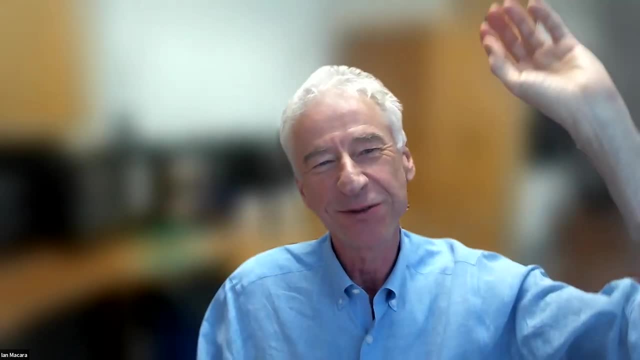 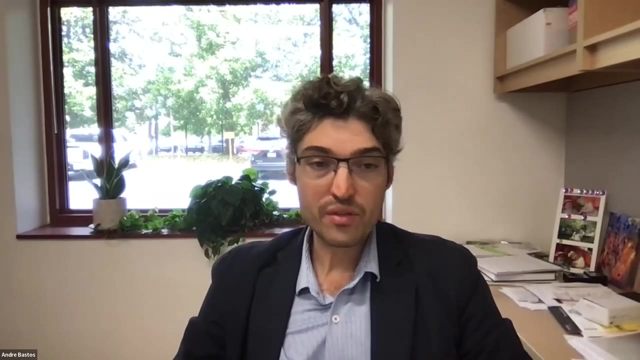 way, you know, a car perceives the surroundings versus the way a primate does. i i don't think at the level of cognition there's there's a lot of similarity. i have to be honest, though i don't- i don't know exactly the- uh, the inner workings of those representations, but, um, in the primate brain, 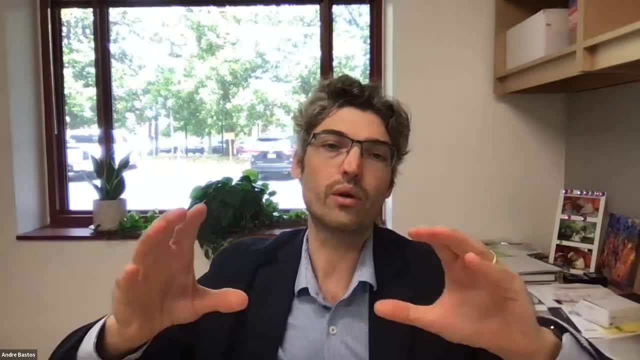 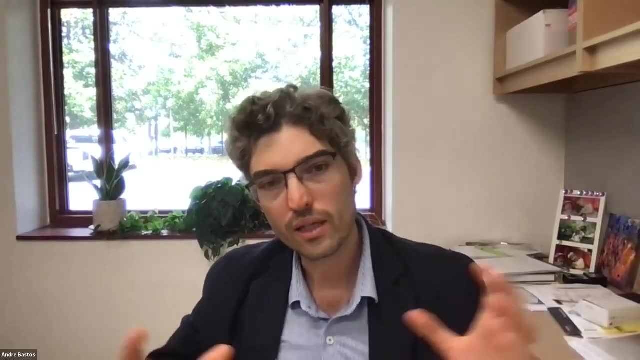 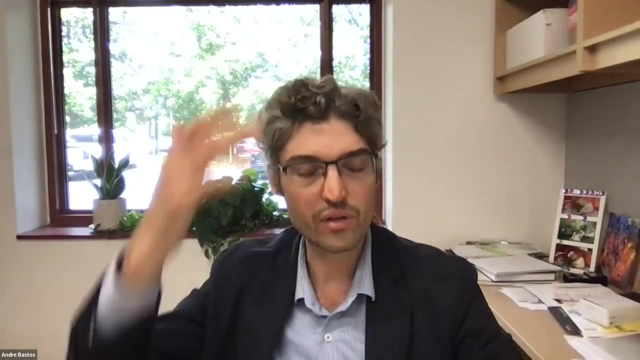 um, the way it sort of works is you have these deep neural networks um that um basically process, let's say, vision or touch or audition. but then, as you get up to the more cognitive areas of the brain, the prefrontal cortex for example, uh, right, right here in, uh, in the back of your, of your forehead, you get to a type of representation. 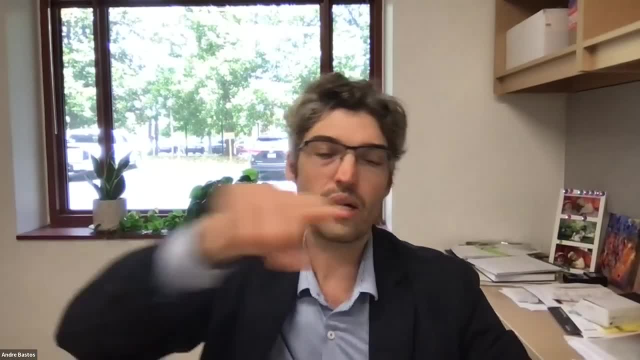 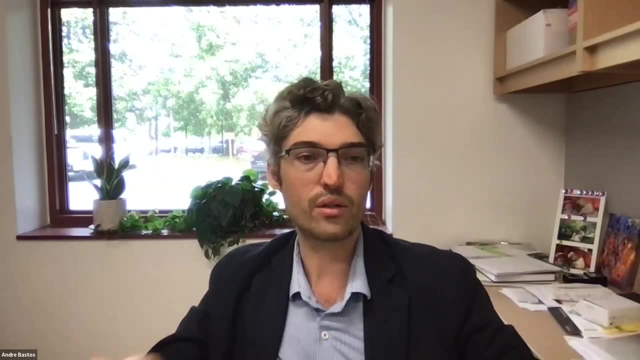 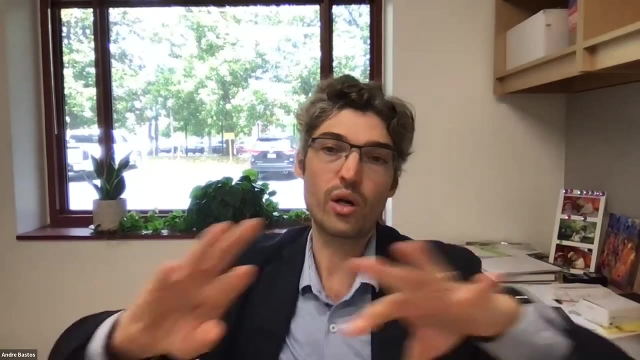 that's no longer so strictly hierarchical and it's more, uh, akin to a, um, a random network which can then be trained. so you, and there are certainly parallels for both of those things- um, within machine learning, uh, maybe it's a. it's a question for jesse whether or not that same architecture. 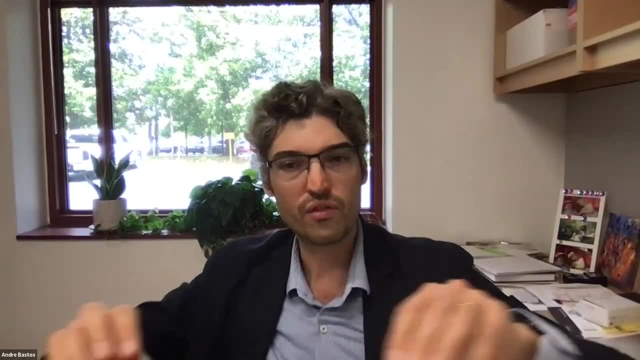 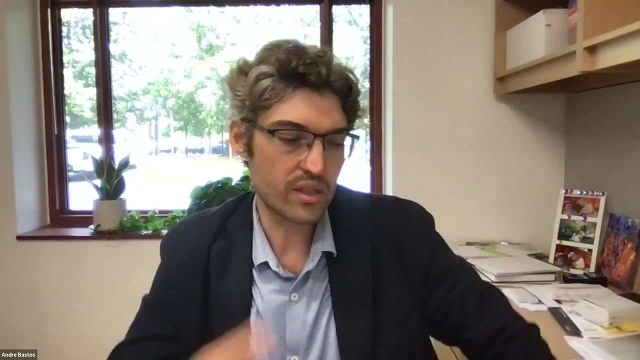 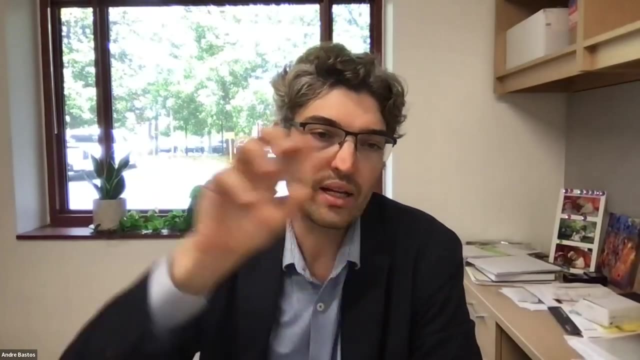 um exists, um a deep neural network feeding into a artificial neural network and then feeding back down and the. the idea currently is that consciousness is an emergent feature of having those two elements in the model, this deep hierarchical network as well as a recurrent uh level, and that, in order to be conscious of 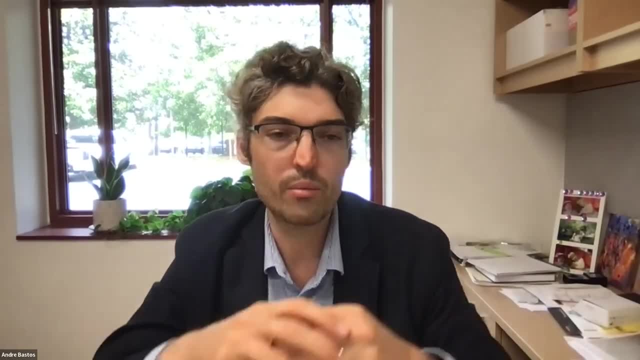 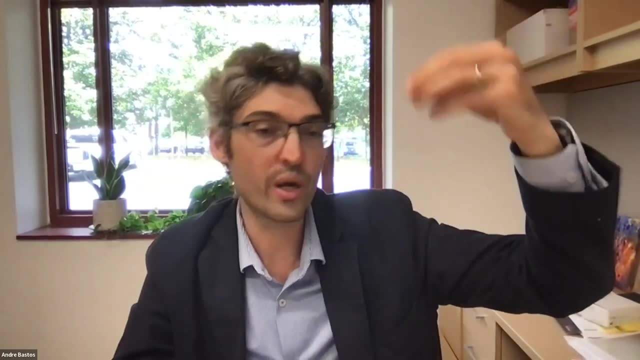 something you actually need, what we call um a broadcast of a signal throughout the entire networks. it's not sufficient for just the top level of the of the brain, for example, to think about a face. if that happens, you wouldn't have a conscious percept. but when you consciously 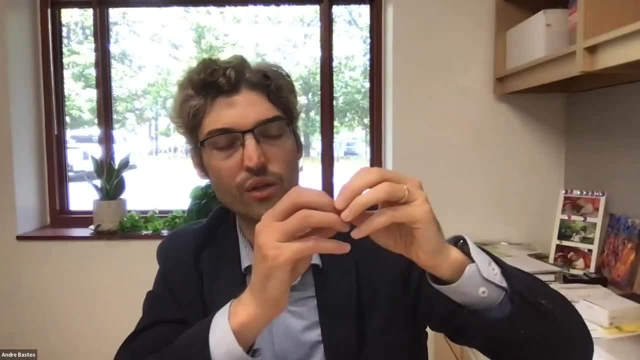 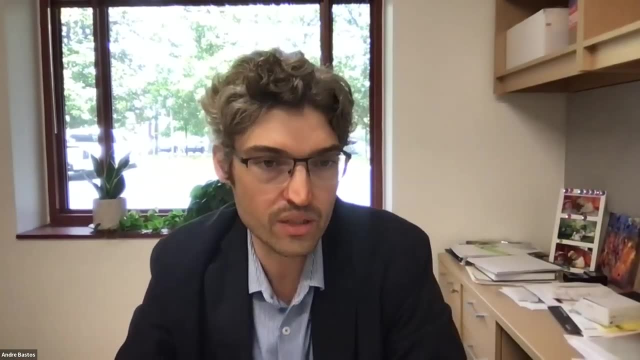 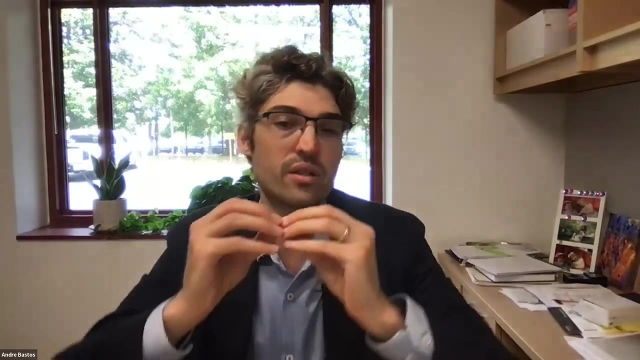 perceive a face, you hit that top level. but then you have this global neuronal broadcast of that information throughout the network. and that sort of level of organization isn't present in um, in machine learning networks as far as i know, the sort of idea that it's not sufficient to just represent but really to globally broadcast that representation. 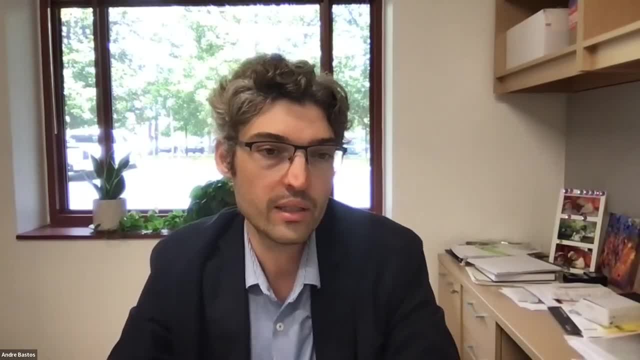 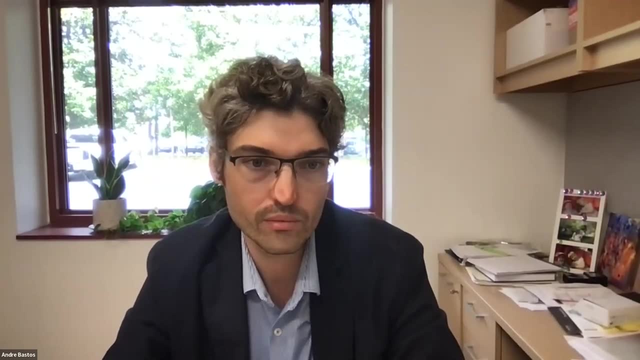 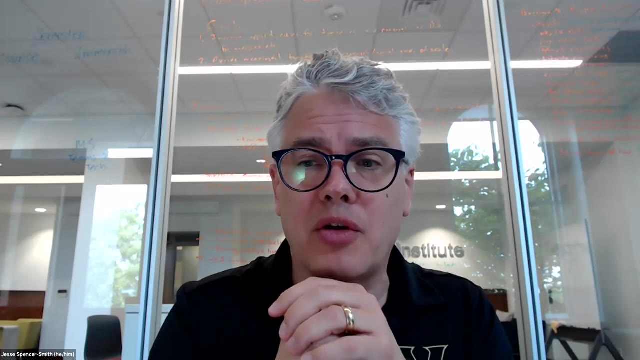 so that's, it's available to a large part of the network. that's currently one of the leading uh theories of how you become conscious of a particular percept, and i'll just mention again real quickly: i, how surprised i was. so, as a cognitive psychologist, i was quite surprised with the capabilities that that are possible without without that, so without 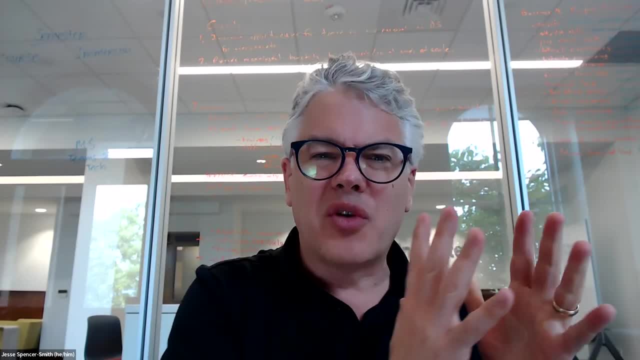 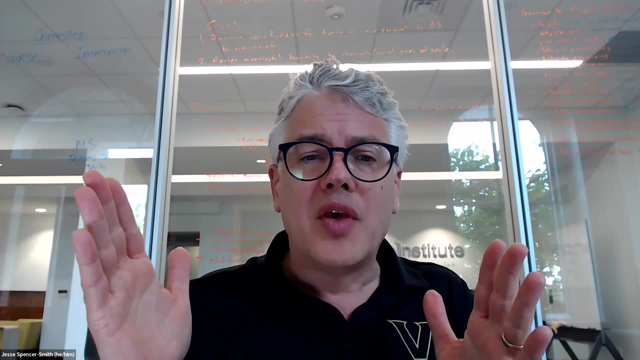 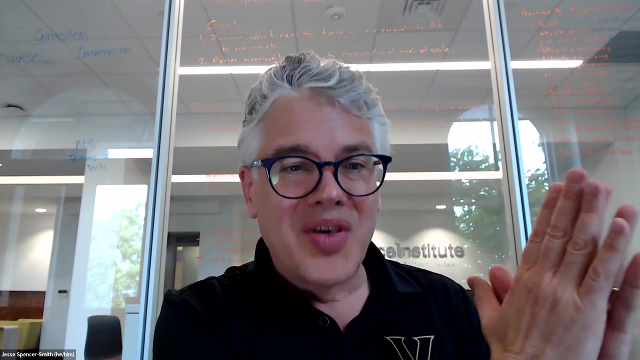 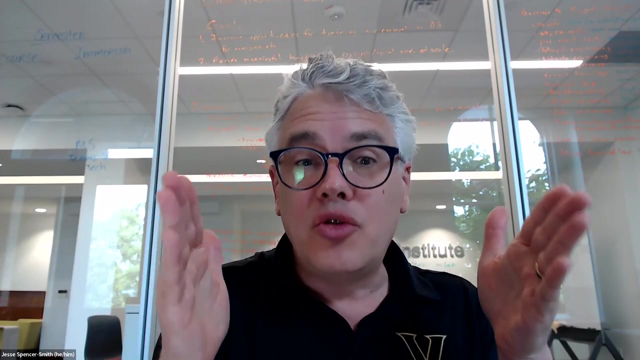 that even the, the ability to, to develop awareness, this very, as i mentioned before, like crystalline kind of representation of the knowledge, very sophisticated representations of the knowledge, but it only some recurrence within, but these are just within stacks. generally it is feed forward, you know, only going forward, and yet amazing representation. so, my goodness, when you actually do introduce you. 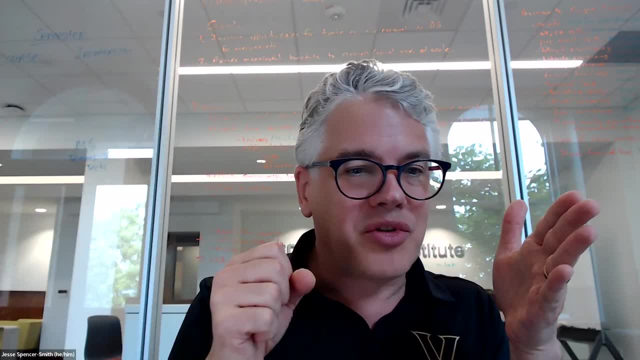 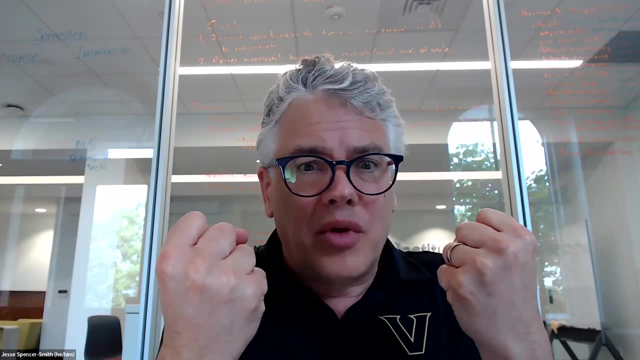 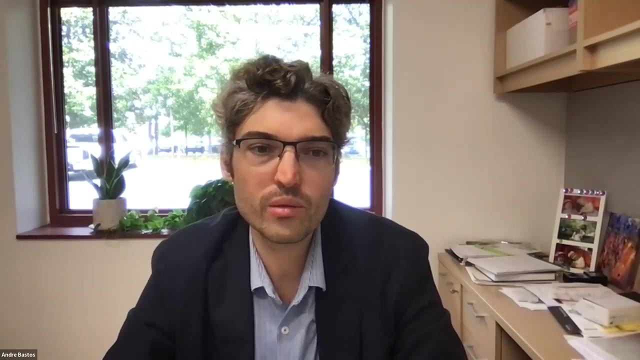 know the architecture which does support. you know that, as you're saying, andre, that the broadcast what? in my mind, it's kind of like you have the foundation of knowledge there, right, and weirdly we have that first. yeah, then everything else is going to come after. well, let's talk a little bit more than about this difference between feed forward and feedback. 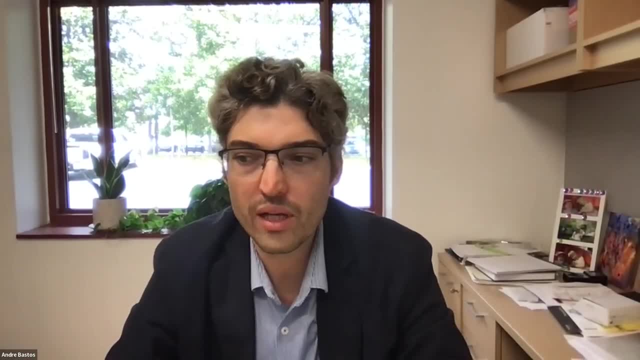 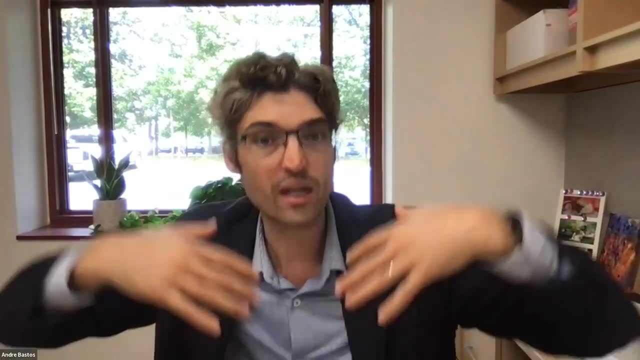 because i think it's a, it's an important distinction there. um, as a neuroscientist again, we have, we have this idea that you know you have your sensory data, it comes in and it feeds up the cortical hierarchy, but then we know that already at an anatomical level we have just as many and 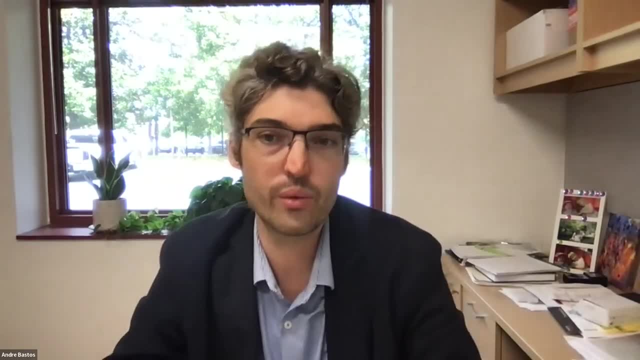 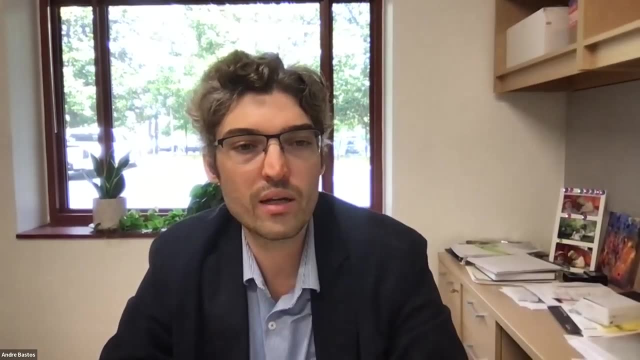 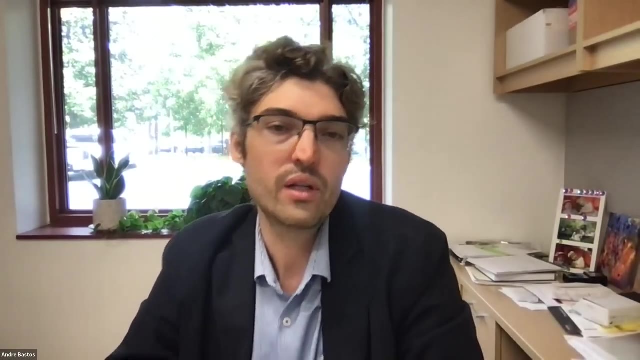 in some systems, more feedback connections coming the other way around. and these feedback connections, we're still studying their physiology and their function. we don't have a perfect understanding of them yet in relation to the feed forward, but in general, the idea is that they are capable of transforming and performing. 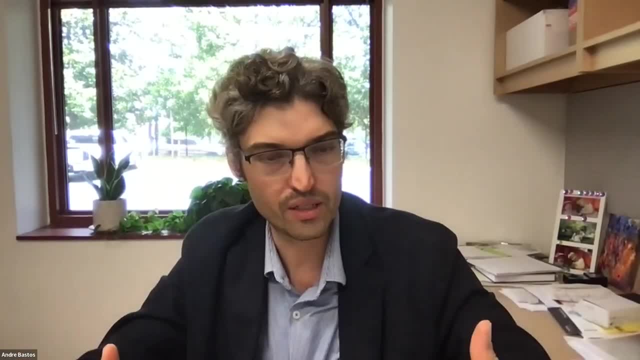 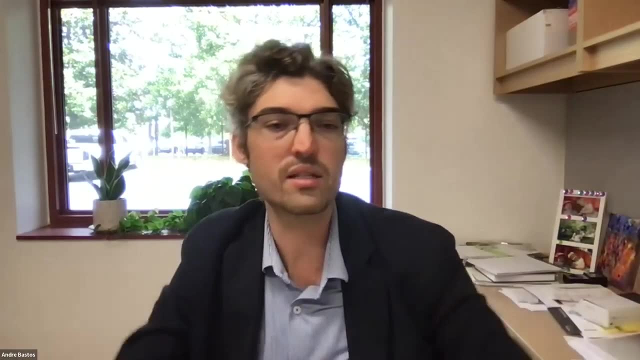 manipulations on top of those first order representations. so, for example, you might represent a car and a tree and a face, but then the feedback processing is necessary for you to decide which one is important at that particular moment in time for you to, for you to pay attention. 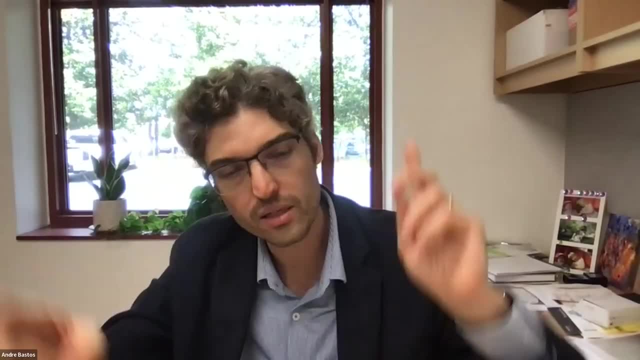 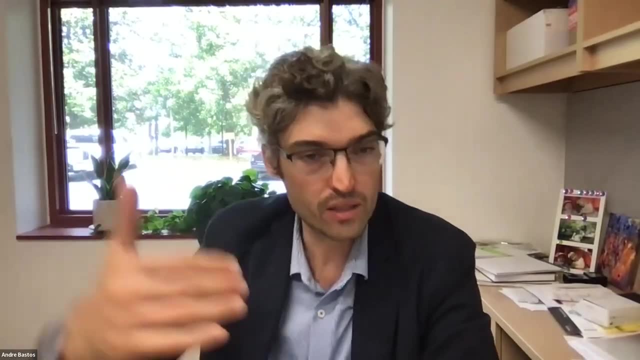 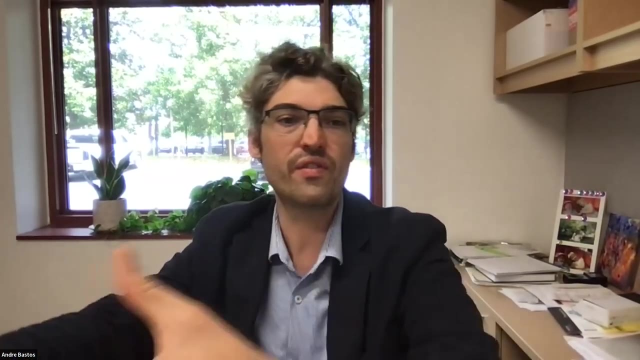 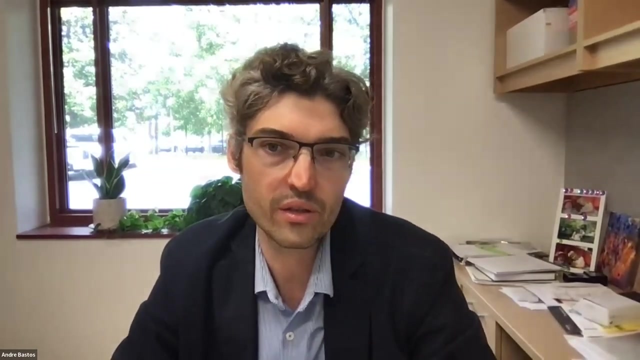 to the idea is that there's always this constant interaction between these feed forward and these feedback loops and, um, whereas the feed forward, uh sort of architecture has been influential in ai in terms of building networks that look like that, so far the feedback information from neuroscience and about the brain hasn't informed too much, although i know that there are certain developments. 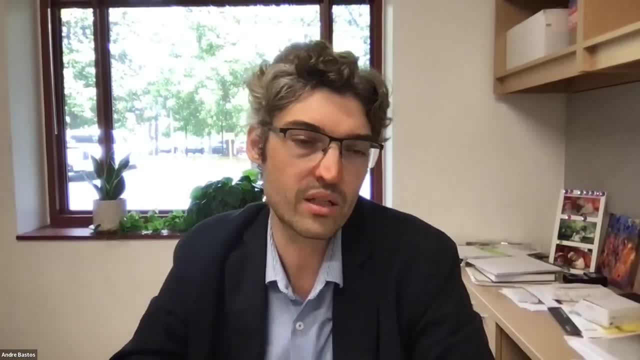 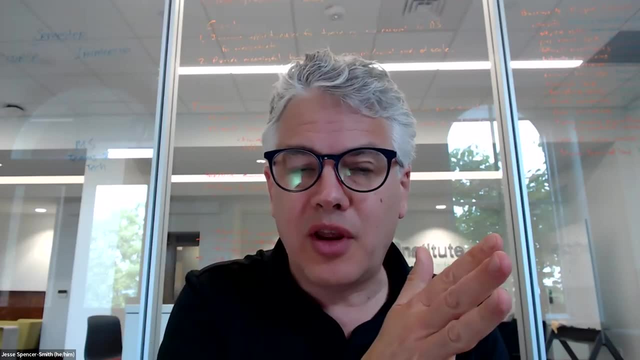 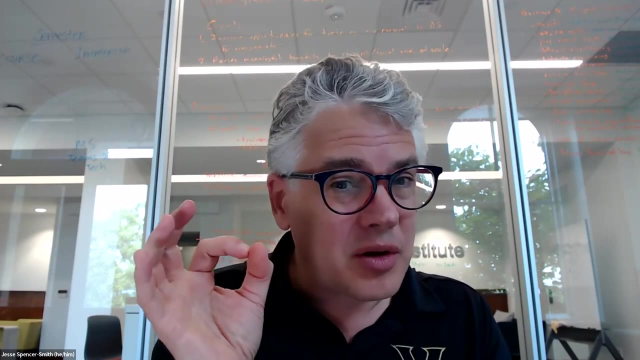 but hasn't informed too much. the training and the learning and the basic structure of these ai models. i would say the what's, what's informed. uh, in the last, in 2019, when transformers were were broadly, more broadly introduced was the idea of attention. um, but done in, done in a very particular way. i. 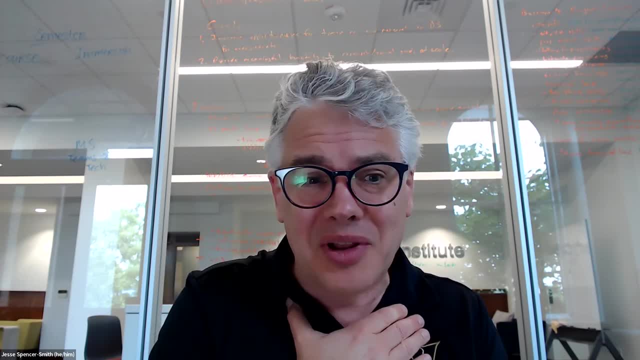 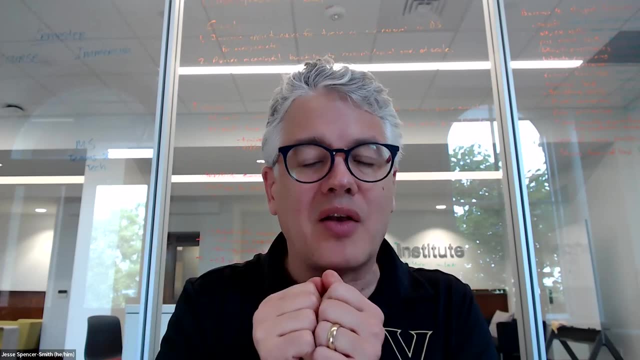 don't know if i personally would have called it attention, but it certainly seems to be acting like that. um, but, but you know, in a very particular way and and the feedback only happening, you know, within particular parts of the stack, the one big feedback that you have that goes all the way back. 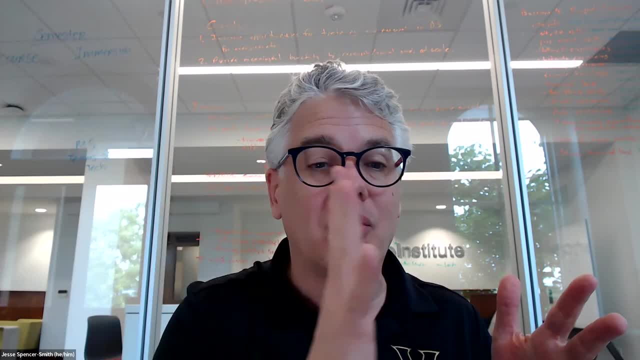 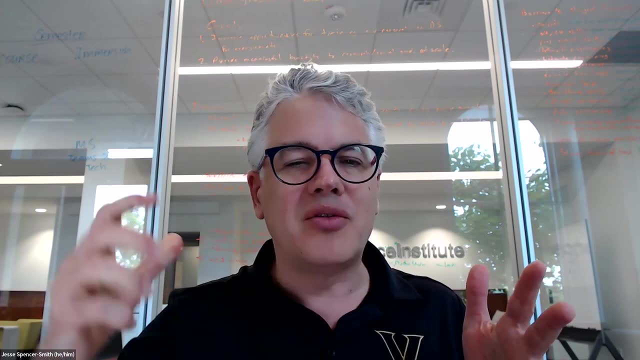 across the network is the feedback that you get from the stack. and the feedback that you get from the stack is that back propagation, which is only happening during learning, and so the, the changing of weights, the learning only happens during training, you know very expensive and that, if you want to think of. 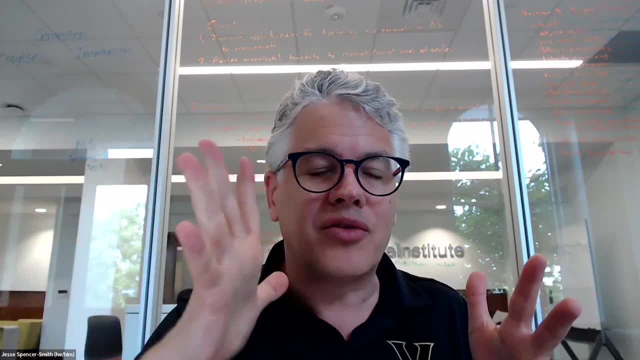 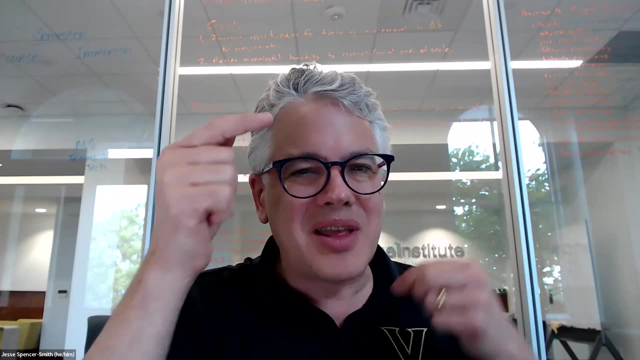 like a broadcast message. message affects every, all the way. it's all at once, like the entire brain being updated, the entire network being updated. that's not biological. you know where we have, like you know, selected uh, feedback and that's what's missing now. granted, even with that, again, we do. 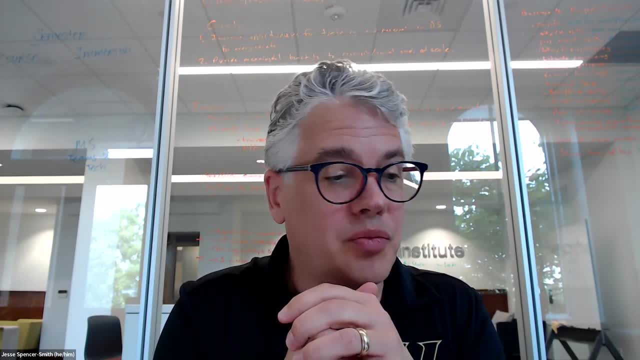 have these, these uh capabilities that we can use to do that. so i think that's a very important, really important thing to keep in mind as we're thinking about any of these uh capabilities- uh, uh, that that are pretty astounding, right, right, okay, i think we should probably switch to some of the 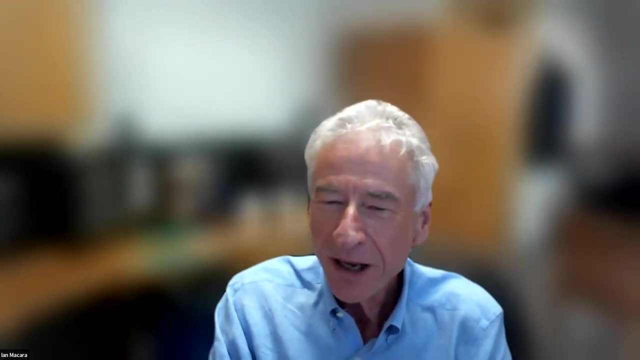 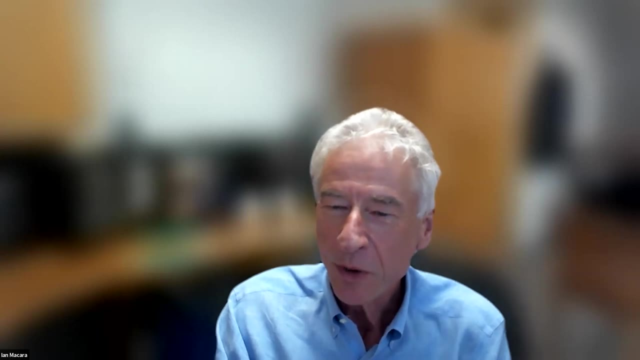 questions that are popping up on the q a here, and maybe, maybe i could ask shannon to respond to this. somebody's asking what can ai predict what will happen when a potential medicine is used to treat a patient and how the compound will act in in the body? and i mean, i would guess at the moment that's. 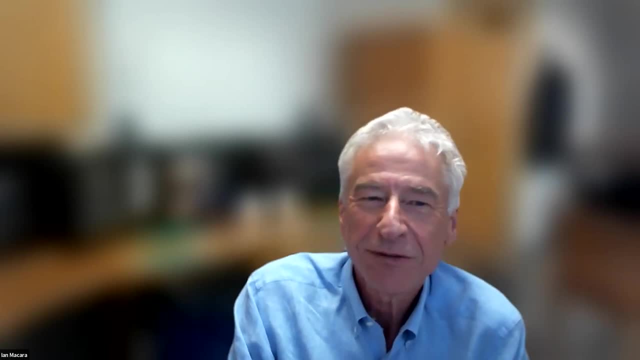 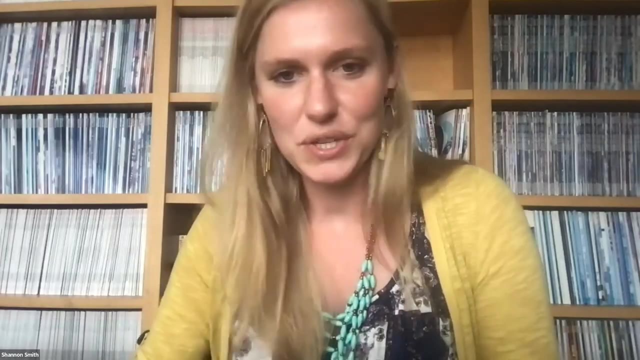 a little far off, but if we think about the different, uh, the different abilities and the different, um, far-fetched. but how do you see it? say, you know, five years from now, you see this, yeah, i, i love this question. um, so that's one of. i would say that's probably the area of biggest focus for 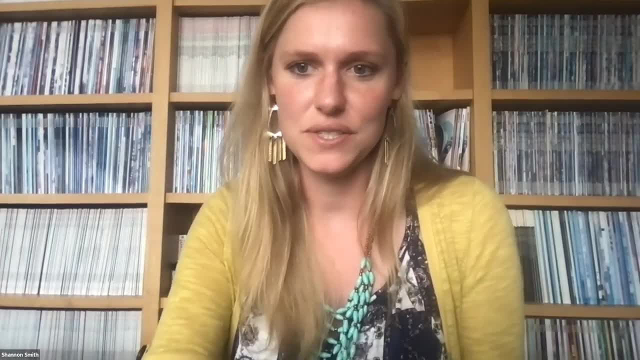 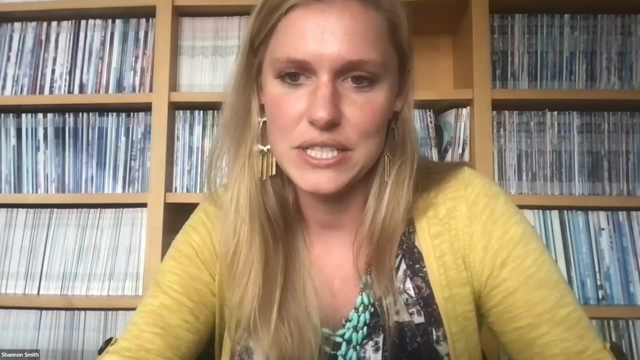 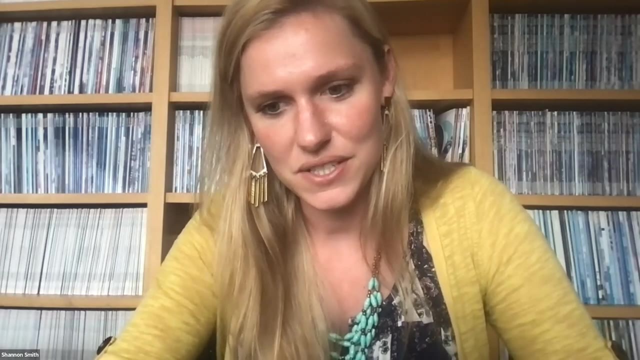 the application of ai. arguably, maybe it's one of the top ones, um, and that is the um. we call this pharmacokinetics, um in my world, basically what the body does to a drug, um, and looking at the safety of a drug in that context, in the efficacy um. i want to base this on the fact that 90 of drugs. 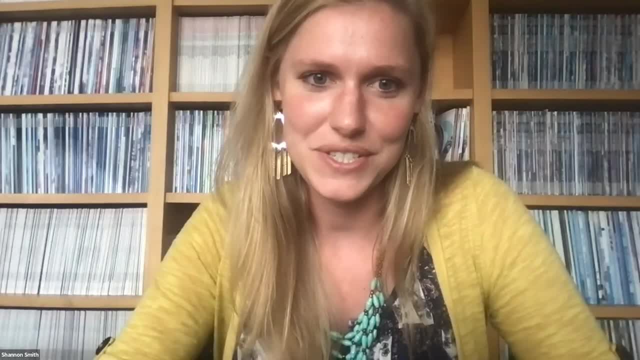 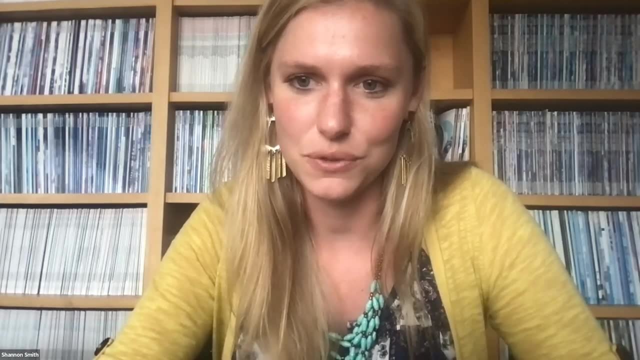 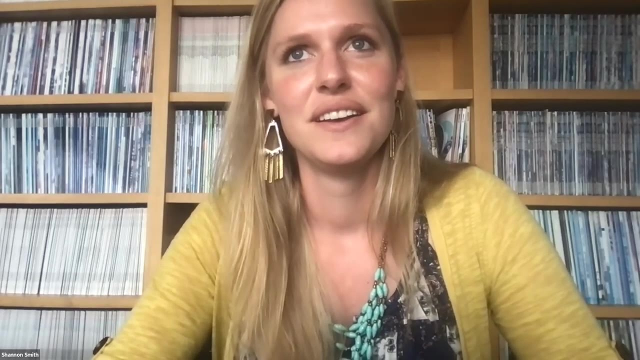 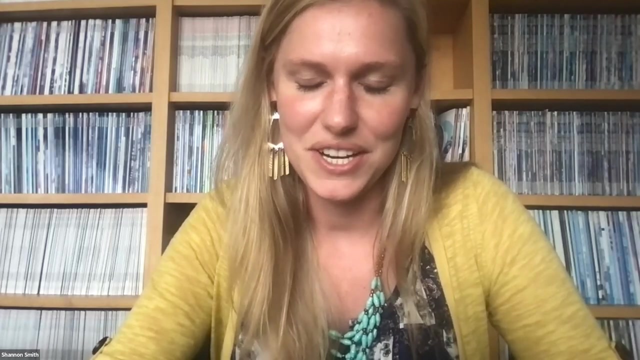 that get into human trials fail for one of these reasons. so this is a big place for potential. uh, with these tools, right, that we can improve using these tools. um, and how do i? i mean that would be fantastic if we could just say: all right, here's this compound, you know, here's um, here's our system, here's our. 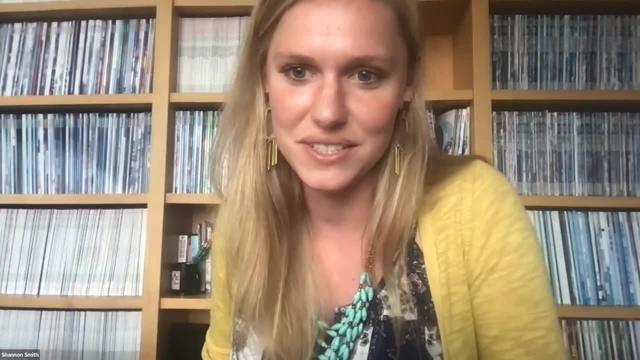 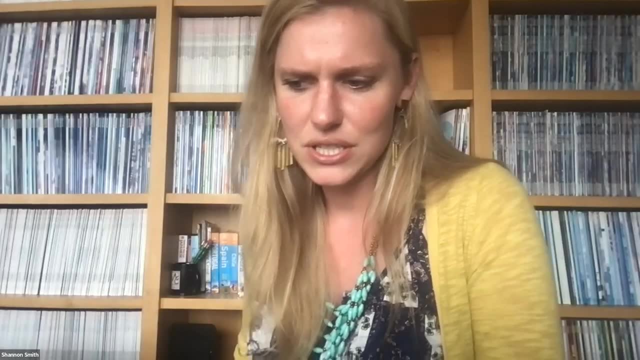 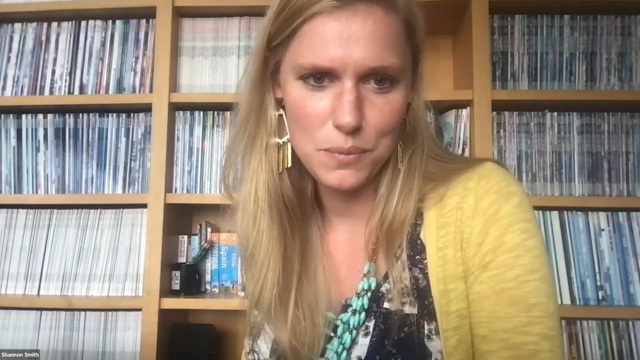 here's our person. maybe in the context of a personalized medicine, right, how would this uh, how would this react? i? i kind of mentioned it uh earlier, but i don't think that this works maybe in like kind of that end-to-end way. um, we can try to answer maybe more specific questions. 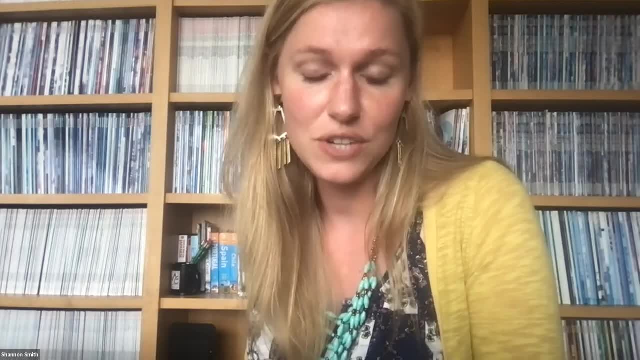 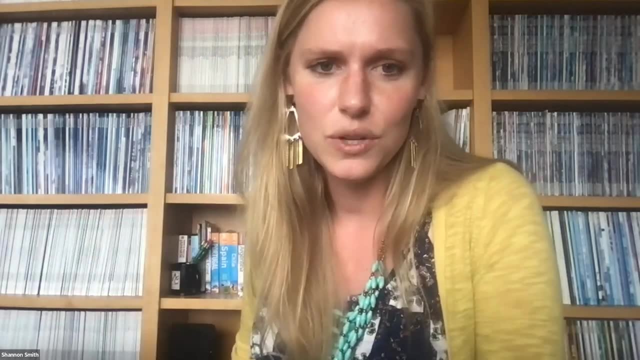 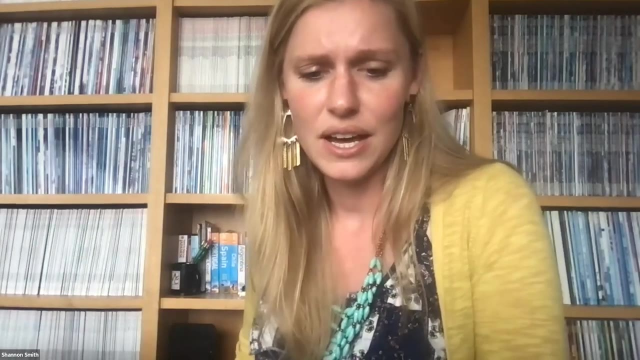 um, and for one thing, drug drug interactions are a really big thing. right, that would be one of the questions we could look at. here's this compound. would we have some uh potential liabilities with uh drug drug interactions- and this is a huge uh field? um, the way that people are doing this actually is using these tools and mining the literature. 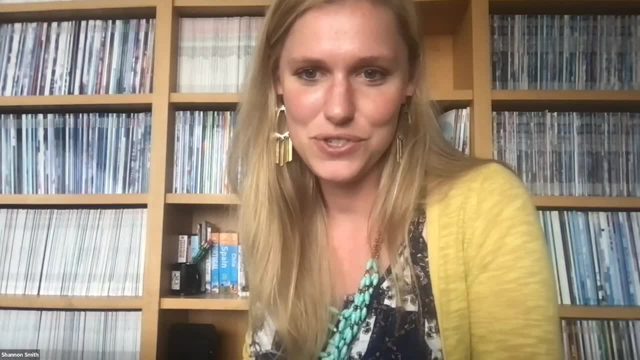 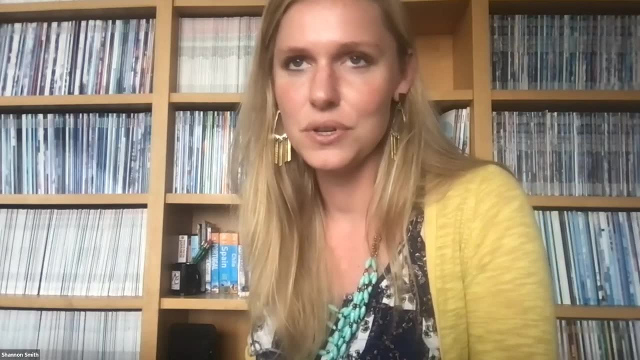 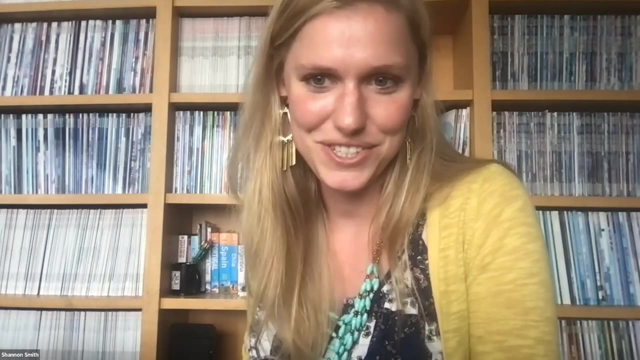 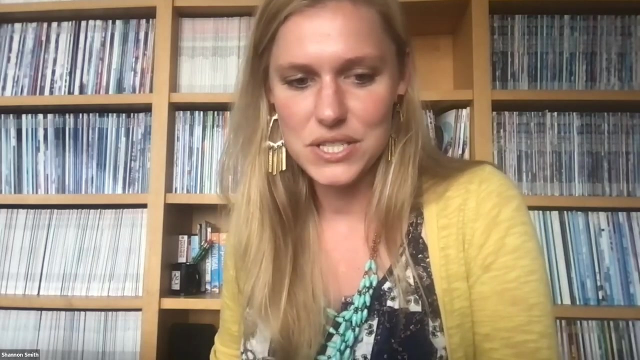 right, so it's actually not looking at- you know the chemistry in the context of the body, but it's actually using this and um and diving through, um, all of our available literature, whether that's publications or the patent literature or grant literature, right, um, and kind of looking at it, uh, that way, um, but it's a huge thing to be able to say: can we predict? 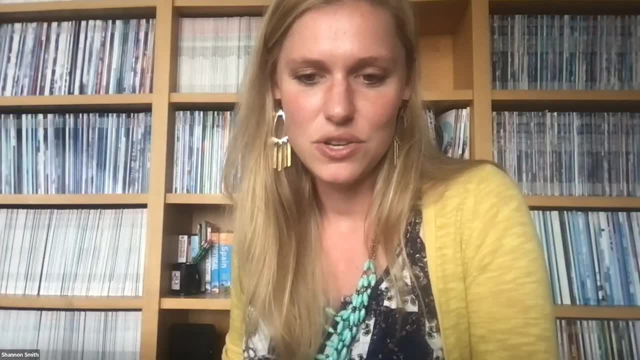 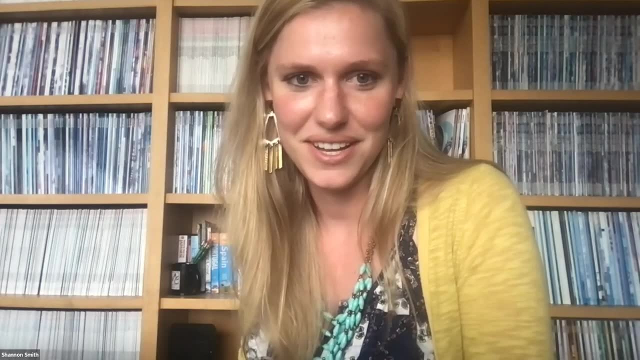 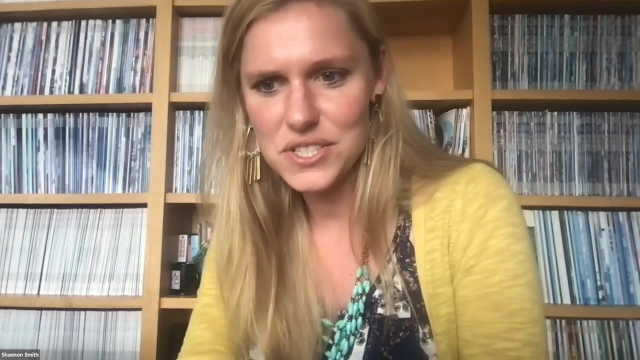 the potential safety of this molecule and you go and ask chemists and they have. you know, um, they have a lot of different ways that they think about that question and we don't really have an ai tool quite yet um to do this. um, can i also? i wanted to, uh, answer another question that was in here a little bit along. 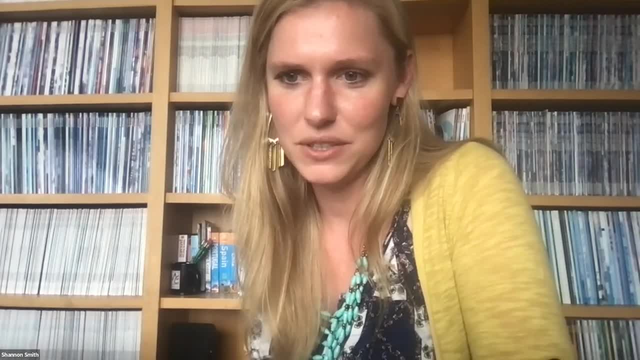 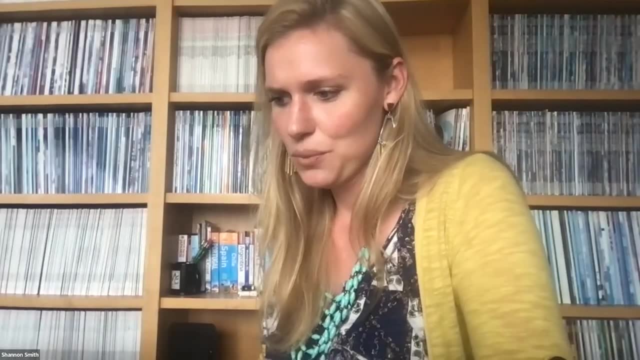 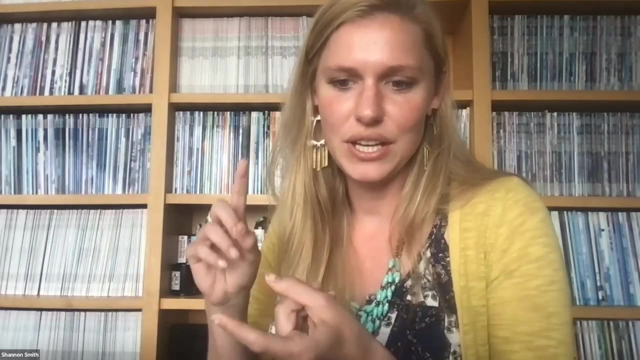 the lines: um. a couple questions further down about molecular imaging, yes and uh. kind of tack this on um, and so one of the things that you would you look at is: um, when you go into clinical trials, right, you're looking at, uh, you'll take blood samples, right, and look at the different. 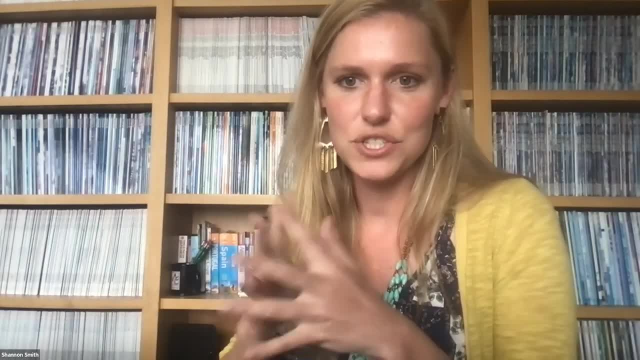 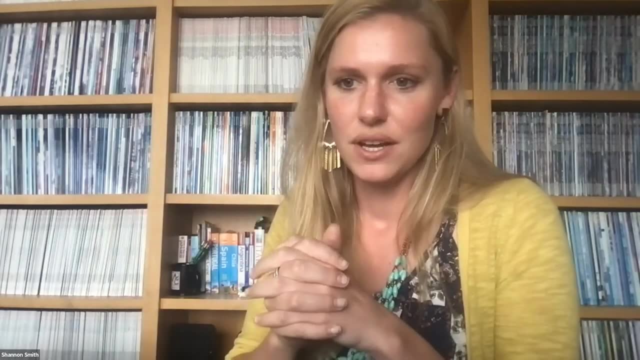 concentrations and you'll look at the different concentrations and you'll look at the different concentrations of, you know, different things within the blood, or do imaging studies, um- which is how i'm hooking into this question- or histology, whatever, if you do a biopsy or something um one of. 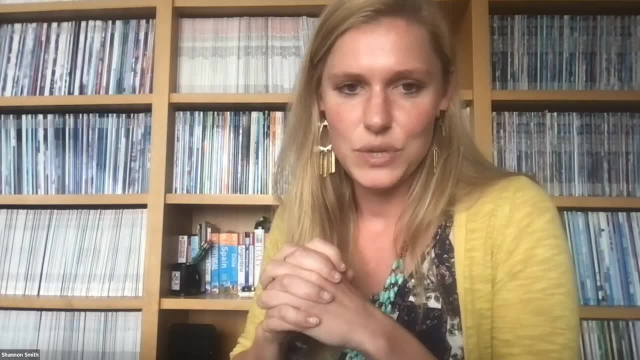 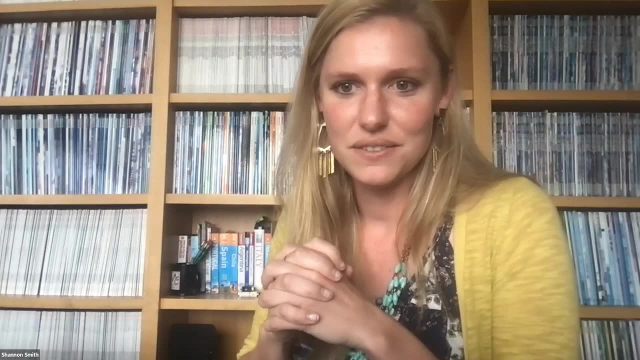 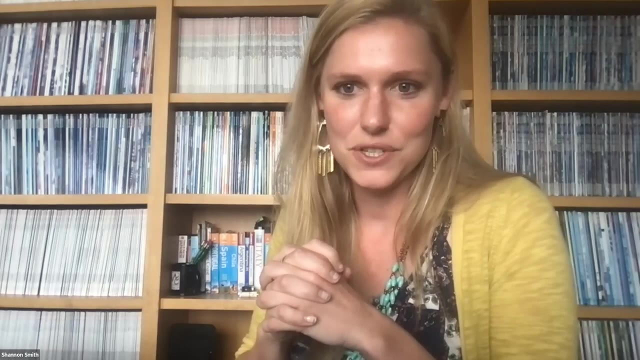 the advantages of ai in the past couple years- and we discussed this yesterday in our little, in our talk- is that you're able to incorporate a lot of different modes of data, right, you're not just restricted anymore to, um, you know, big matrices of numbers, right, images. you're able to incorporate a. 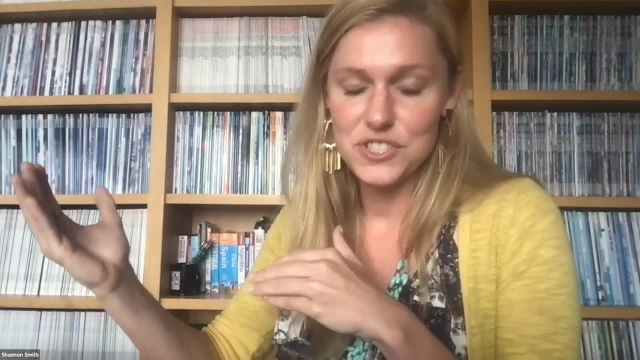 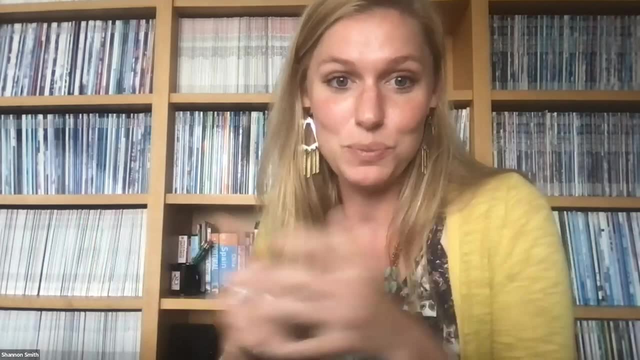 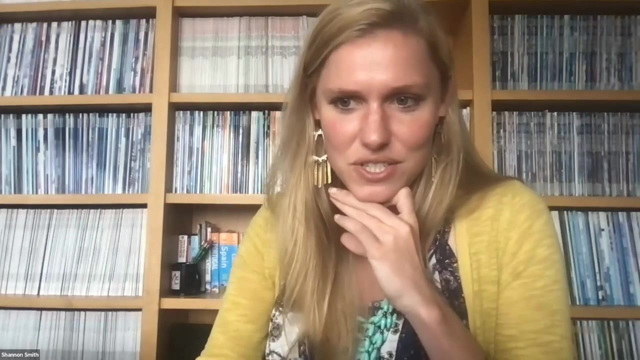 population of numbers. right images are being able to, you know, be our standard way to get these data. um, or looking into, uh, medical records would be a really great place to be able to do this. so i think maybe um josh him to answer your question here. i would think it would be really interesting to use. 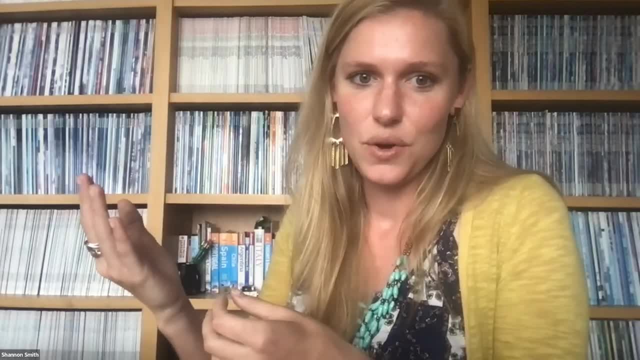 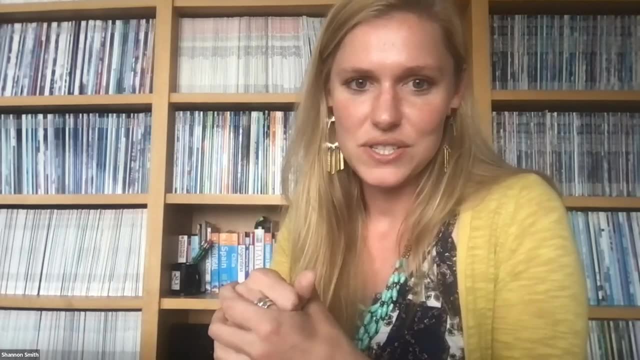 these tools to figure out what you're missing, maybe in the context of combining your imaging data with maybe some of these medically denied ones and then the other you know you have everywhere in medical records and the maybe what radiologists are, you know what they see, and kind of figuring. 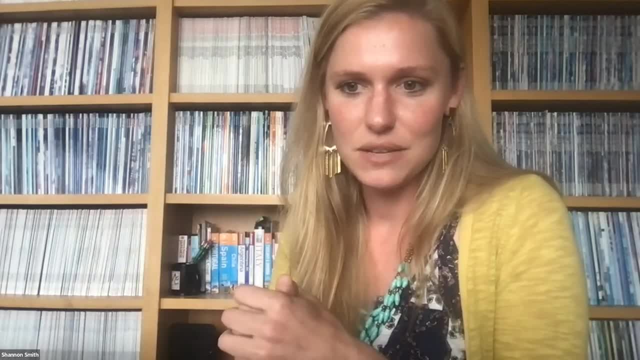 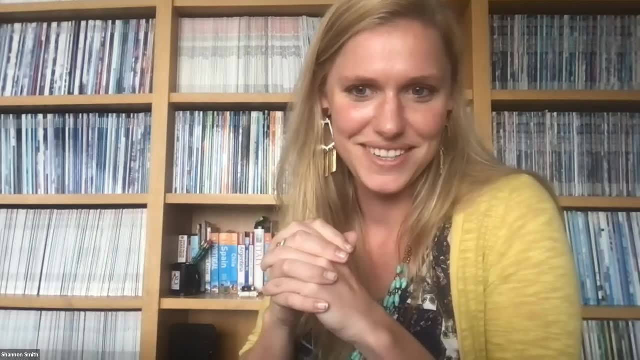 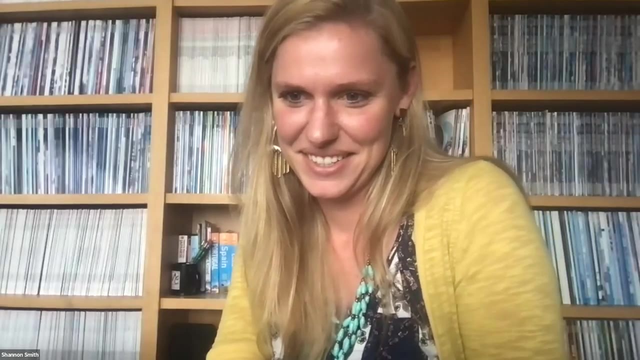 out, you know, combining those different data inputs. I think that would be. that'd be neat. I hope that answered your question. Actually, Shannon, there's one more question for you popped up. It's whether AI has already begun to decrease the cost of early stage drug development. 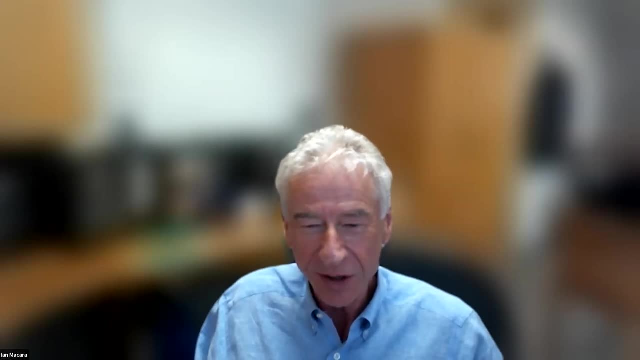 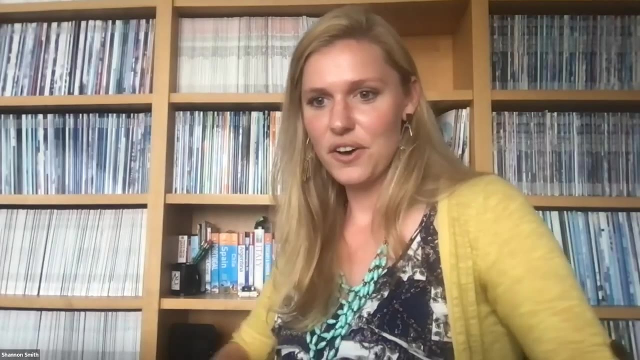 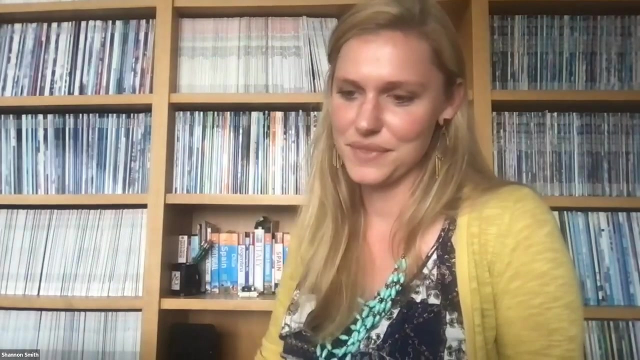 and you know, in general, are these, are drugs that are identified by these programs more effective? Yeah, a little early for this, but No, I think so. there's a couple of examples that that I'm going to, that I'm going to point you to where this has been used successfully. 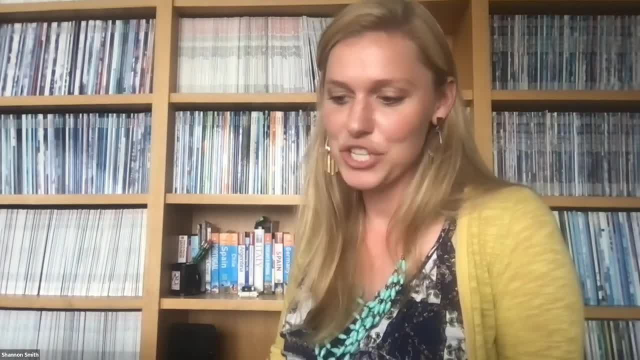 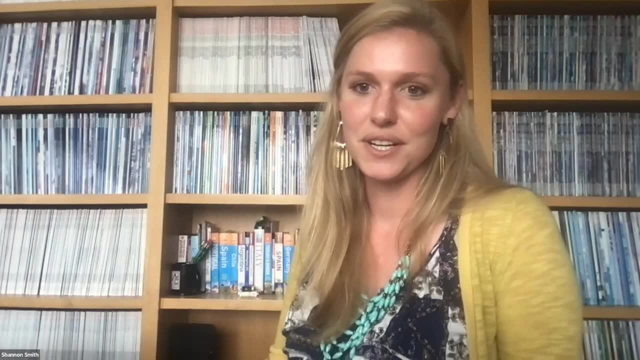 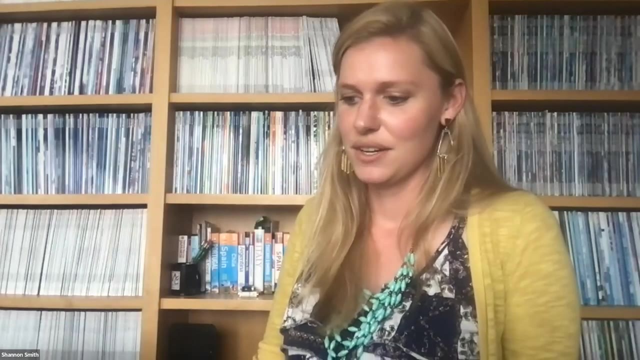 And so in 2020, Accenture developed a drug that is now in clinical trials for obsessive compulsive disorder, And that was kind of the first one that was deemed an AI drug that went to clinical trials, And so for that they had a. for those in the drug discovery world, they had a. 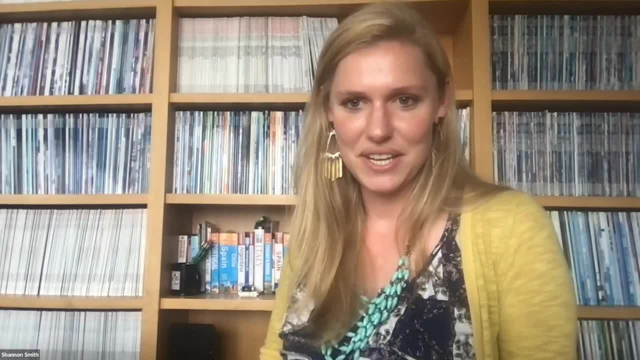 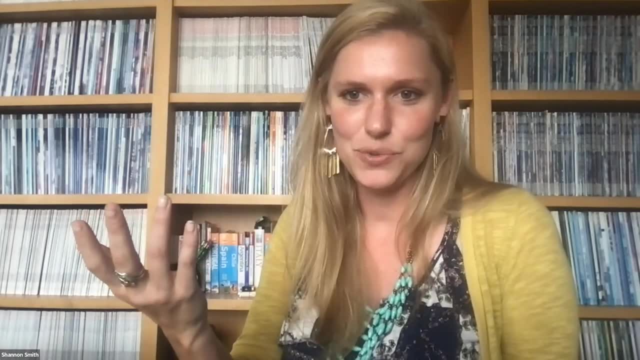 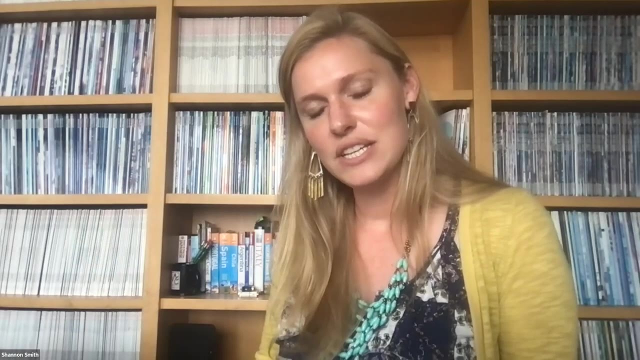 set target that had been validated towards this indication And it had it's a it's it's a GPCR right, Which we use a lot for CNS disorders right, And they were able to do a lot of the compound hit, discovery and subsequent optimization, which really cut down. on the time and also the cost and doing that process more efficiently to get it into clinical trials. So that was in 2020.. The second example that I'd point you towards is this company in particular, Nelco Medicine, that developed a fibrosis drug And what they did. that's different. 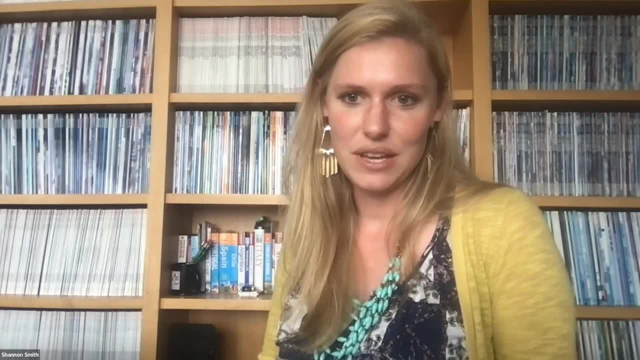 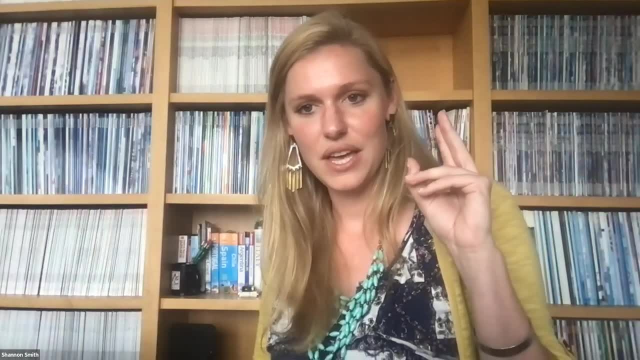 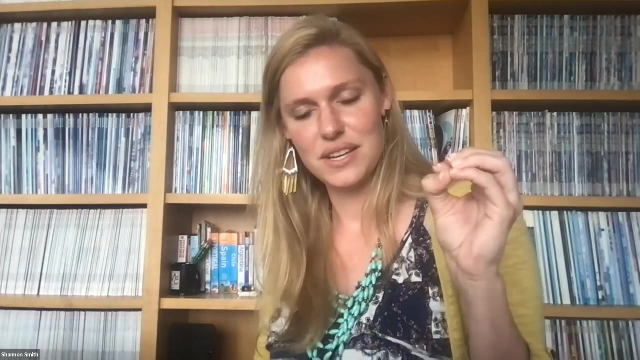 from the previous drug that I just mentioned is that they did not have a validated target when they were applying their AI to this, So they actually used it from start to finish. They they used AI methods to scan the genome and kind of these- the expression levels. 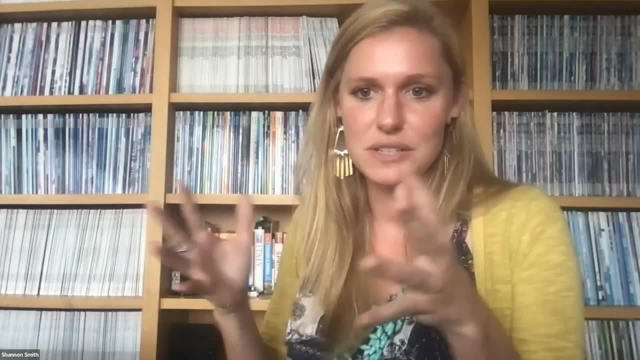 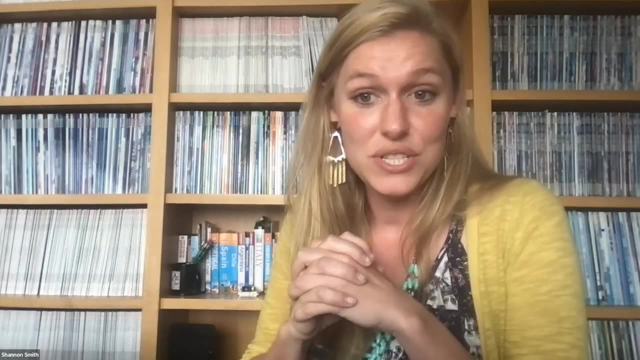 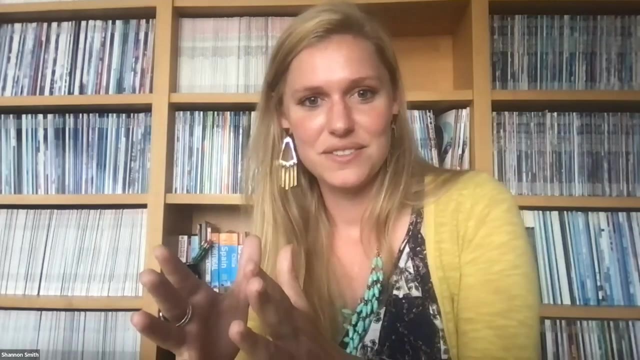 assume- I don't know for sure- of different proteins to figure out what's involved in this disease state and went in and identified a protein target and then validated it. also used AI to find a compound to target that protein, with the subsequent optimization. And now they're taking. 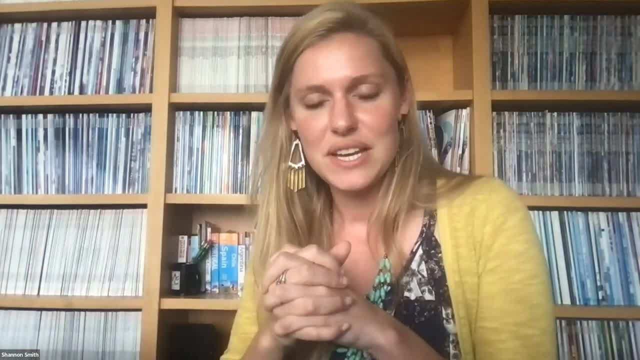 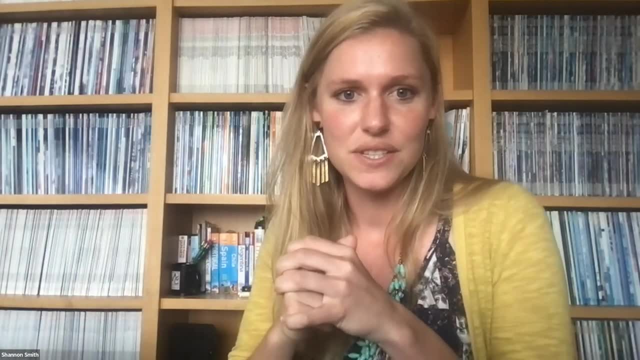 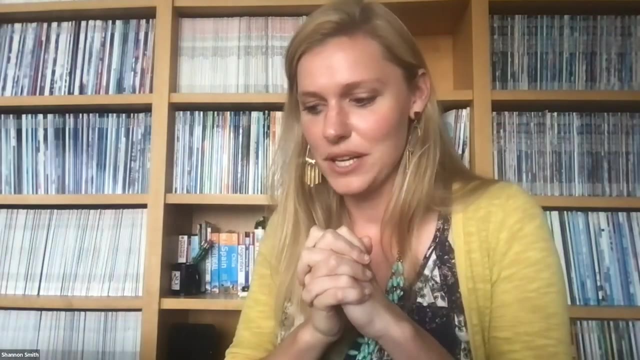 it into clinical trials, where they're also using these AI tools that I briefly mentioned, kind of combining data from as they follow these clinical trials and trying to figure out the effect when you put this into human. So they're really using it all along the pipeline, which is really cool. 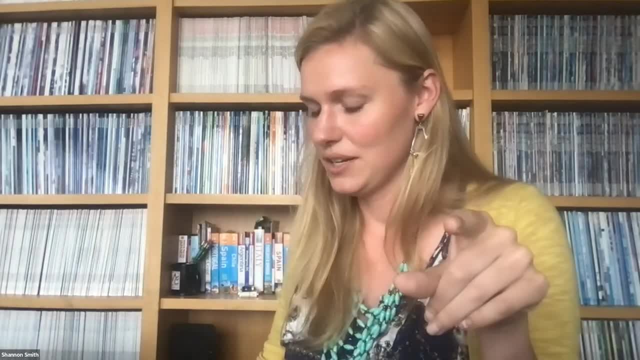 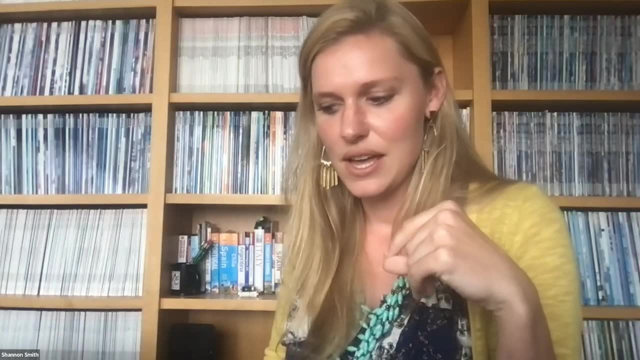 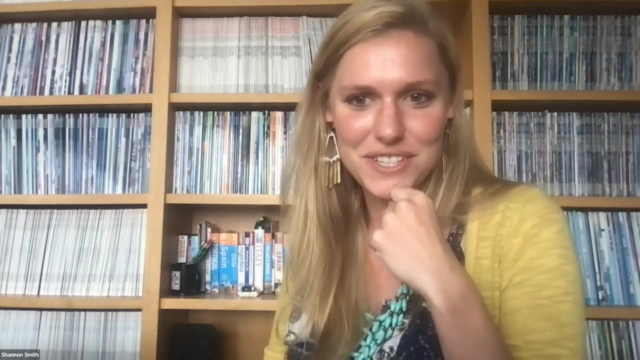 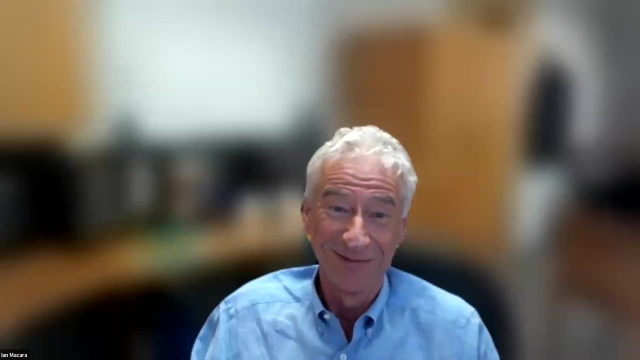 So to put a number to that, I've got a couple numbers jotted down here. This process to get it into clinical trial took 30 months and it was 2.6 million euros, which if you compare that to other drug discovery ventures, that is really fast and that's really cheap. I think this is a 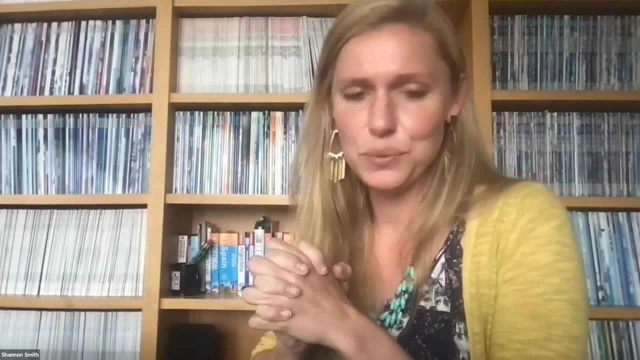 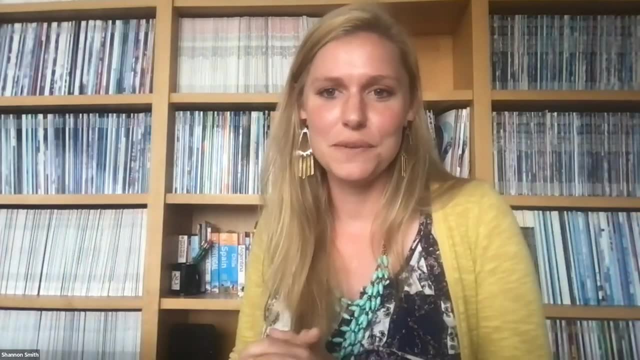 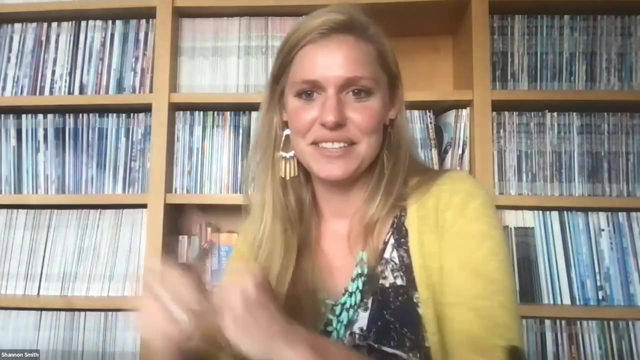 phase one currently, so we'll see what happens with it. but that's really cool. I mean, that's fantastic to go from a. we want something to treat fibrosis. let's figure out what's involved in that, let's make some compounds to bind to it and then let's navigate what it's doing in the. 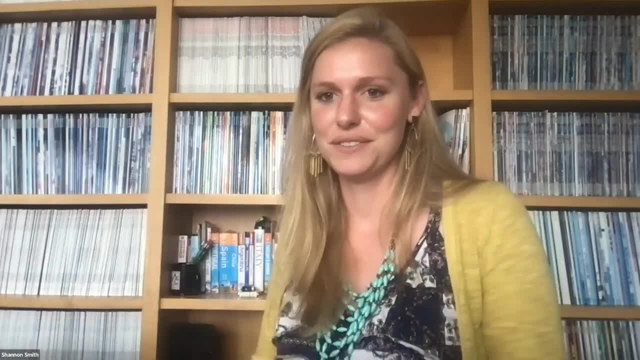 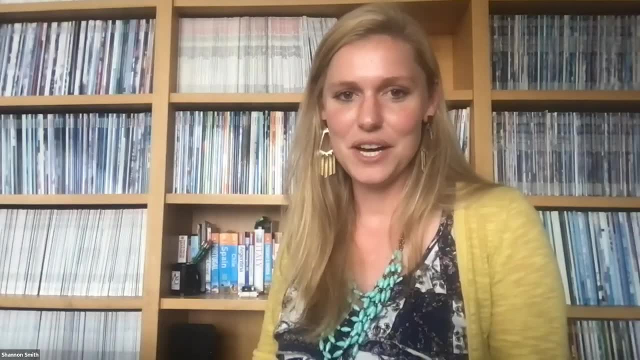 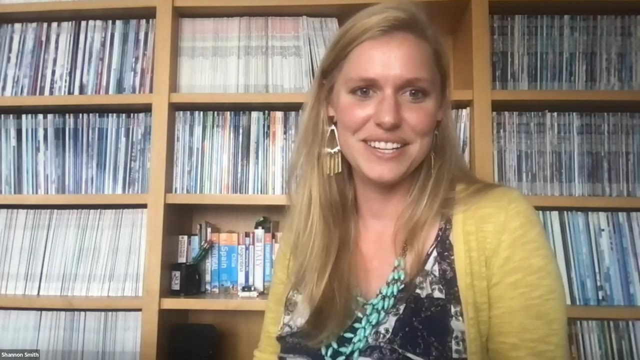 laboratory and using AI all along that pipeline. So it is starting to get there. I think we're kind of in this- I don't know kind of in the upswing of where this is really becoming a realistic. it's the hardware right And kind of the development of these AI tools really allows us to. 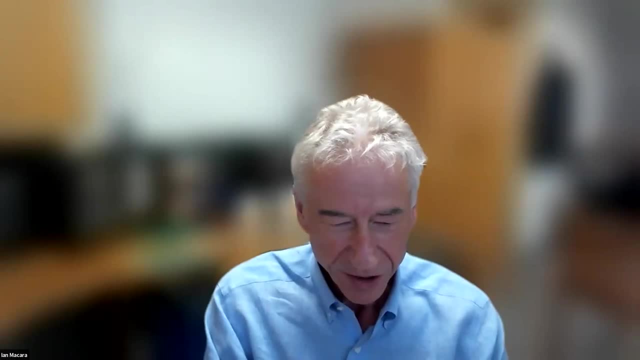 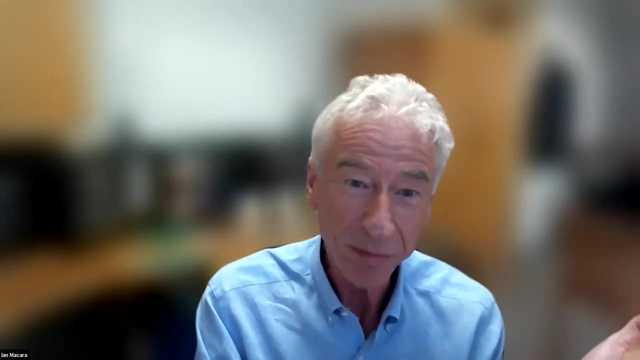 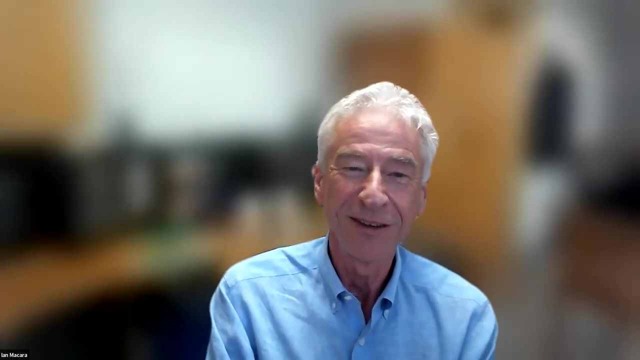 do this realistically in practice? It was a big article in Nature a few months ago where they could screen, you know, virtually they could screen billions of compounds against a particular target. I mean, you know that would be impossible to do experimentally. And then they, you know, they pick the best ones. 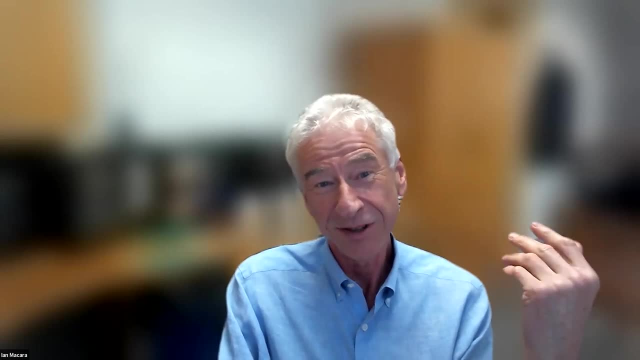 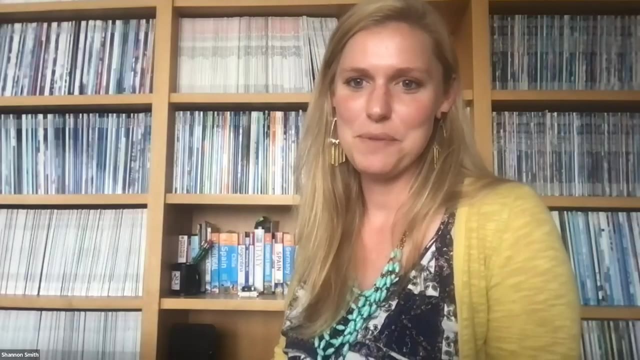 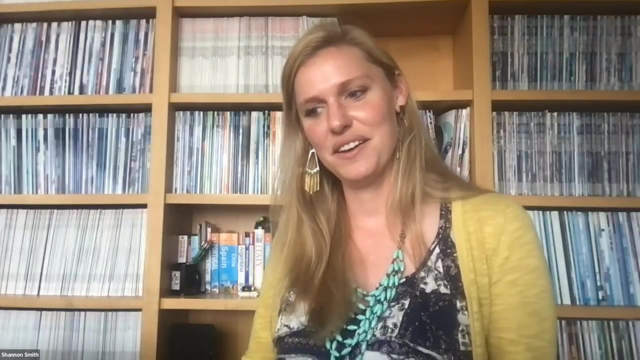 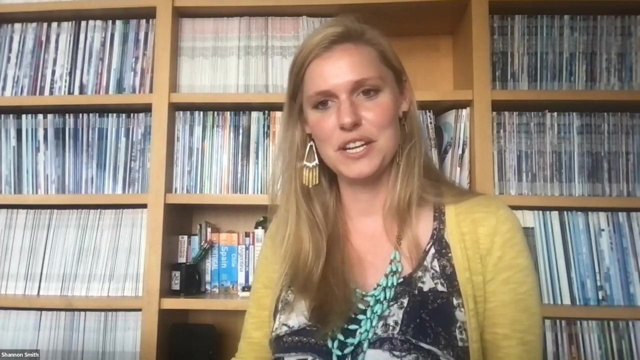 and sure enough, you know, I mean, when they do test them, the top hits, they work. It's pretty remarkable. Yeah, that's exactly what I do. That's my project. I virtually screen billions of compounds And then come out. we're able to obtain a hit, you know, from a small number of compounds tested. 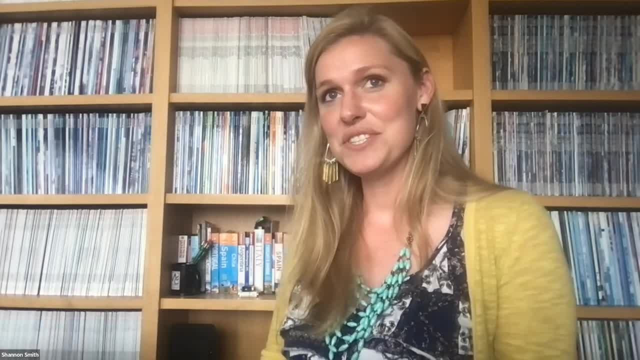 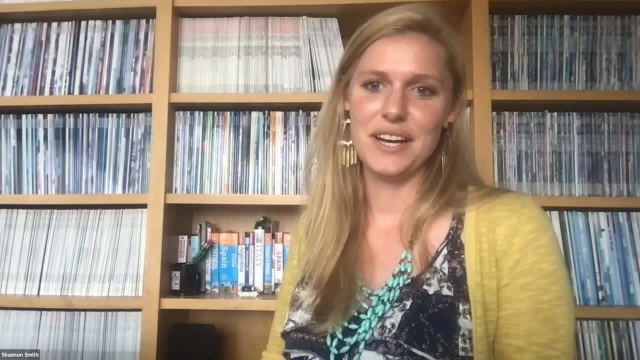 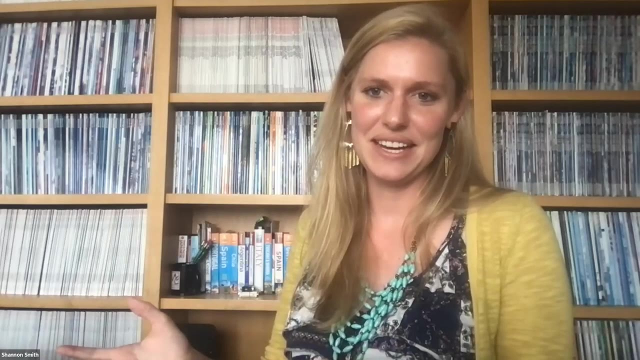 And you know this is kind of a. you know this is a really difficult thing to apply this to drug discovery because chemical space is just enormous. So how do you go about efficiently scanning that? And this is a big question. And I think it's a really important question And I think it's a really 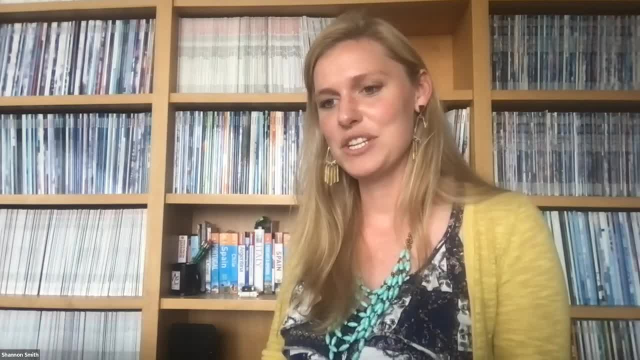 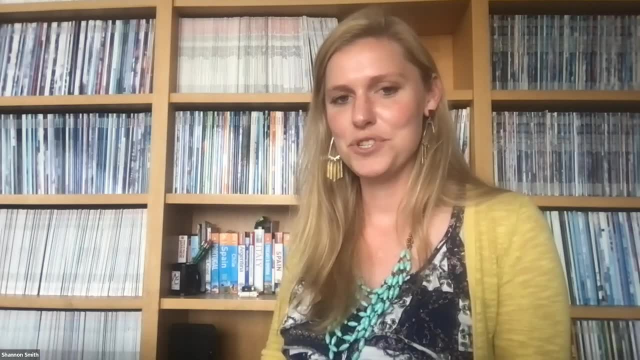 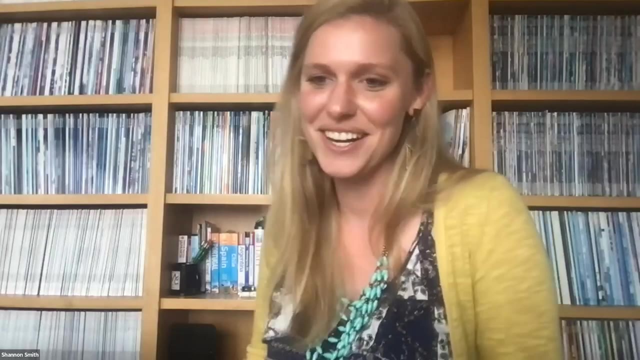 big, big question, And we mentioned AlphaFold earlier, that's, you know, DeepMind. I think that this is the problem they're trying to tackle next. Sure it is, And it's an important one. It's one that is. it's really hard just because it's such a diverse data. 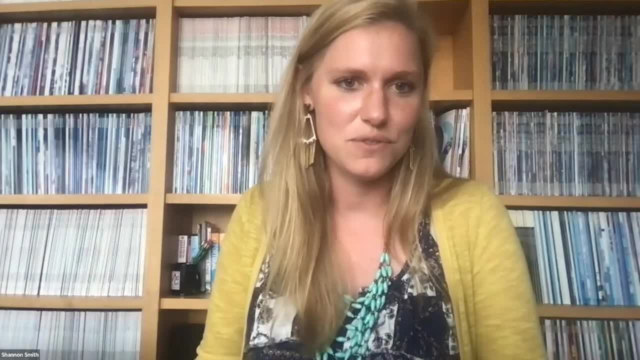 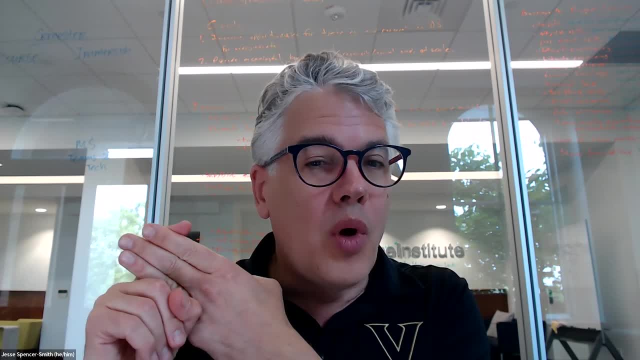 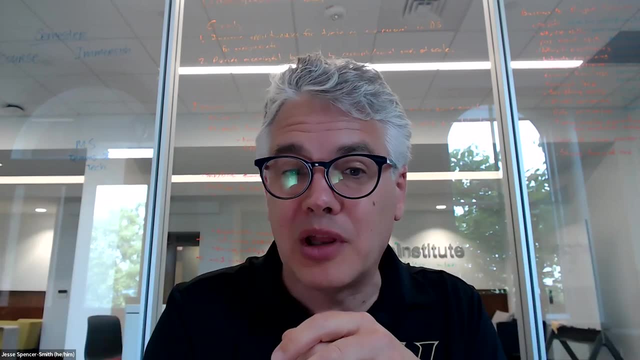 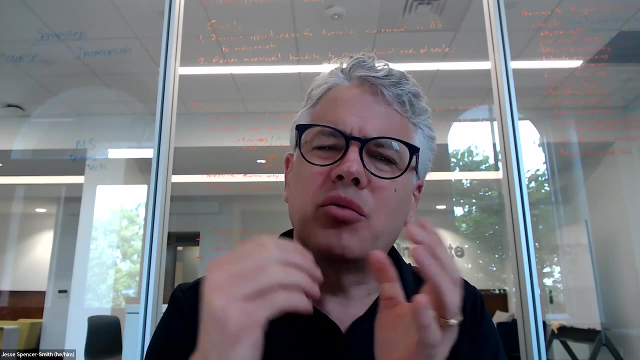 that we have. we need to be versioning our data and to know what we're actually training the models on to be sure that we do cover the full spectrum of the possibilities, including the edge cases. So that's a real ongoing problem. That also goes and speaks to the previous question. 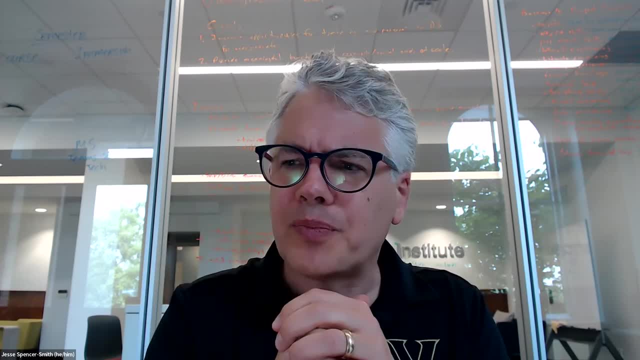 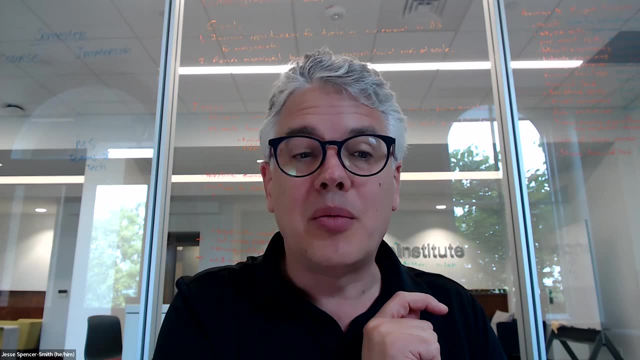 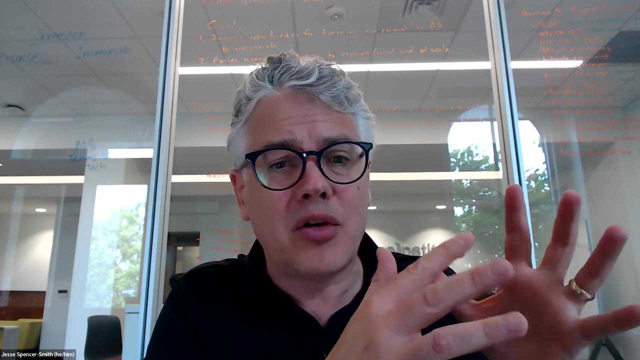 about explainability, especially in clinical settings. Often the answer is: did the model learn on a patient like this? And if you're able to say yes, here's the population that it learned on, then at least you answer whether it was exposed to those types of patients. because 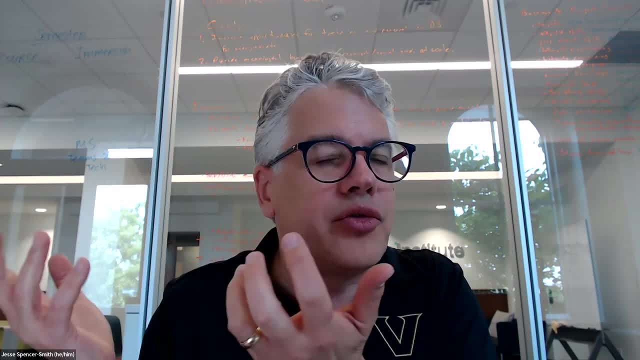 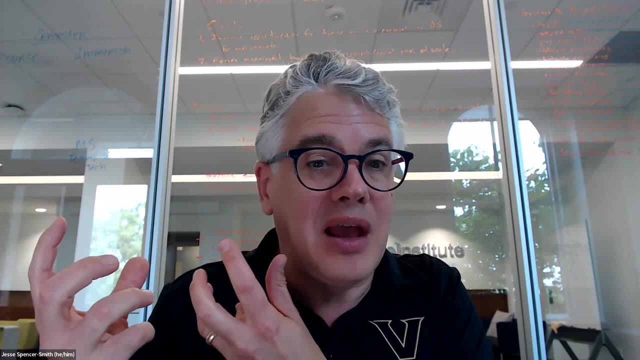 otherwise you could be well actually. no, we never saw, So there's no hope really of doing a good job. necessarily You might be able to impute or, for the model, make a good guess, but you can't count on it fully understanding what all the possibilities are. 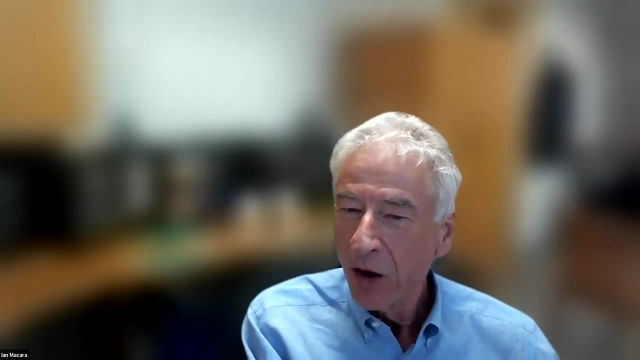 Ken Lauer had a question: Whether you're able to learn on a patient like this. What's the future role of academia in AI research, Because a lot of it's being done by large tech right Like Google and so on. Is that a problem? Will we eventually be at the mercy of? 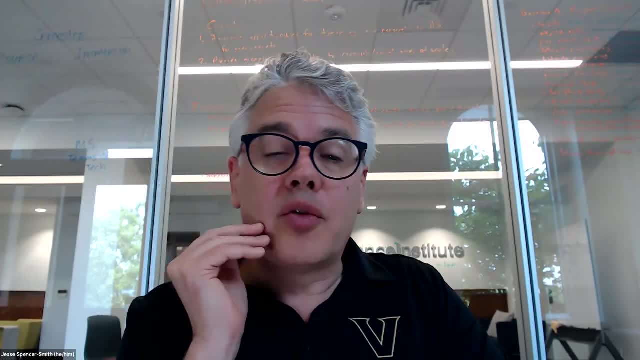 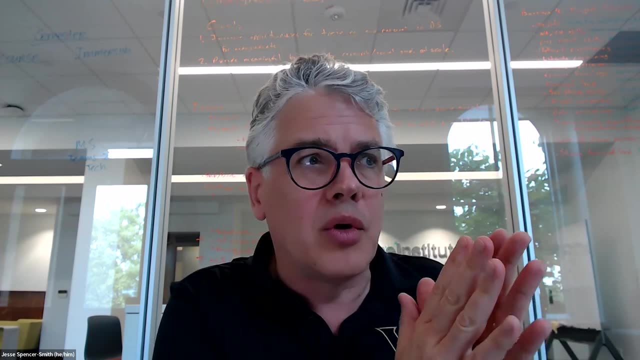 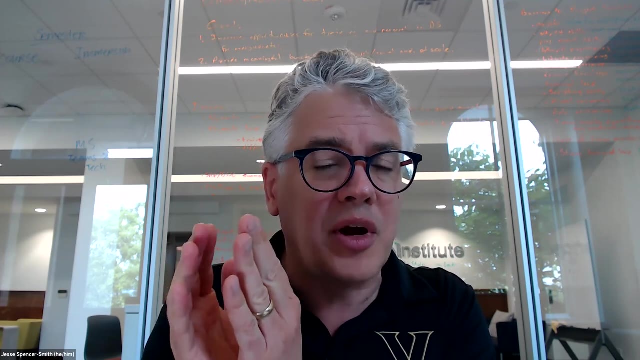 that. So there are a couple of issues here. First of all, we can use the tools that big tech creates. That's okay, It can move our research forward, But can we actually move the ball forward and solve problems that have not previously been solved by training up brand new networks? 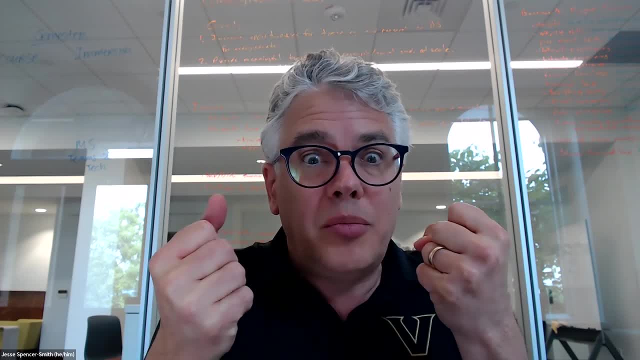 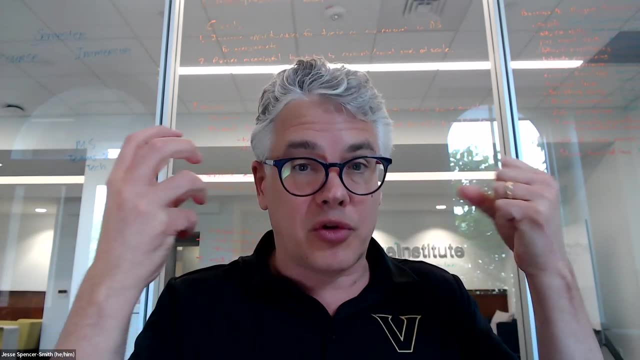 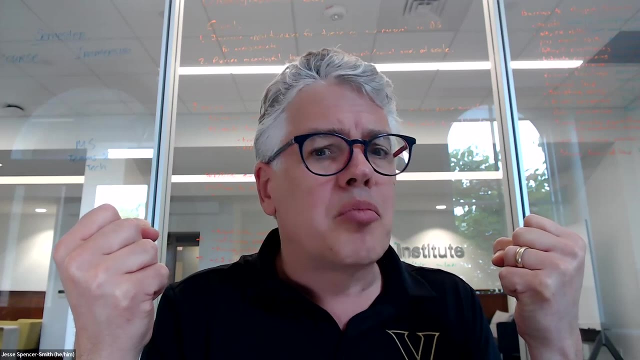 Actually we can. So the very, very large networks that can only be trained by large tech companies or by organizations like Big Science, which is training an open source, large language model. right now it's about- I believe, as of today it's about 60% trained, 60% there, But these smaller 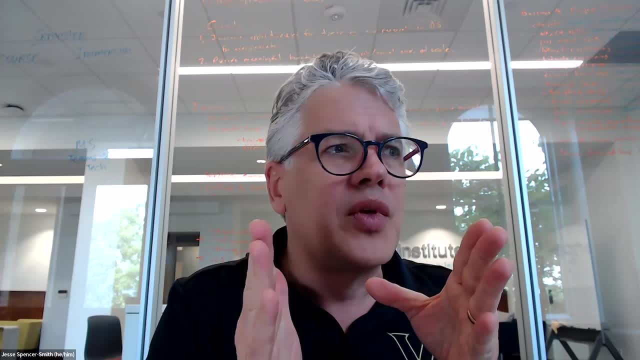 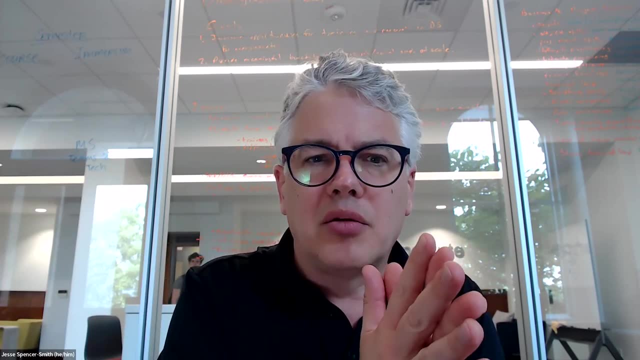 models. remember the transformers are general purpose, very powerful learners. So if you have a problem and you want to learn about a particular problem, you want to learn about a particular problem, you want to learn about a particular area- then you can train a model even from scratch, on this. 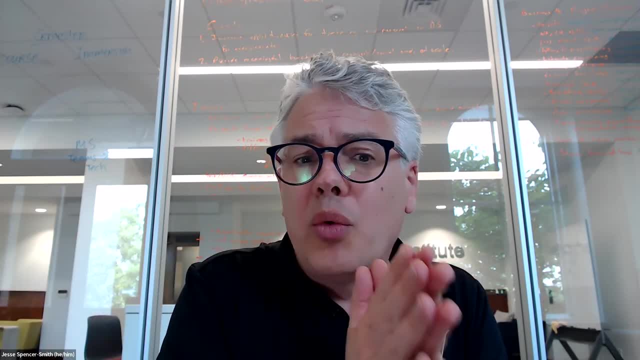 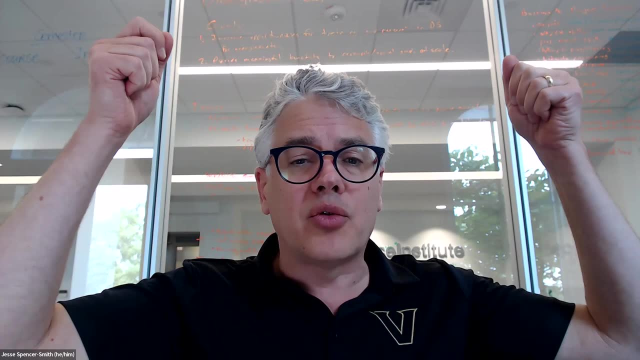 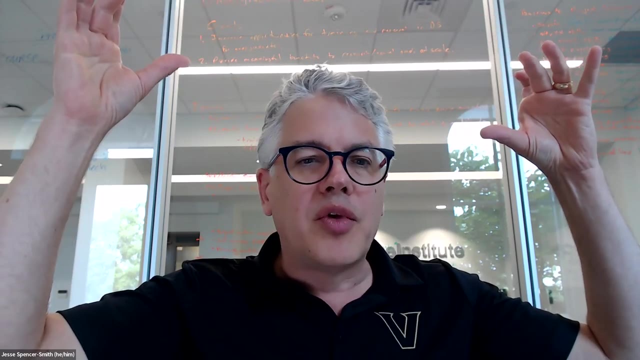 particular data, So that's always a possibility. This specialized model can very well outperform even a larger model. that's sort of a jack of all trades. So it's learned a little bit about your particular area because it's seen some. But actually, if you have enough data, 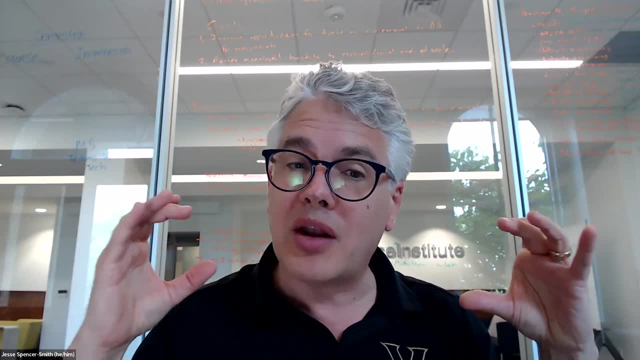 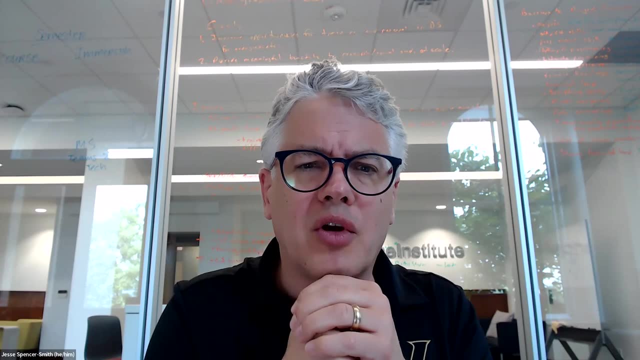 you can train a specialized model to solve your particular problem, And that is still absolutely something which a big tech company is not going to be taking on because they're not interested in your particular area of research. So, general purpose learners, we actually do offer workshops and trainings on how to do this, and 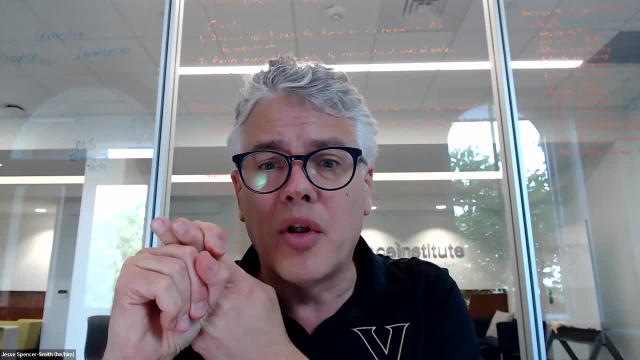 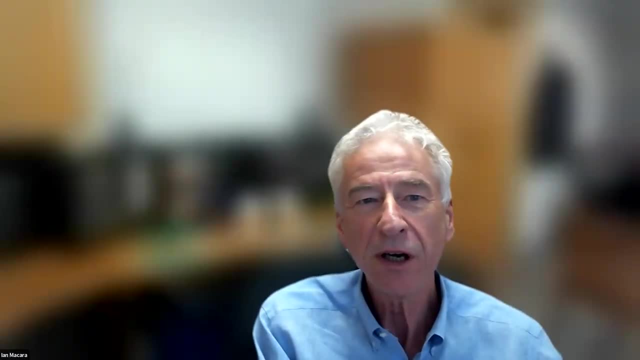 how to train models from scratch, And that's, I think, going to be a really important part of researchers' toolkits in the future. Yeah, absolutely Okay, we're almost done. That could bring up another possibility. There's also things: a new model for science. that's. 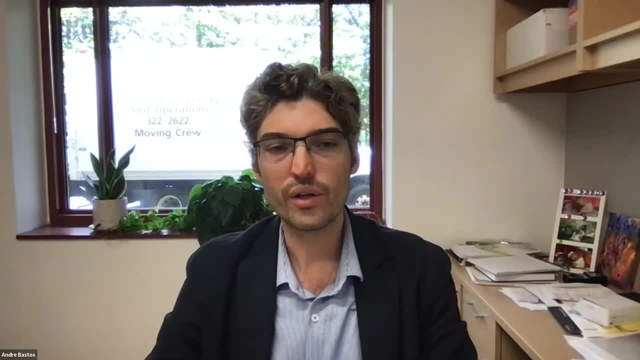 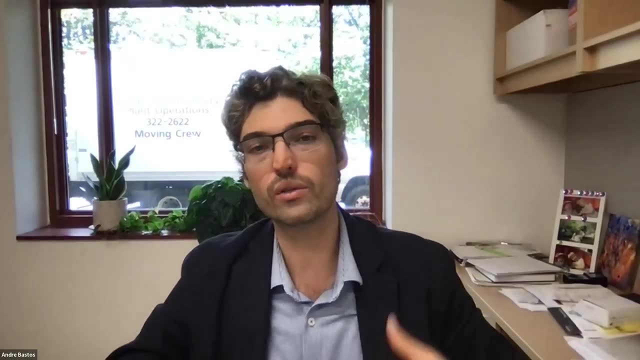 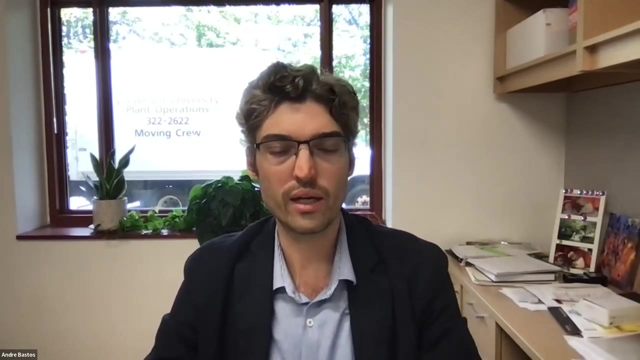 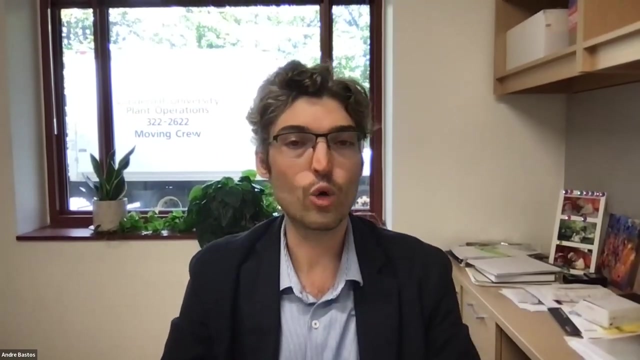 emerging in open science and open data, where you have certain institutes, like, for example, the Allen Institute, which occasionally puts forward their own massive resources in order to either collect particular data sets that they can partner with individual universities on and dedicate institute level resources for data collection through what they call the Open Scope.